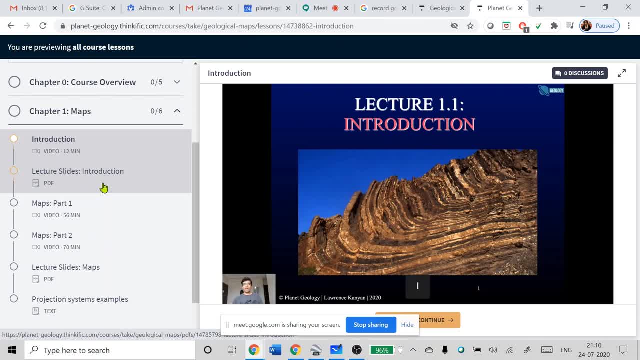 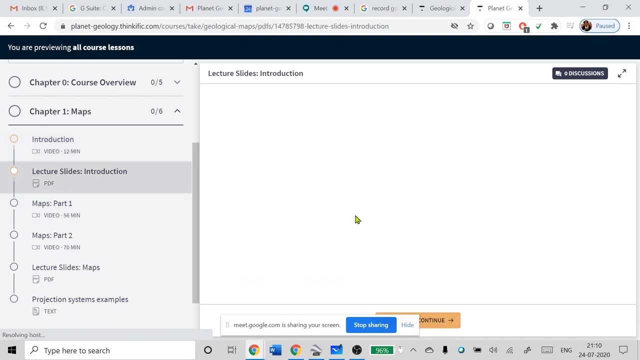 Sometimes they are asking questions based on projection systems. So these are very important for any competitive examination. So, and even like For a geologist, it is very important that you understand all this. So what are maps? what are different projection systems? those sort of things you will find in this part. 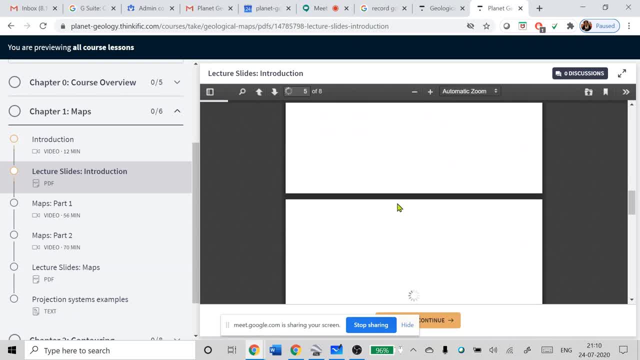 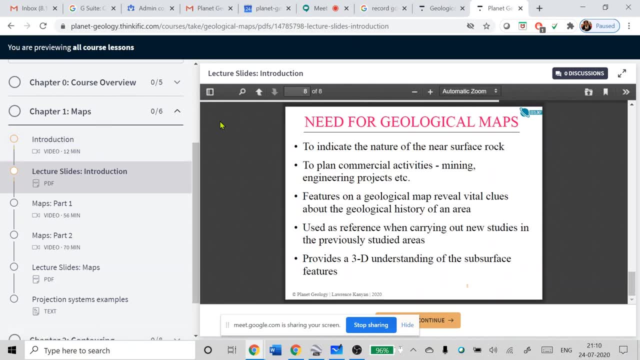 So, and I've also included the slides from this chapter So you can go through these slides and also go through the video lecture. So this will be very useful in. So this was, this was a, so I'm actually modifying it a little bit. 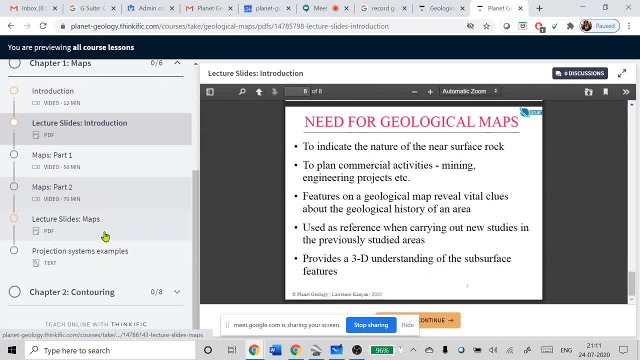 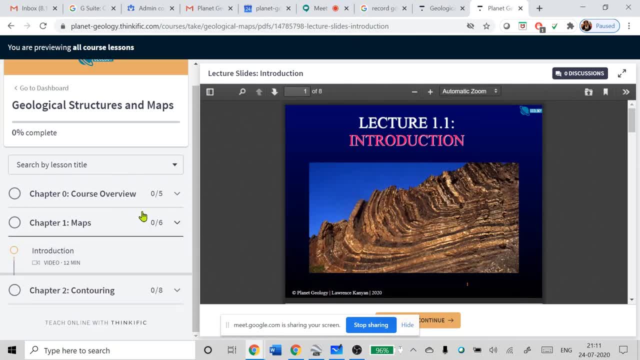 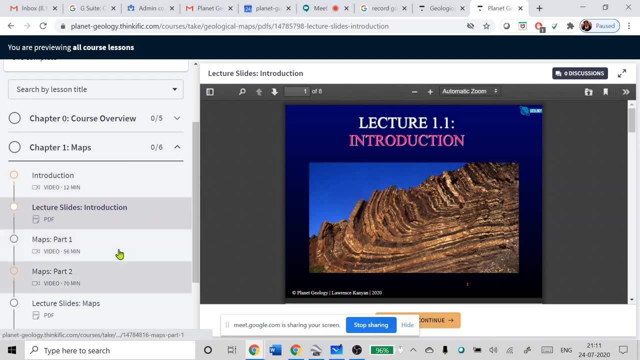 So the syllabus that you would have seen. so that is not the final one. So you will actually study much more than what was already shared in the In the syllabus. So after this second chapter is on contouring, So here in the first chapter you will also learn about toposheets, how they are numbered and 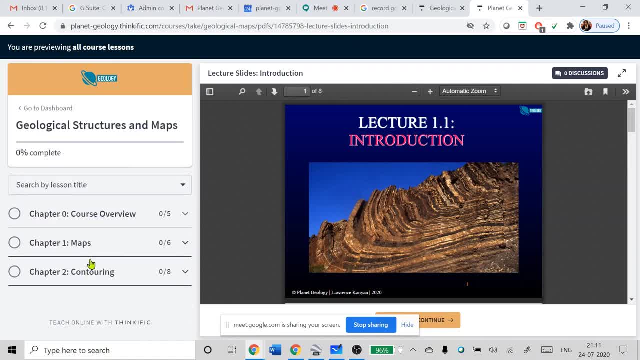 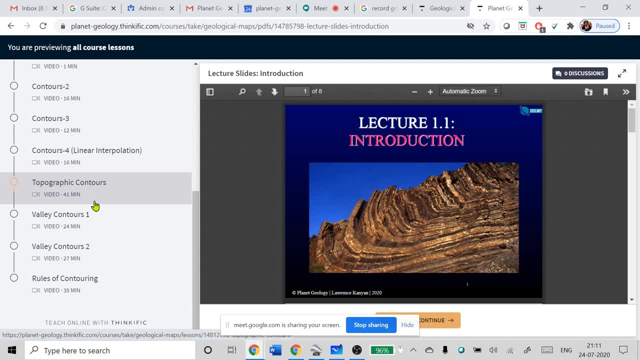 And about topographic maps. So here it's more. in the second chapter It's more about contour patterns of different geological features, such as valleys, hills, all those things that look after this. So this third chapter, next part, that we will study today, 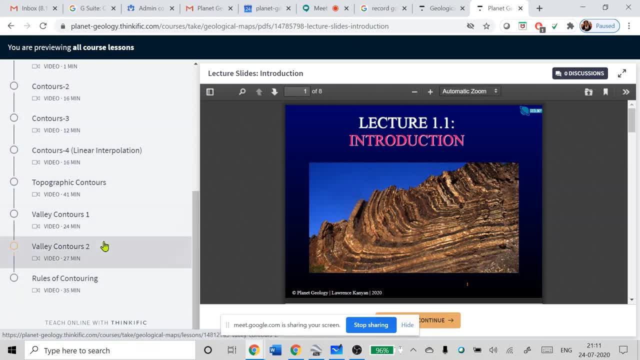 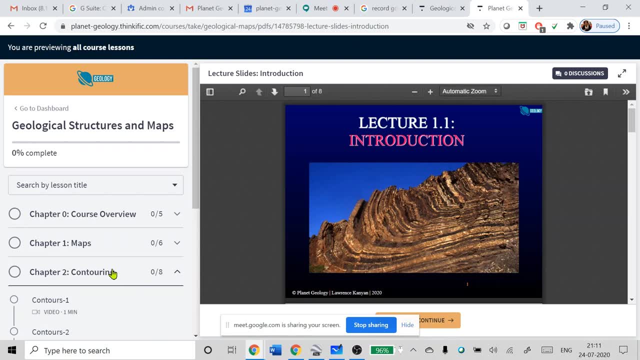 So I will encourage you that I know I'm assuming, Like you know these basics of contouring and also we'll study slightly a new topic today. It's not new, so we'll try to study it in actually a different manner So that you understand and you never forget how to solve these types of questions after. 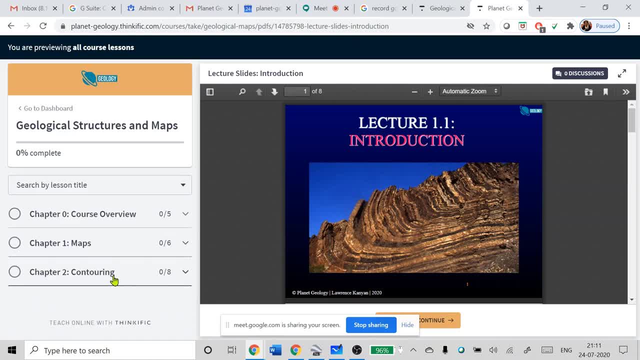 So you, I encourage you to go through these and I will also include quizzes within these chapters. So first you are encouraged to go through these and then attempt those quizzes. So the quizzes have not been uploaded yet, so they will be uploaded So you can go through those quizzes. So those will be uploaded. 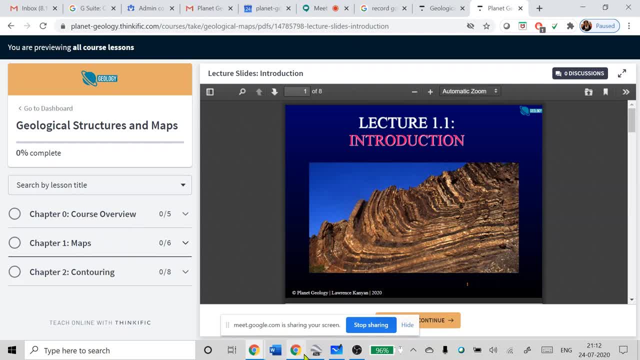 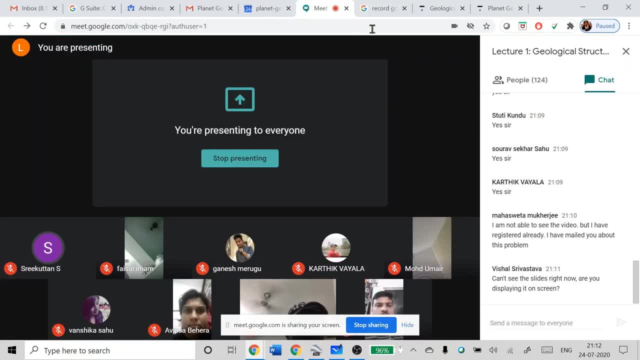 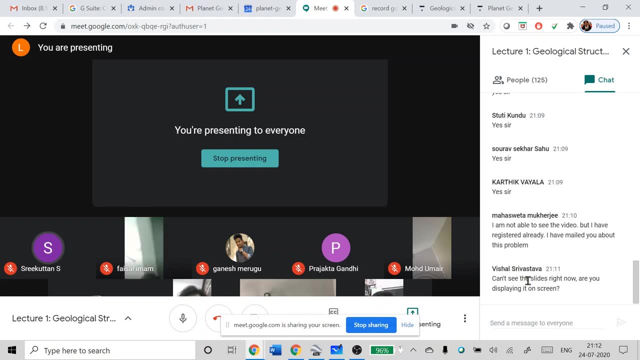 later on now, after this. so if you understand what contouring is, i will assume. so let's see, i'm not. so i i'm not displaying the slides yet, but can you see my screen? so some people are saying like they cannot see the slides, so i'm not, uh, presenting the slides as of now so you can say if, if, if the 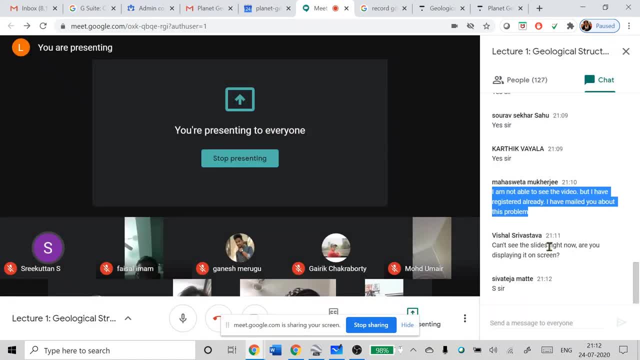 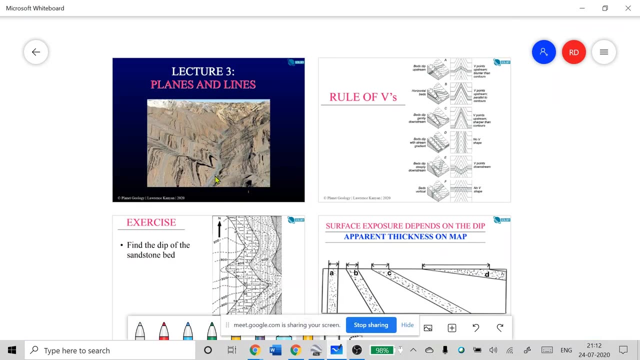 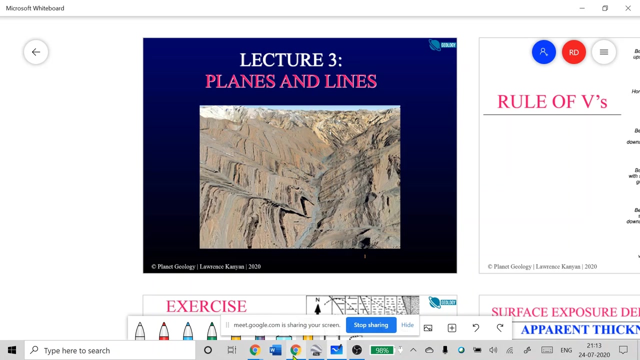 i've shared my screen. actually, if it is visible, okay. okay. if there's okay, then good. if that's visible, start with this one. so now can you see the slides. yes, sir, yes, okay, all right, so. yeah, so now it's better, when i ask some question, you can actually speak up, so that 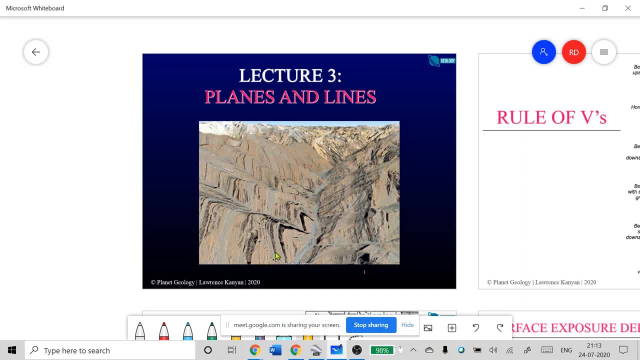 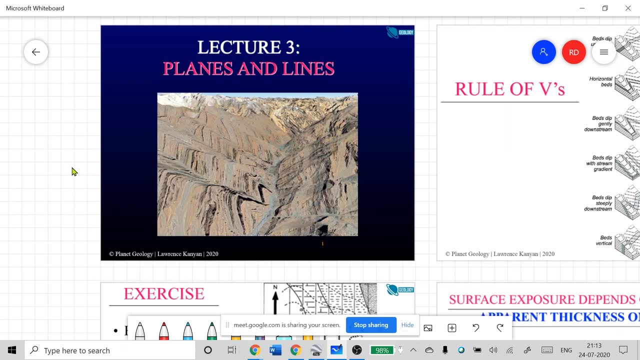 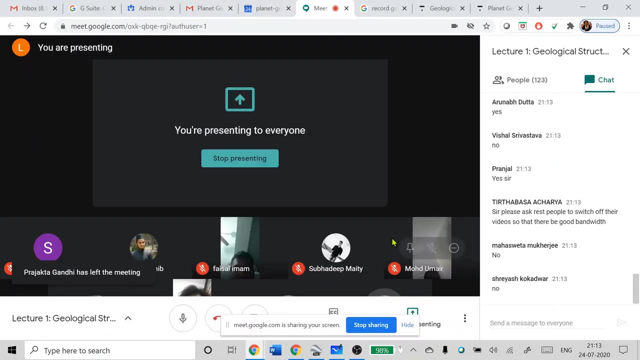 i don't have to look at the chat every time, so it's easier for me also. so, uh, in this part we will actually learn about uh, planes and lines you would have already gone through. yes, sorry, you cannot see the slides, uh, but i've shared with everyone. i think all of the slides are visible. 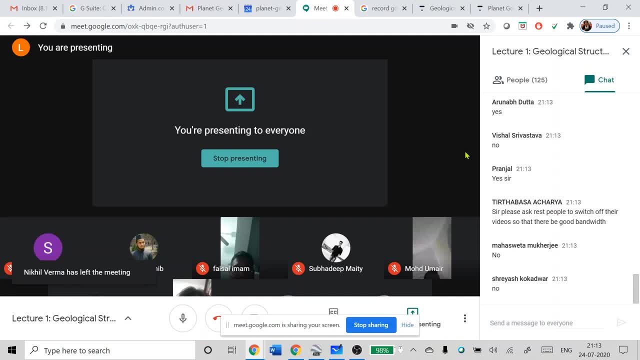 of them. can you please? either you can disconnect and try to connect again, and or else you can do is maybe check your internet connection, but I don't think what you will be able to do with that. and yeah, another thing, like someone has made a good suggestion, what you can do is you can actually other people you can 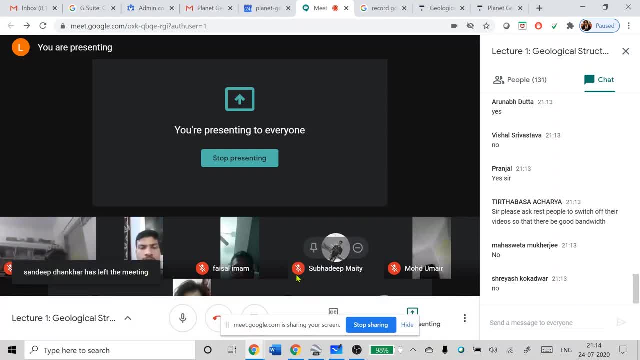 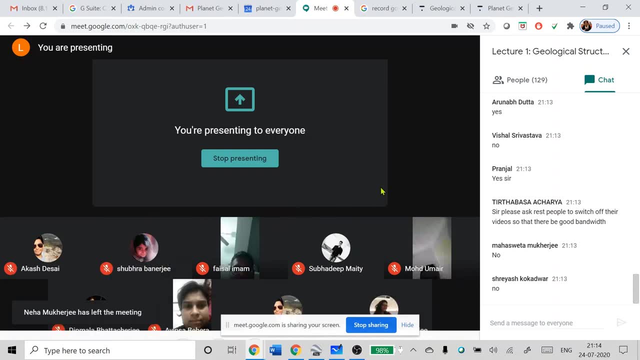 actually turn off your camera so that bandwidth is saved and there is less lag in the videos. so you can actually turn off your webcam. if you have to ask a question or something, then you can turn on your microphone and webcam, then you can ask. so that's that. I think that will be better. 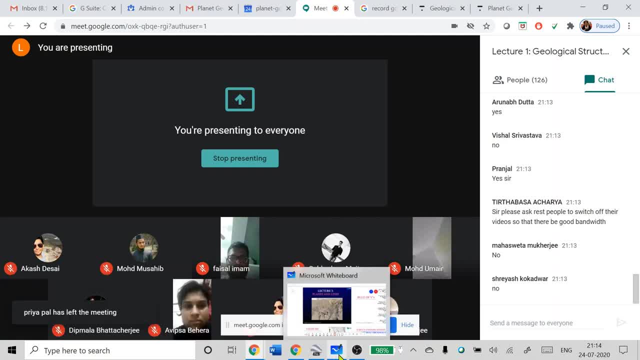 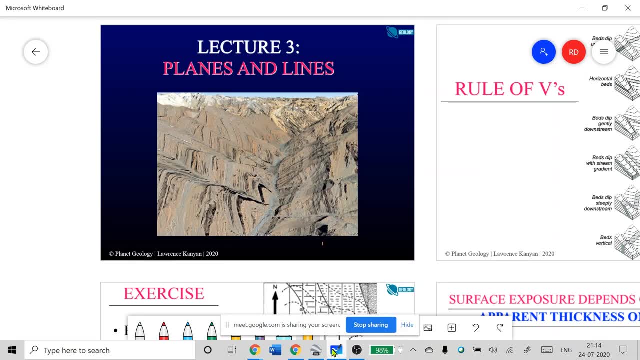 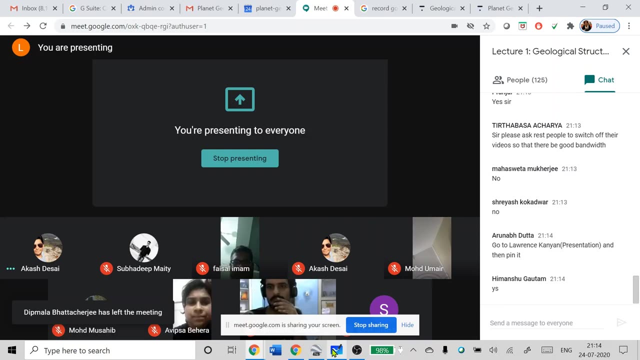 okay, so can you see? can you see the slides now, if okay? so if you are not able to see, maybe try to disconnect and connect again, because it could be problem with bandwidth or internet connection, but otherwise it's it's name. so actually I don't yeah. so no, I actually want to use this whiteboard, so 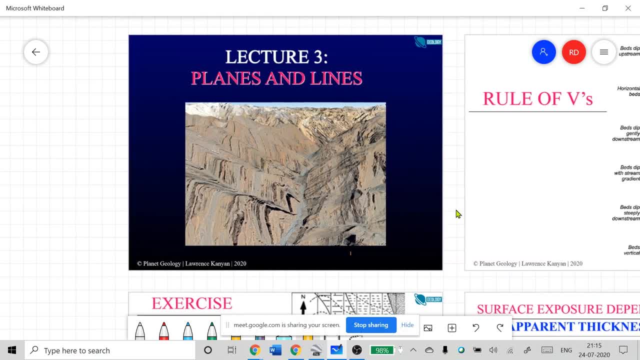 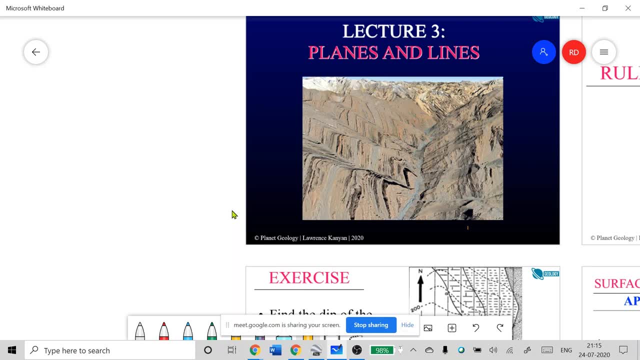 that I can annotate these slides. yeah, so now you can see. so in this part we will learn line of plane. so if you have gone through, so this contour pattern of valleys, hills, spurs or overhangs, etc. you will already if you go through the previous lectures. 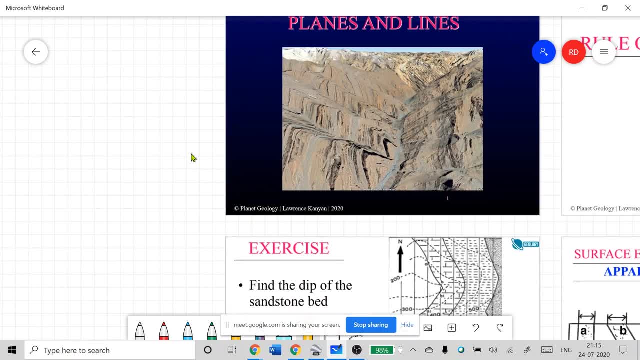 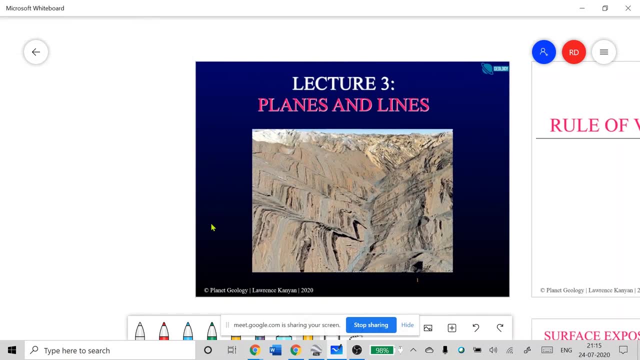 which i have already uploaded. you will know about them now. in this part we will specifically learn about the surface expression of in a valley. if you have these dipping beds- planar dipping beds- so we are not considering any faults or folds at the moment, so we only have planar dipping beds. 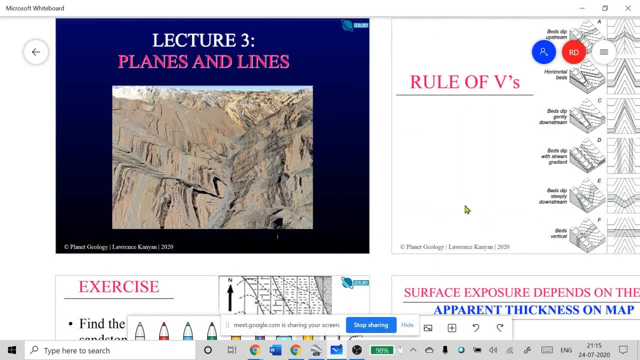 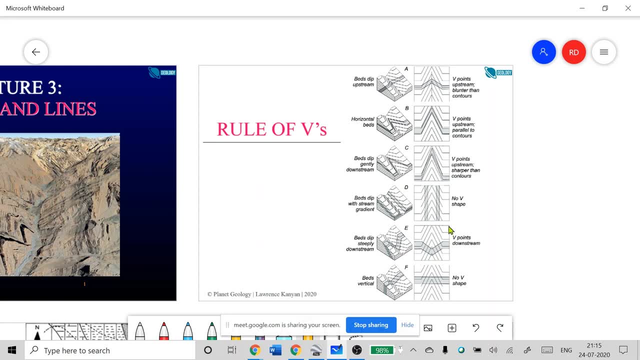 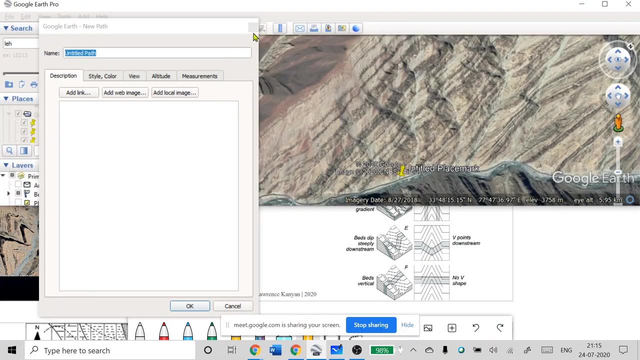 so how will the surface expression look like? so many of you would have already seen this type of figure. for some of you, it can be slightly difficult to remember, so we will try to try to make it easier to remember. but first i would like to show you some real life example. 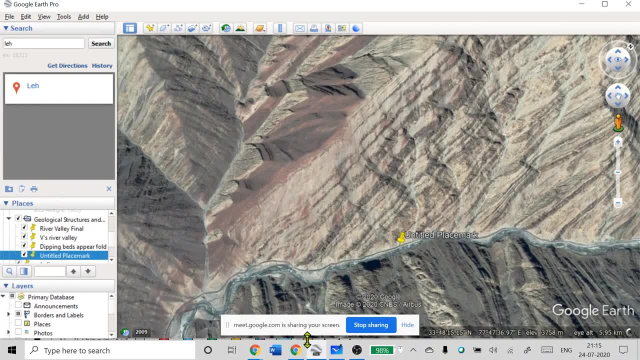 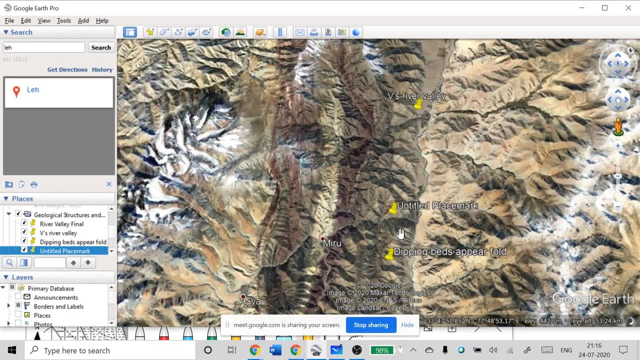 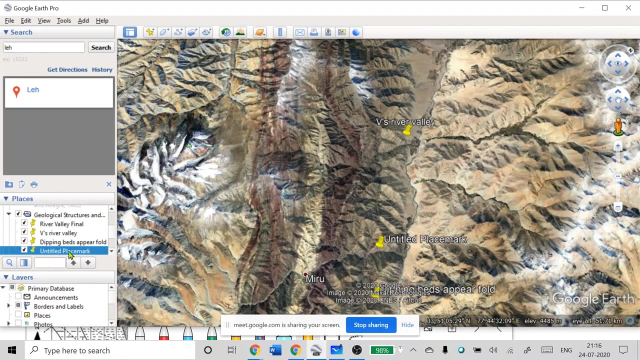 of this thing where you can actually see this. so now i think, can everyone see this? uh, so this is a google, so this is the Google Earth view, so we can actually view it in 3D. so I will also share this location placemask with you so that you can import them and 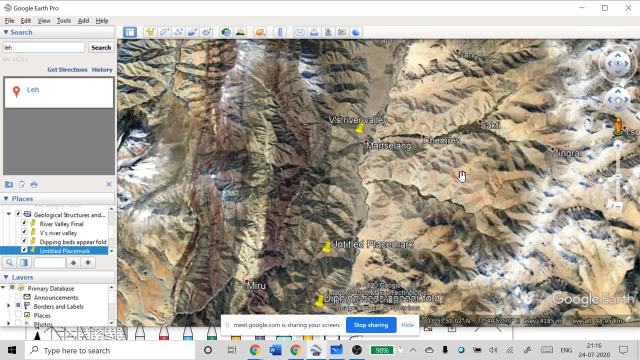 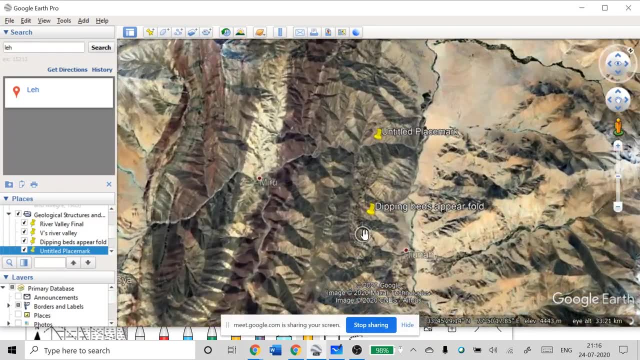 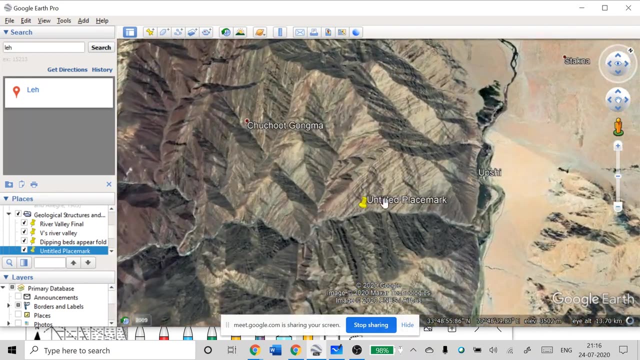 visualize for yourself. so this area is actually, we are very near to Leh. so this is Leh right here. so we are pretty close to that. and, yeah, this one. so this is the highway that you take from if you are going from Manali to Leh. so this is the. 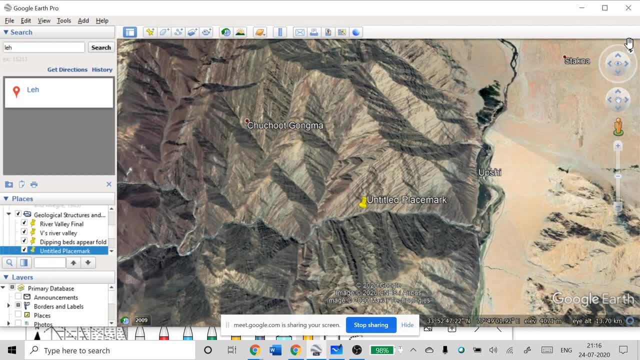 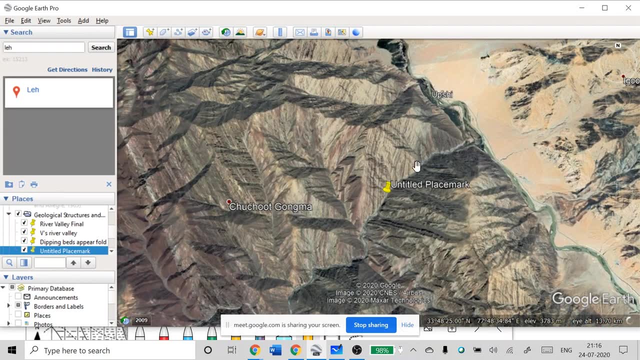 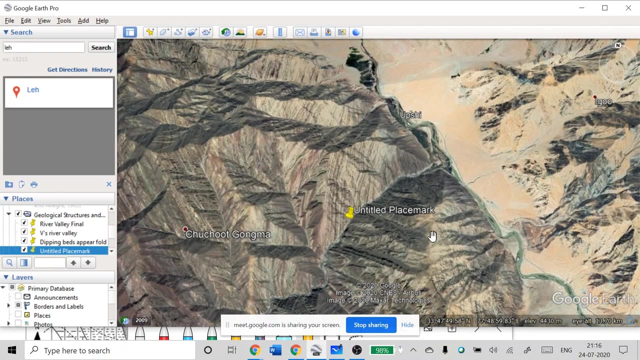 highway you will go through, and here you see these very nice- let me orient it so- these, these beds which are dipping towards southwest. so they are. you see very nice expression of this. so now there are two things that you have to understand from this view: one is topography and other is the strata. so 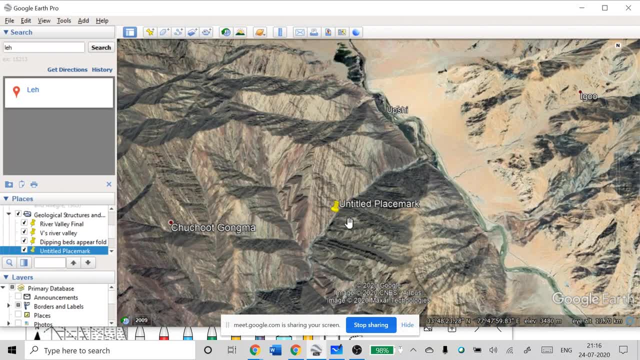 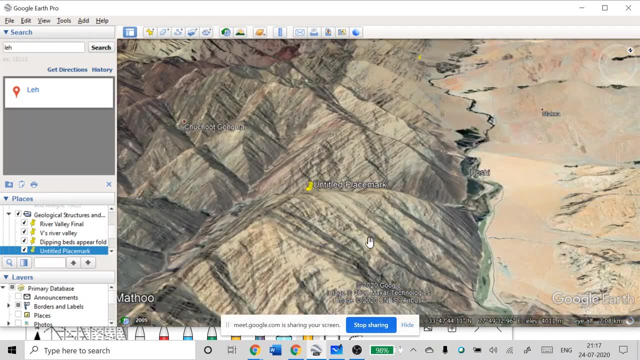 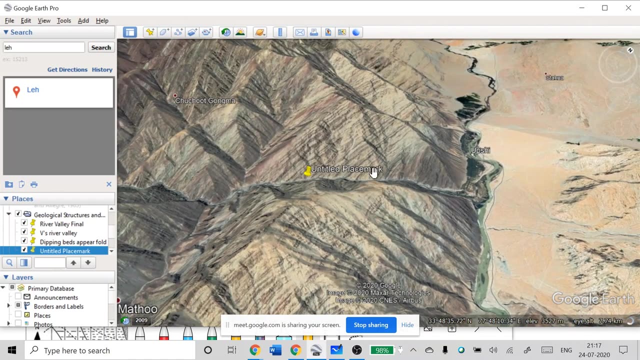 the these layers that you see here. they form the strata and this top graph achieved during the orientation of the boulders in dhu math. this is the topography that you see here, the variations in elevation. so that is topographies. topography is formed due to action of the duty, action of electro. 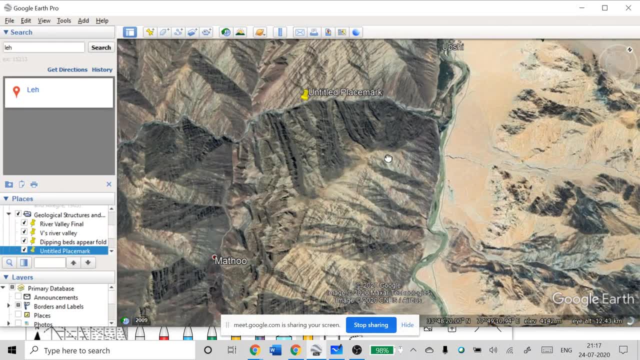 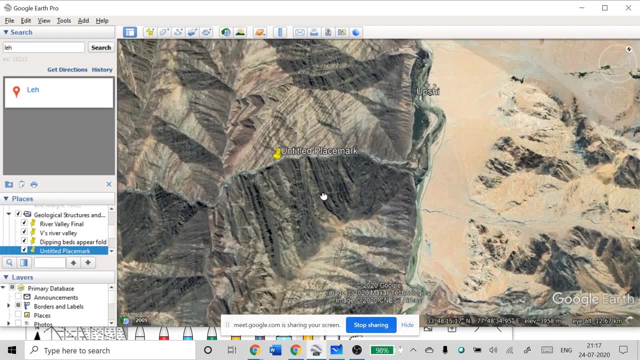 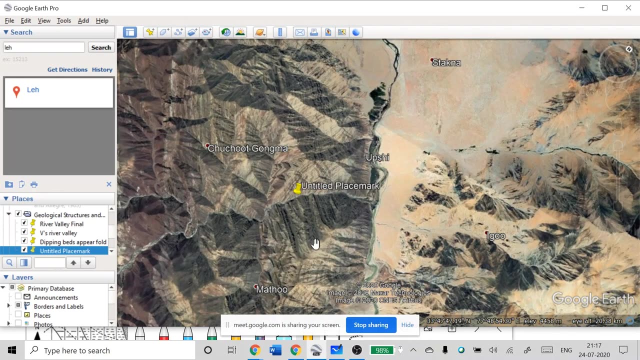 erosional in such as wind, rain, all these things. so they will produce the surplus surface topography in this region, which is once elevated. example here: what you see in this case, strata, is something that was that if it's sedimentary, it was sedimentary layer and in some case you will see foliation if it is metamorphic domain. 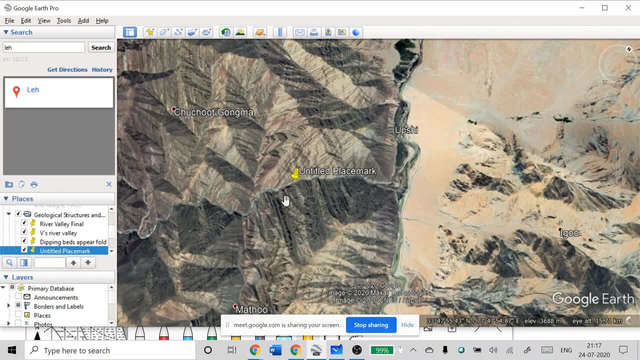 and this strata if it is tilted. so you can assume that there was some tectonics, because principle of original horizontality says originally these were, these were all deposited horizontally and now you see if you see them dipping. so there, there are some exceptions to principle of horizontality. but 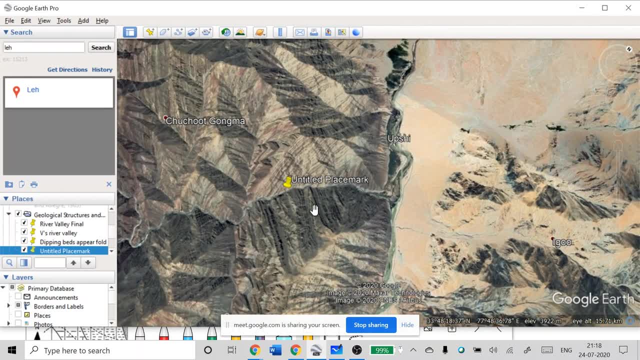 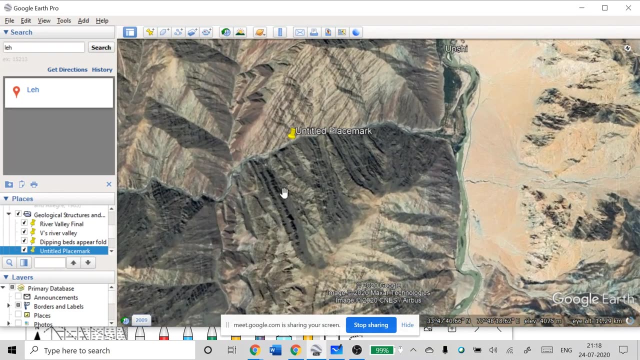 you can see, there has been some tectonics which has tilted these. so here we see these planar plane, these planar strata, which is these are cut by valley, so there was initially no break in continuity. so you see this strata here and this strata here, so this is continuous. only thing is in: 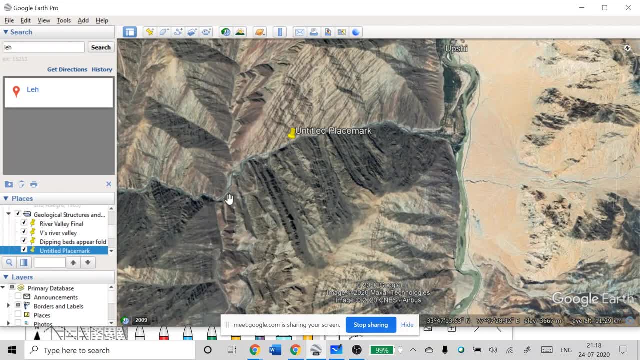 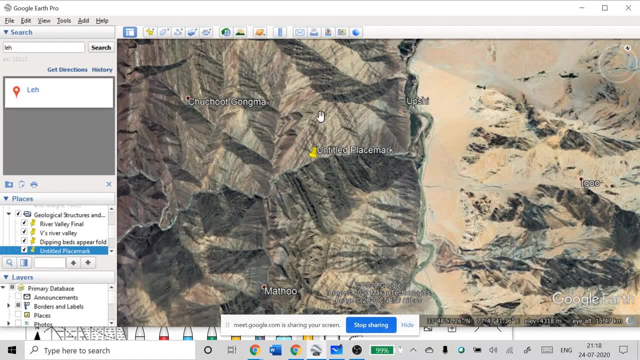 the middle, it has been eroded, eroded by, by the river which is flowing here. so this, this is the topography and the strata. strata are these planar features which we are considering here and now. after some time, we will also learn the concept of stratum contour. so we draw contours. so if you all, you already 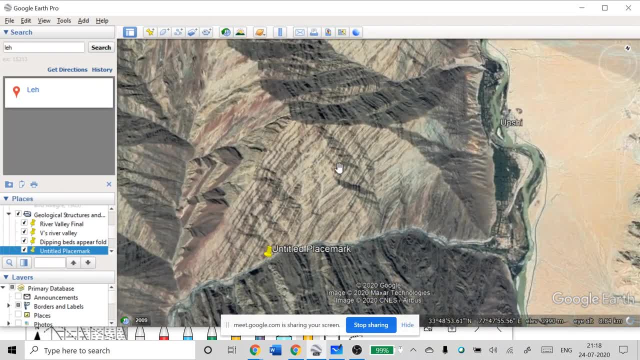 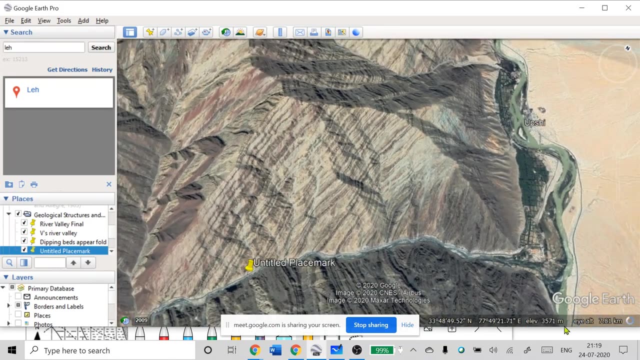 know what are contours. so for topography, contours are lines which join points of some equal value. that value could be anything, it could be. you can draw contours for elevation, so those you will call them elevation contours, which you see in topographic maps. so, for example, if this elevation is here and you can read these elevation values here in googler. 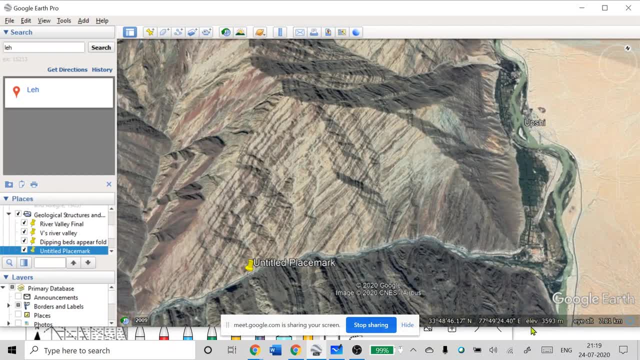 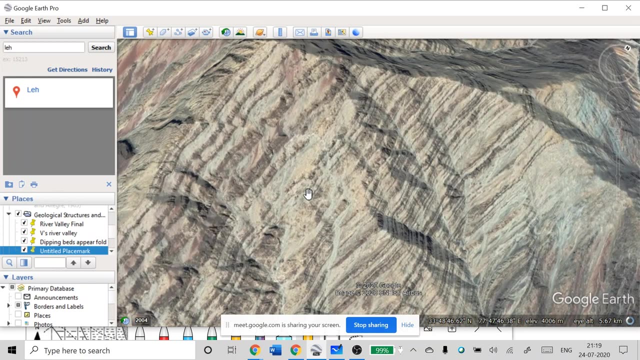 so that is very nice about this. so these elevation values you can read here. so, for example, if i click here, it's almost four thousand meters, and if i go down near the uh, near the valley slope, it's thirty six hundred meters. so what you can do is, if you want, to draw a contour. so we have all. 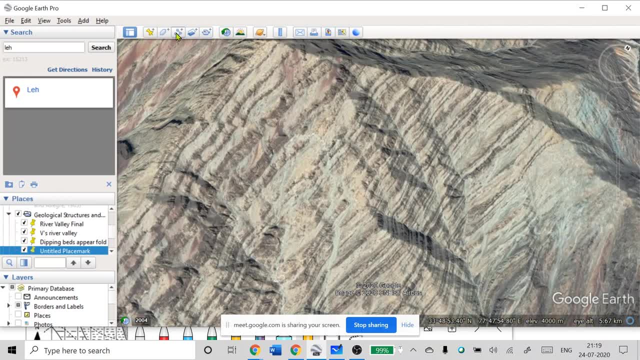 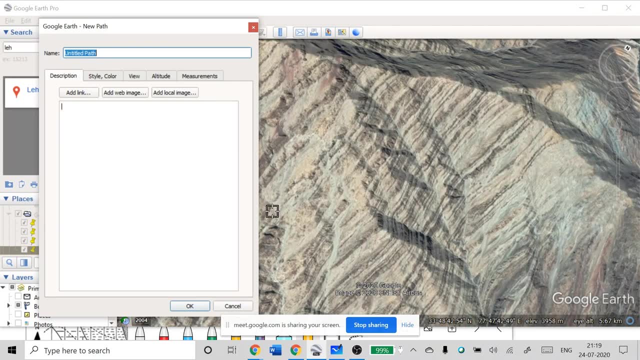 shown in recorded lectures. but if you still need to draw in google earth, actually you can go here, add path and you can actually click here how the contour will look. so, for example, if i want to draw four thousand meters contour, i put a point and then keep looking at this elevation value here so that you have points of equal elevation. 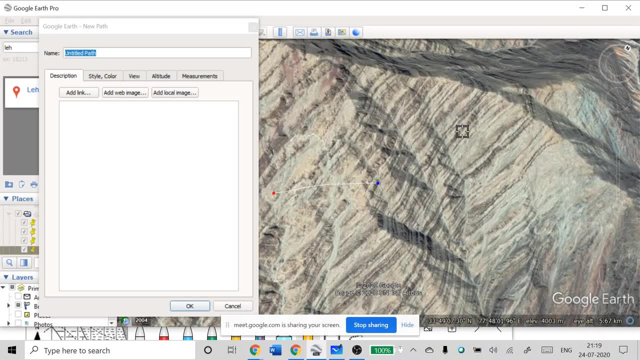 so now i could just point it here, or some the yeah, somewhere here, so you see, you can see it will turn, turn around like that. so these are almost 400. so you, these get folded because of there is there is another small sort of stream, but slump that is there in the middle, so that that is affecting these. 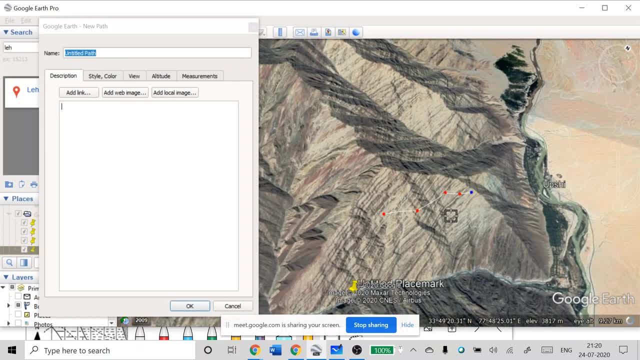 contours. so now you can finish it and it will actually turn around here and it will go here like this: and if you draw it here, so it will cut the river here and come back here. so you see what will happen. so this stream is joining this- uh, bigger stream. i think this is indus and this is zanskar, so it is going. 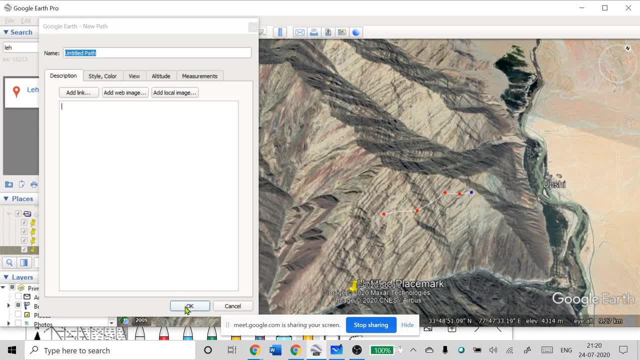 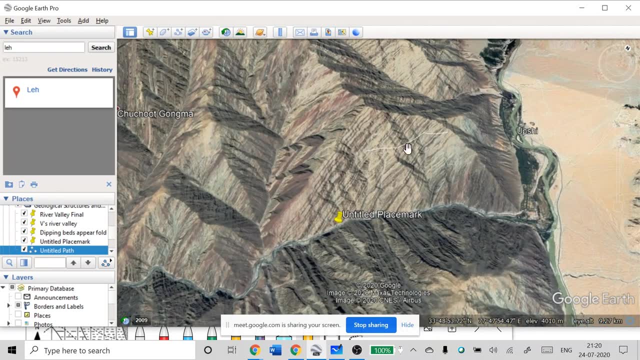 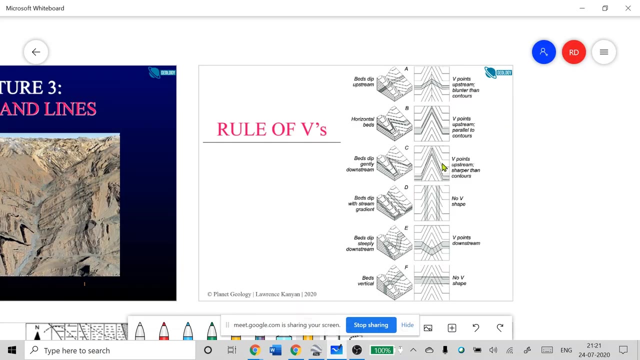 from west to east here this stream. so you this is sort of a contour line, you can continue it and it will give you the whole contour pattern. so here we were looking at elevation. another thing now. this is these type of contours. they are known as topographic contours. so if you go to this map here, 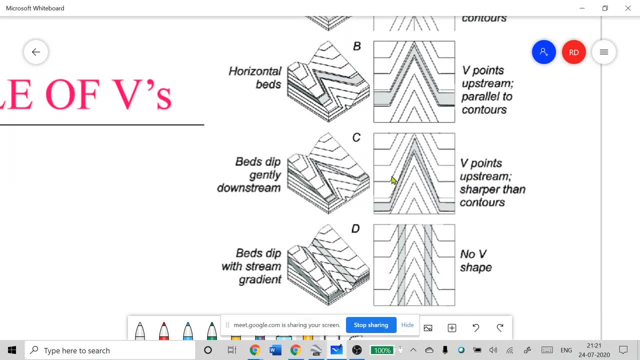 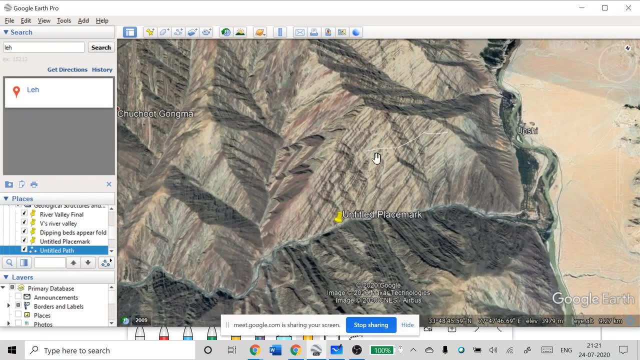 so these, these that you see here, these are the topographic contours which, which i just drew, not the shaded part, but these dashed lines, these are the contours. so this is what i'm drawing. so if you come, if you continue this thing, so it will come here and go something like this, so it will. 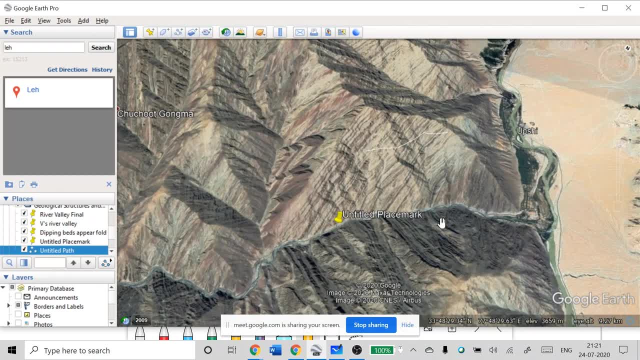 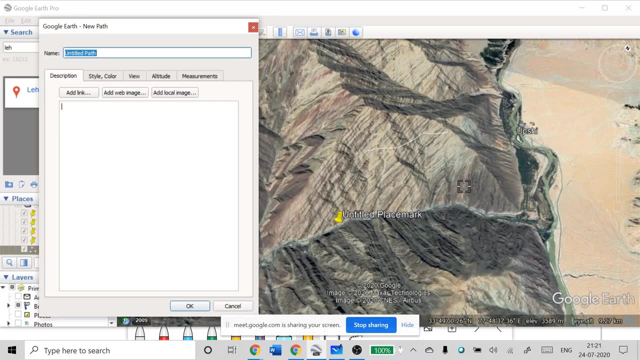 form a v. so let me very quickly tell you, because here the slope is not that huge as you would see, for example, in the example you had included, but overall it will look. in this part it will look something like this: so this will be your topographic contour. so 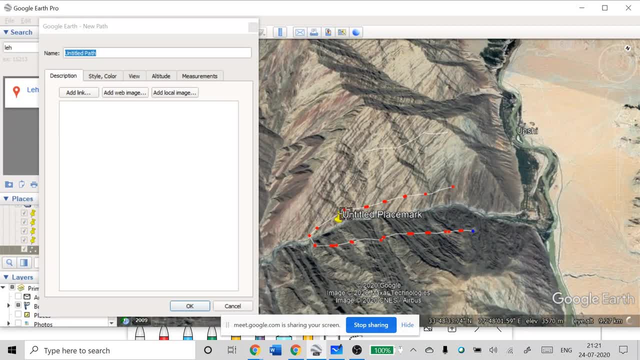 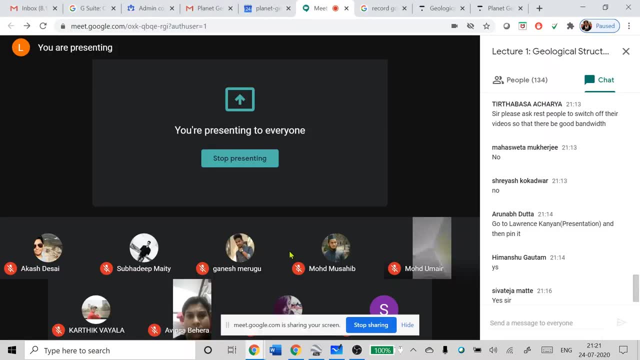 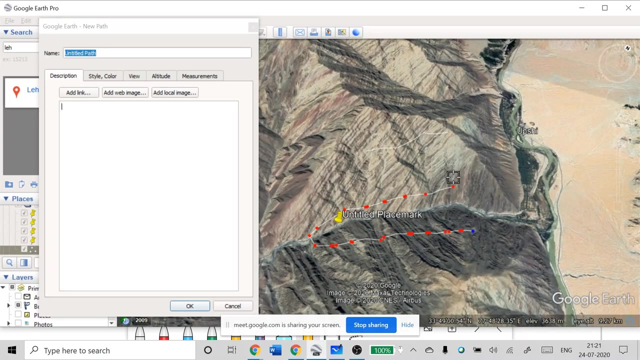 elevation will be same everywhere in this case. so i've drawn it. i didn't look at the elevation values because that will take a lot, a lot of time, but you can see how, how you can continue it. yeah, so this, this is a topographic contour. you can draw it like this: 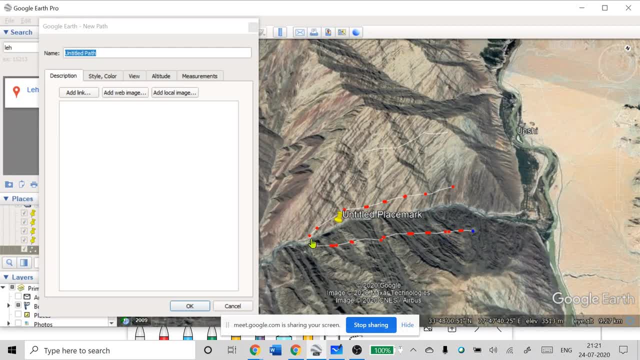 okay, we can't really see what your keep in mind, uh, because this is spent so big in my mind. but if you look at this value here you can draw some moyens like this okay, so then you can draw this contours and so you can see here, for example, you can also draw more for more values, for example. 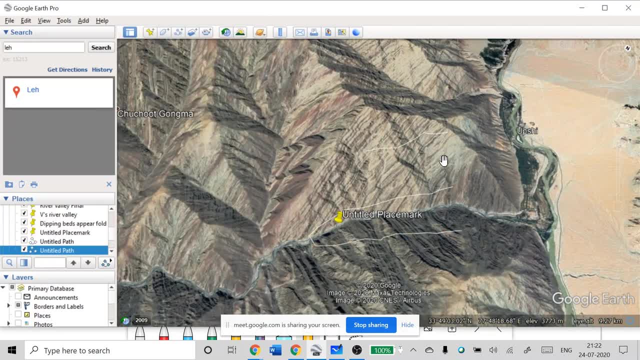 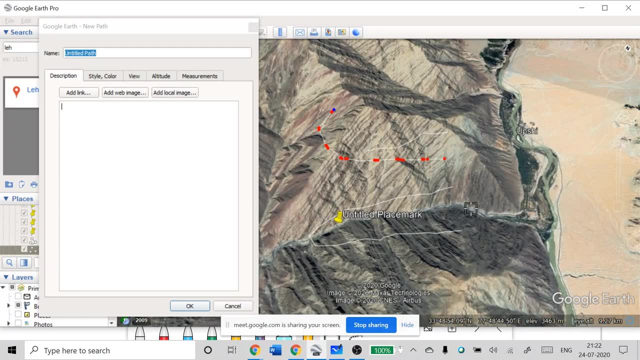 if this was three, five, eight, nine, so you can draw. you see, here it is also three, five, five, sun, so more or less same. so you can draw another one here, for example. but okay, let me, okay, so then you can draw some other contour, also for other value, and it will probably go. 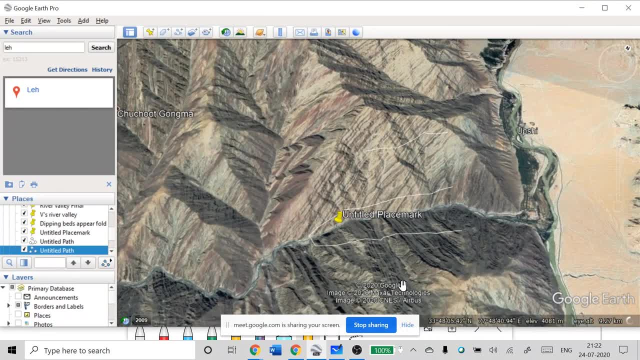 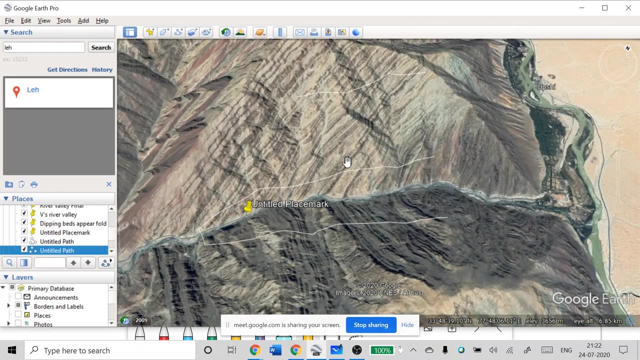 contours. now, another thing that you should understand so is the concept of stratum contours. we will come to that. actually, it's better, we will study it right now. only so here, if you see you pick any stratum which is continuing here. so for stratum contour, you need two points, which 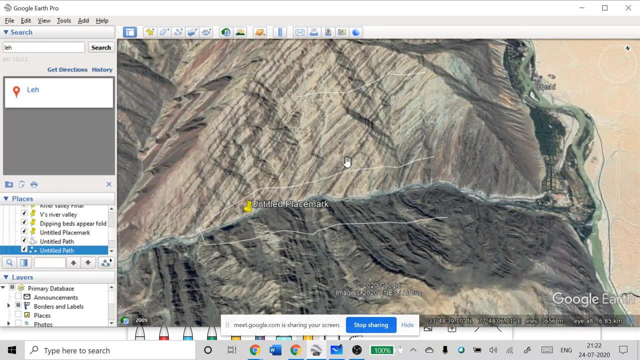 have same elevation. so stratum contour is nothing, it's just a strike line. so for a planar bed, for example, here these are planar, so it is just a, it is just a strike line, but we don't say like all. so strike line is a stratum contour, but not all stratum contours are strike lines, because 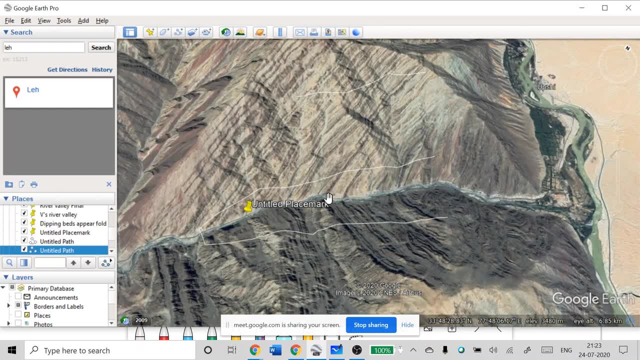 some features, for example, if you have folds. so in case of folds you have for one limb you can define a strike line. but if it is undulating surface you can- it is very difficult to define strike line. so that is why we use the concept of stratum contours, so what we call them as. 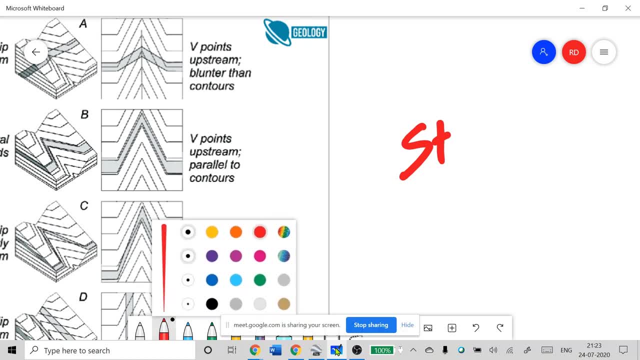 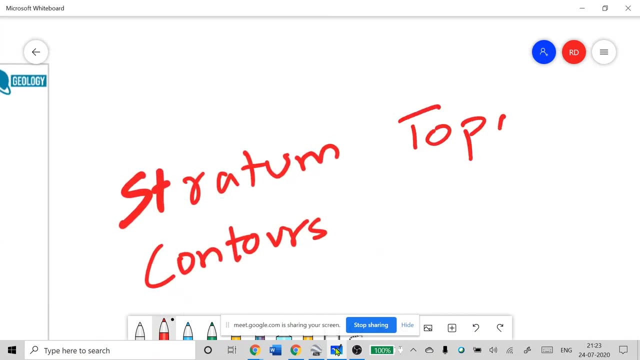 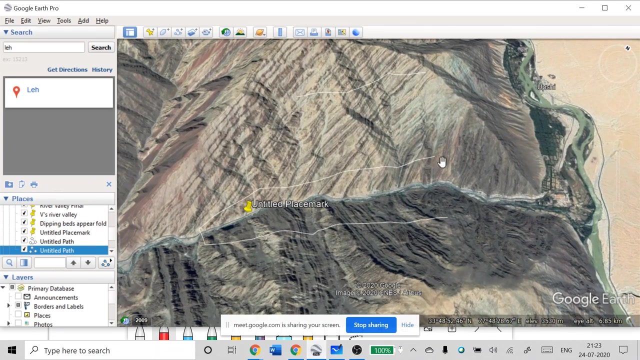 stratum contours, so you should understand the difference between these. and another are topographic contours. so topographic contours- we have already seen the one that we drew here- this is a topographic contours, so you should understand the difference between these- and contour, so it joins points of same elevation, whereas stratum contour you cannot move from. 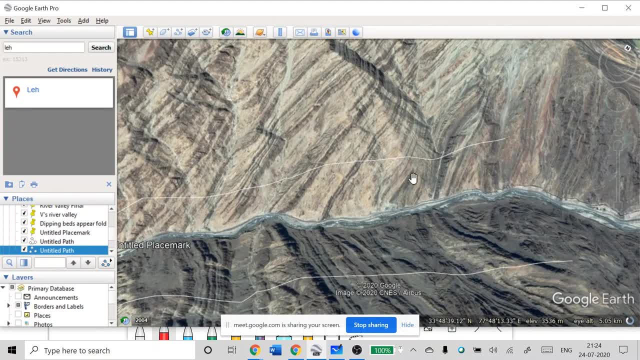 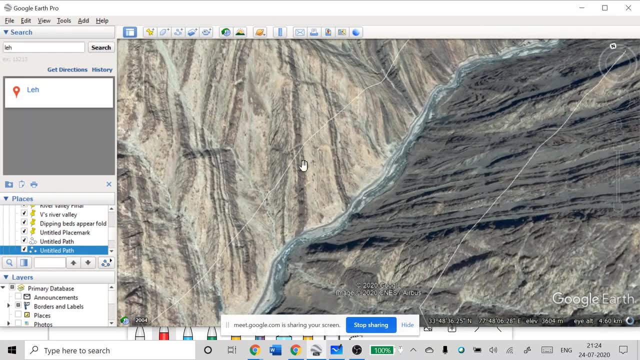 one layer to another. so here you see, we are going from this layer to this layer. that is allowed because we are moving along topography, in stratum contours, for example. if you see this, maybe somewhere it is exposed. so this bed is right here, so you cannot go here or there. so 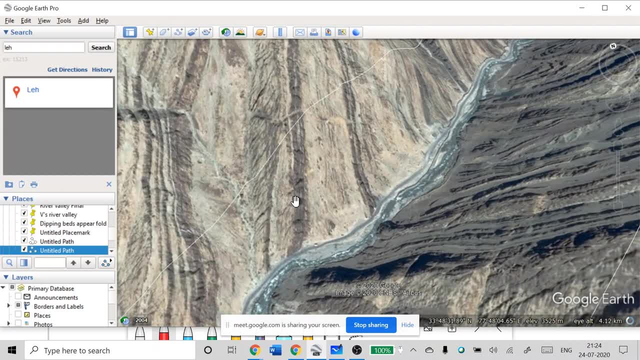 you have to stay on one plane. you cannot even stay within one bed, because a bed is a three dimensional feature, so but the contact between two beds, that is a planar feature. so if you are along that, for example, if you see this bed, maybe it is continuing on this side, so you have to stay. 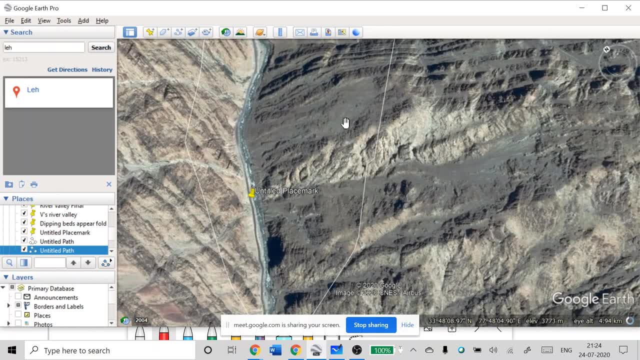 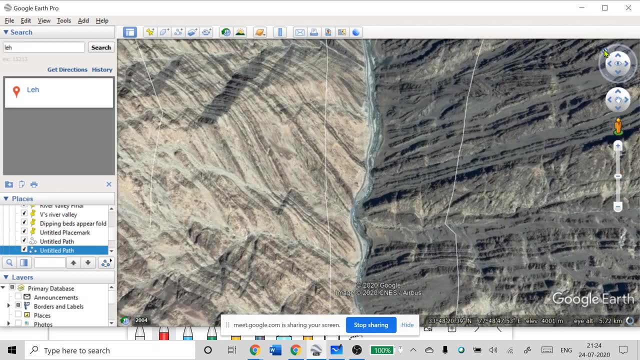 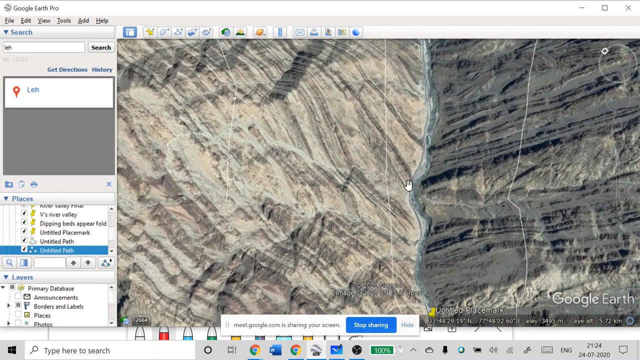 on same bed for. so here, if you have to draw stratum contour, so it will also be a point of same elevation, but you have to be on same strata. so let's see, yeah, so now you can see this, we can take this bed which is continuing like this. so 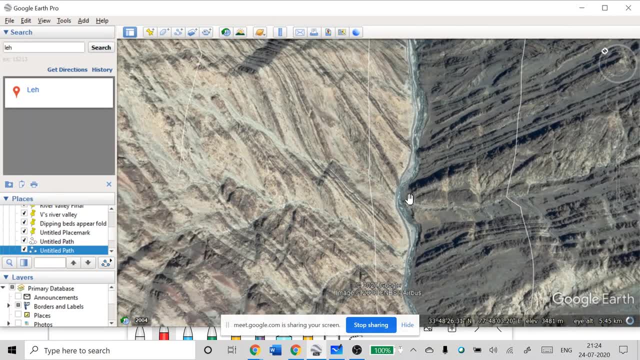 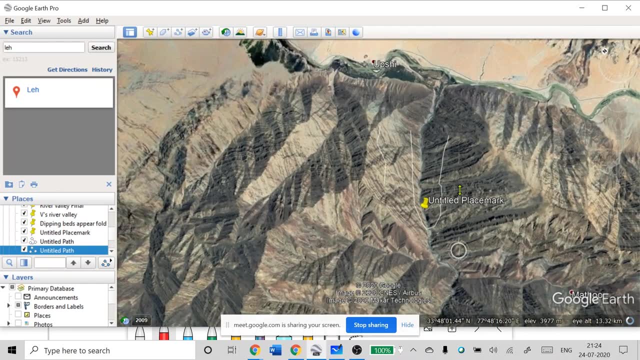 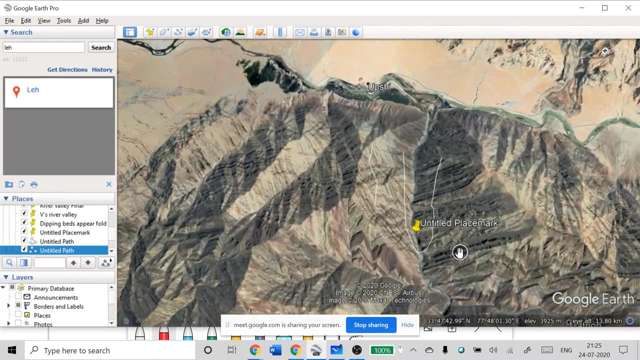 you can call it strike line also or stratum contour also. so what you can do in this case to draw a stratum contour. and another thing that i have before we proceed is that you see, these v's are forming. so these one v is formed by topographic contours for the valley and the 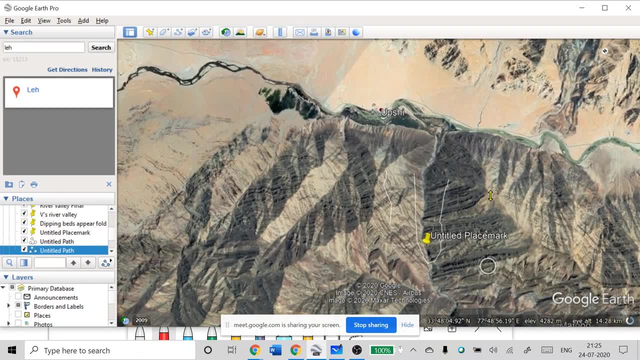 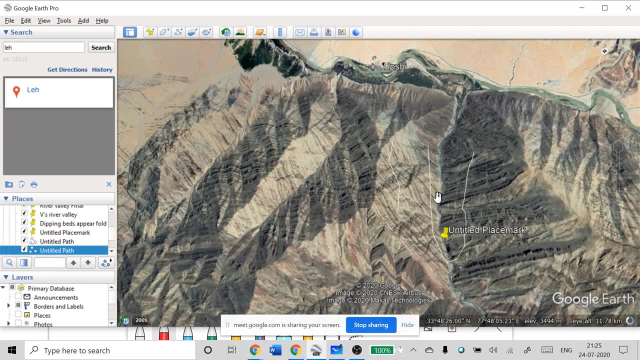 outcrop pattern, or the trace of these surface, trace of these beds. they are also forming these v kind of features and what you see in this case is this v is pointing in the same direction as the topographic contour. so this v is pointing in the same. 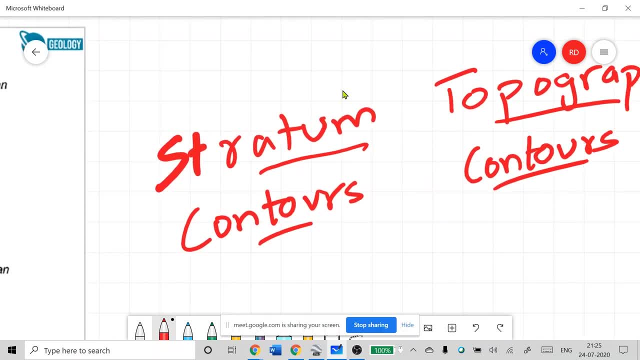 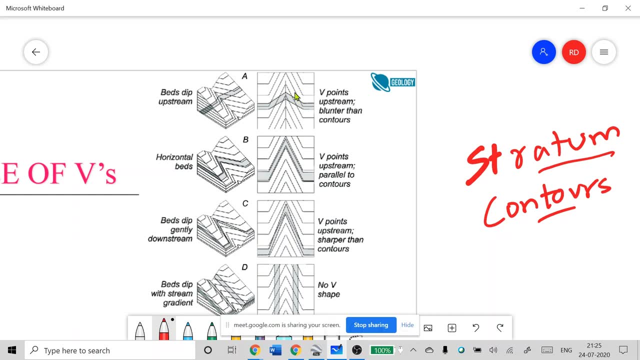 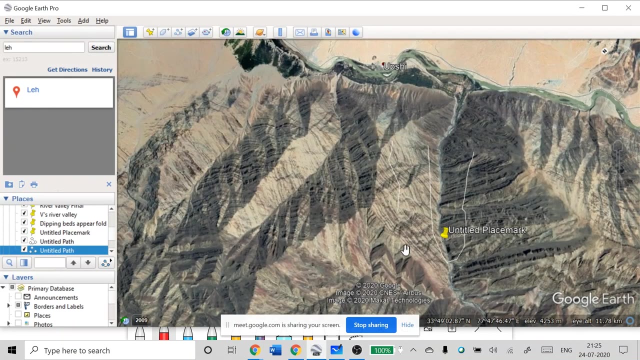 direction as topographic contour. so if you go to this image, so it's one of these cases, so in the same direction. actually, contours are much gentler. so this is actually the beds are dipping upstream, this case, and you can see also. so this river is coming from this direction, beds are dipping. 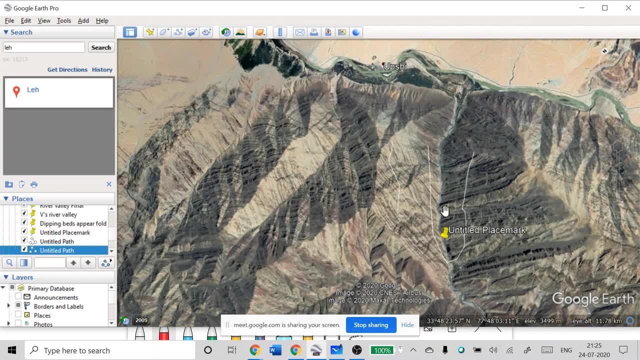 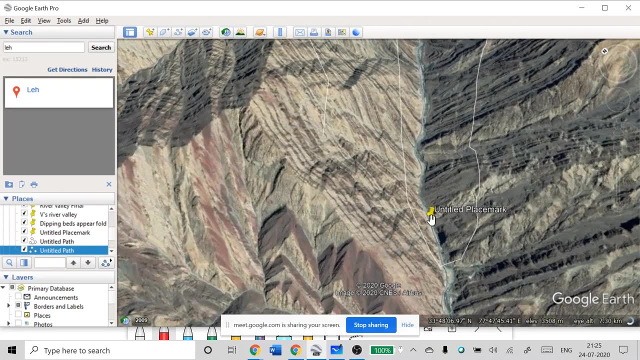 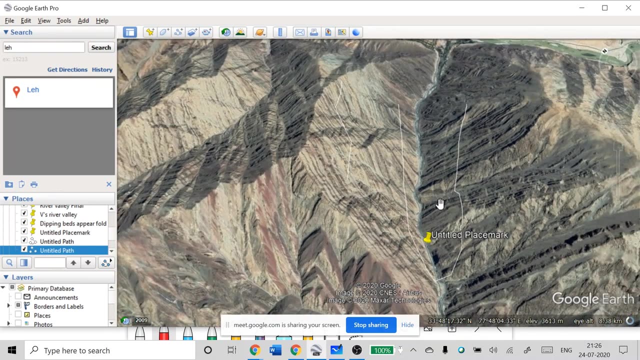 upstream, so they are pointing upstream also in this case. so this is, I think, in the silver and it's joining it. so you see, the V's are pointing in the same direction. now another thing that you need is some strike line so someone can. so I will just tell you how you can. 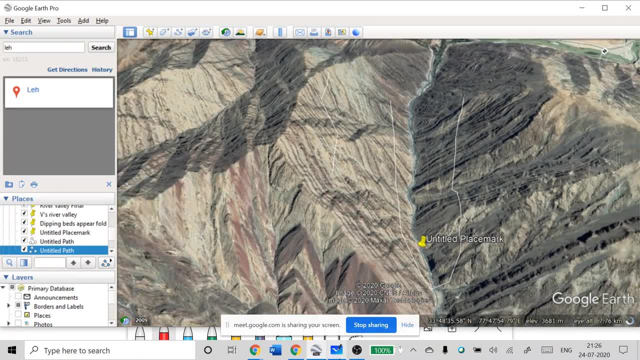 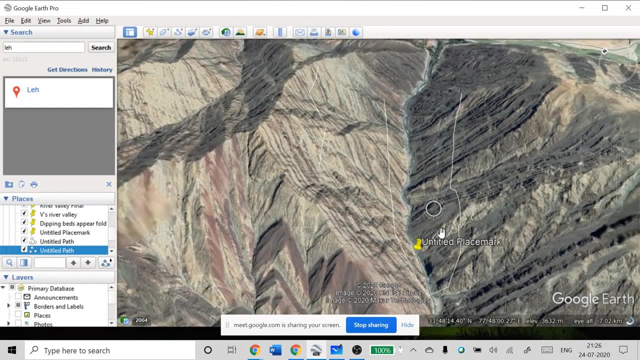 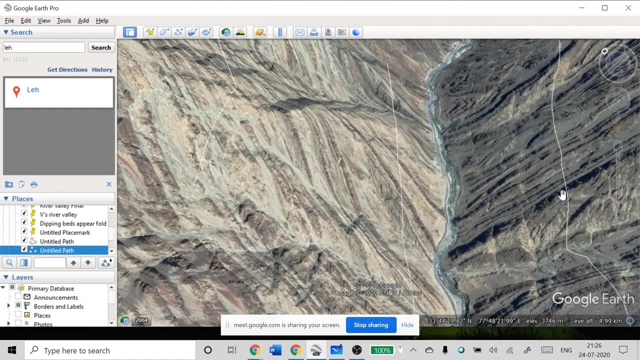 actually, actually, you don't need to cram this whole thing. you can actually solve it very quickly. you just need to draw two lines. so what you see here in this image, let's pick up any bed which is continuing. let's see, let's say, this is continuing like this, so this bed here. so what I do is I take, try to take two. 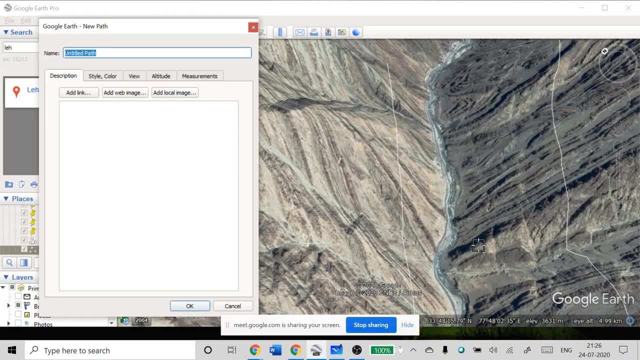 points of same elevation. so again, I look at my elevation here. so it's: yeah, let's pick one at 3600, the same you here, and let's say this: this is the same thing which is continuing here, so this is also we drew as. so this is, this is just a rough line. so this contour that I 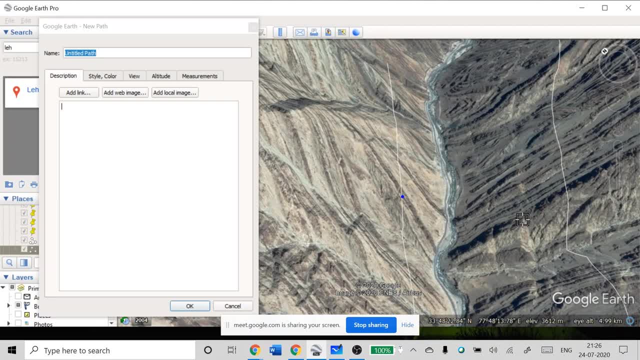 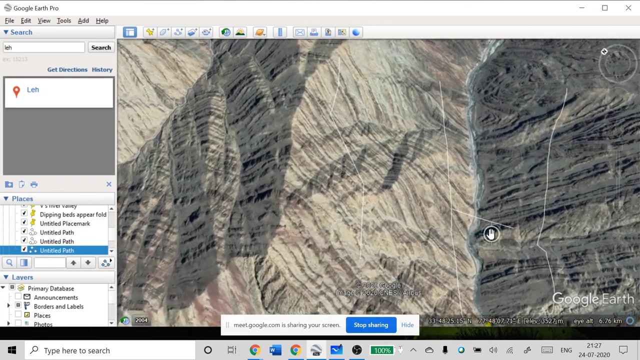 drew. I didn't look at the elevation, so it's a little bit wrong. it should come actually in this part. yeah, so this. actually it took it along the ground, but if you look it from above you see, so this is a strike line. now that you have drawn so this, because you see it is on the same bed, so you it's. 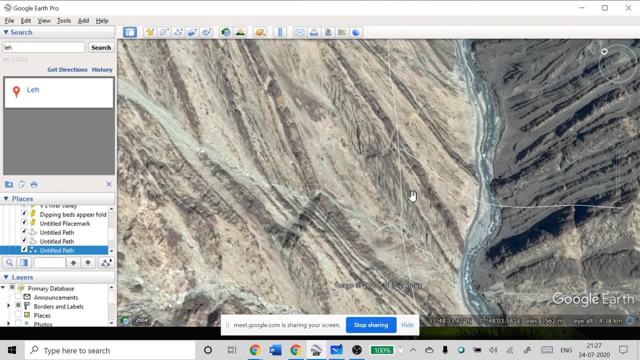 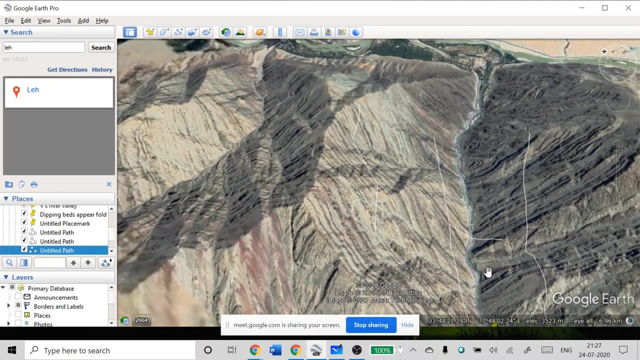 actually on the plane. that is contact. that is a contact between these two beds. so a plane will be a contact. even the whole bed is a three-dimensional feature. it is not a plane. so now I have got a strike line or a stratum contour, so this: 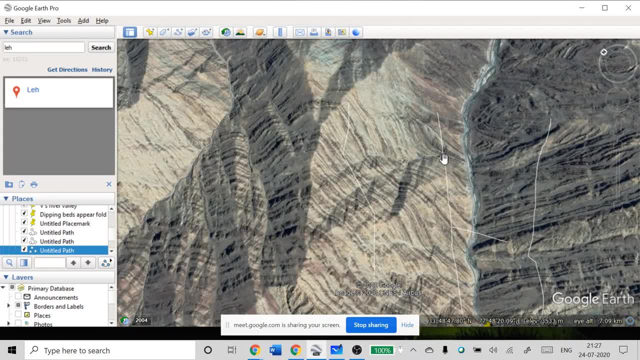 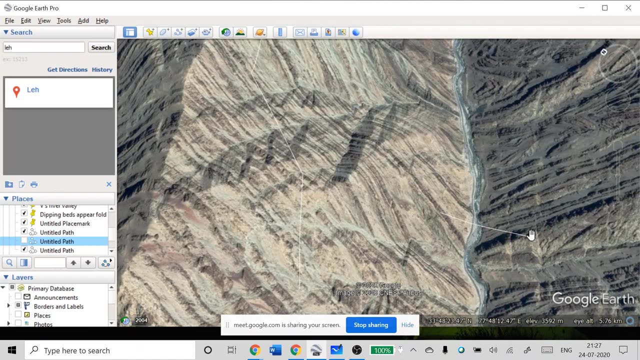 is known as a stratum contour. I will actually delete you go. this is more distracting. yeah, so this is a stratum contour that you have got because it has same elevation- we took 3600 in both places- and it is on the same plane and this is also a strike line. another thing now you can do is you. 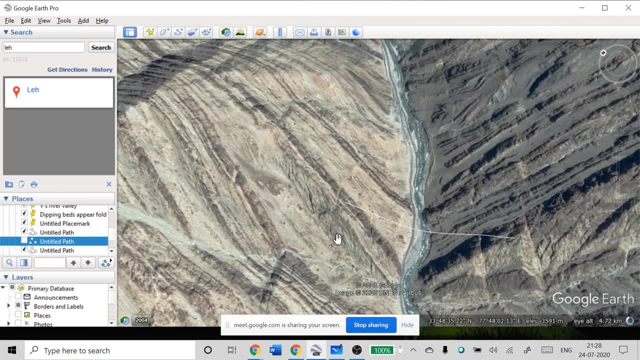 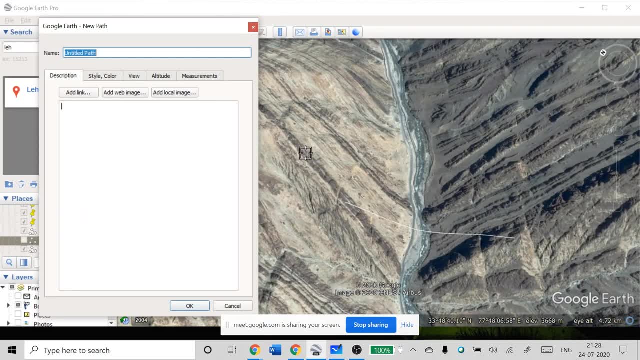 can take another strike line. so if you have two strike lines you can actually determine which side it is dipping. now to draw again, I'll draw second strike line. let's draw it at somewhere around 3700. so again, read the elevation value here. and it has to be. you see, they are almost. 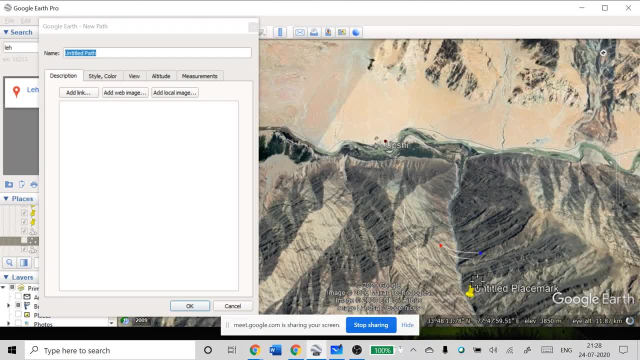 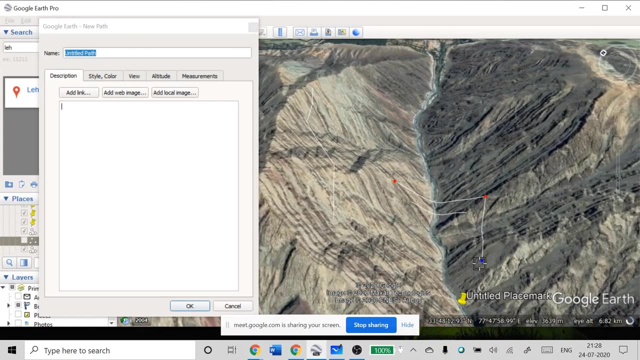 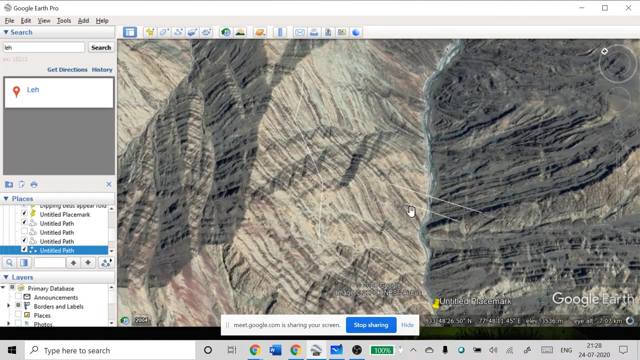 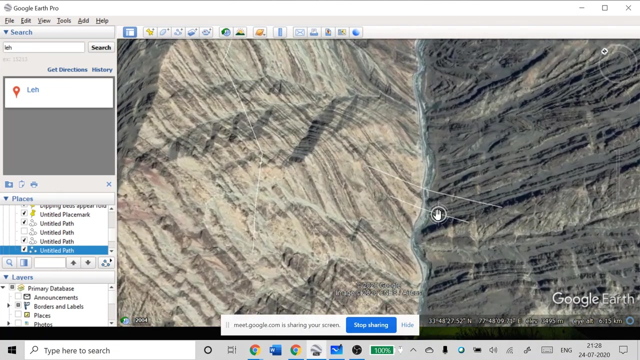 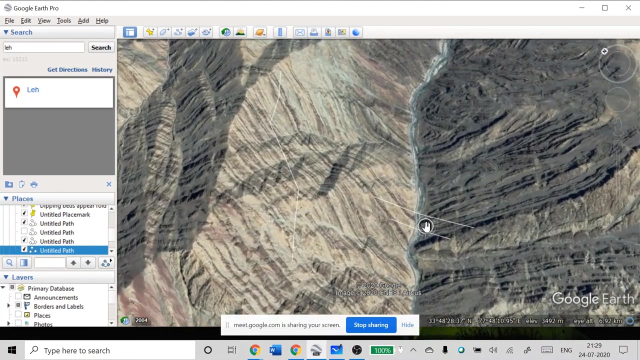 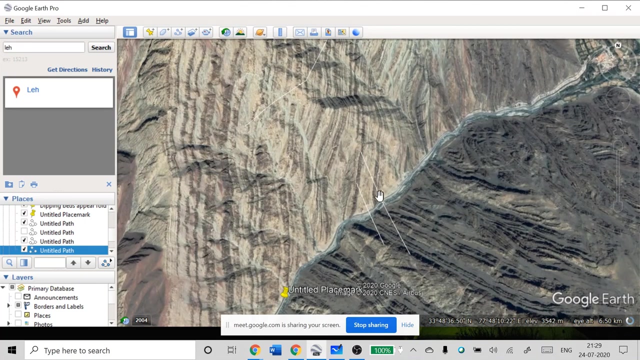 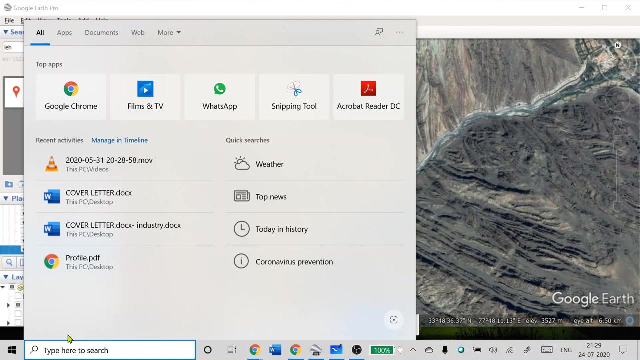 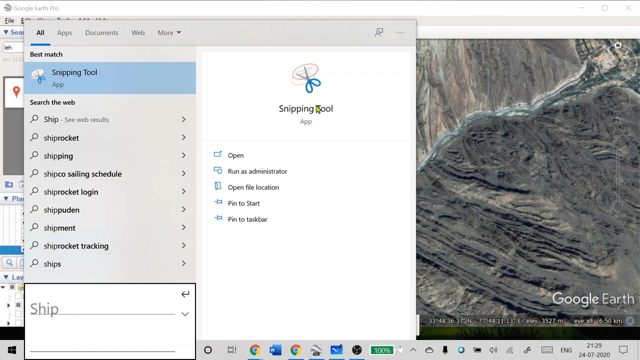 parallel, so not completely exactly parallel, but you get an idea. so these, yeah, you, you, yeah, so correct. so this is, the dip is towards the southwest direction and you can actually get it from. let me take a snip of this thing so that we can draw it. 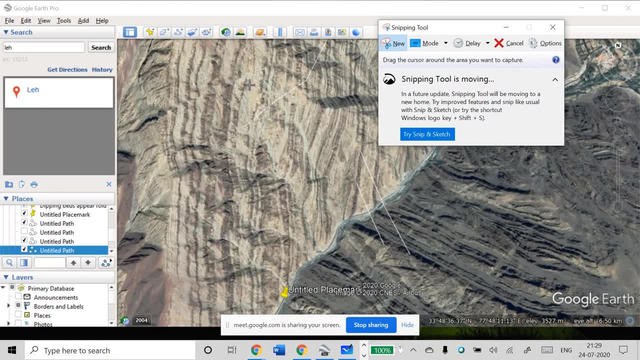 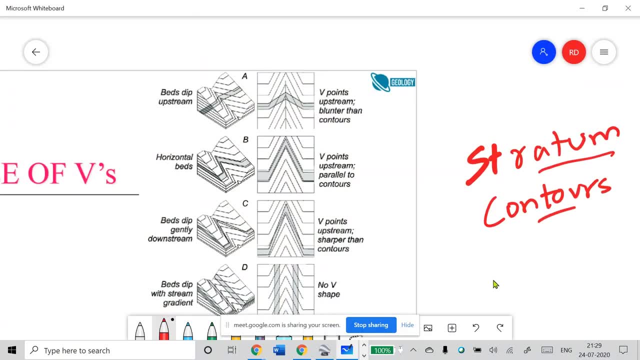 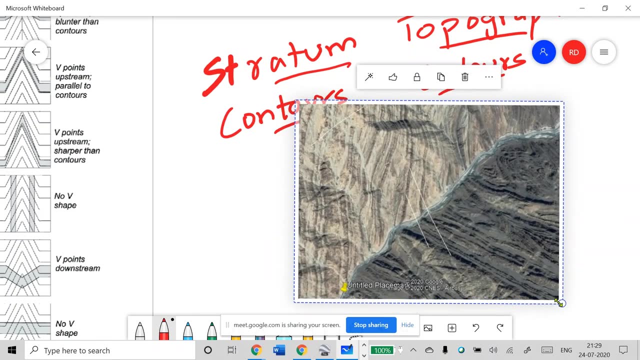 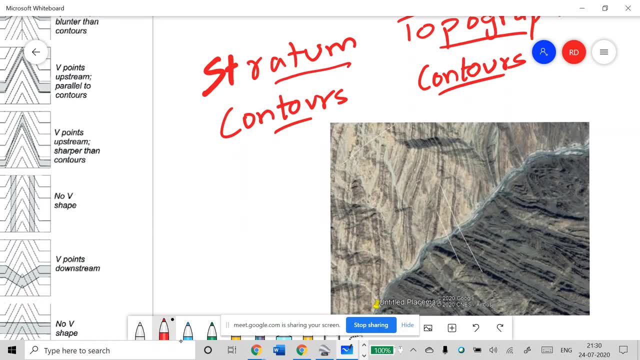 so now you see, so here we could not and it goes. so this is we draw at 37, yeah, anit grade, and this me direct 3600 for this me direct 3600 for drop, to examine it here. so i'll try to you see, zoom you. 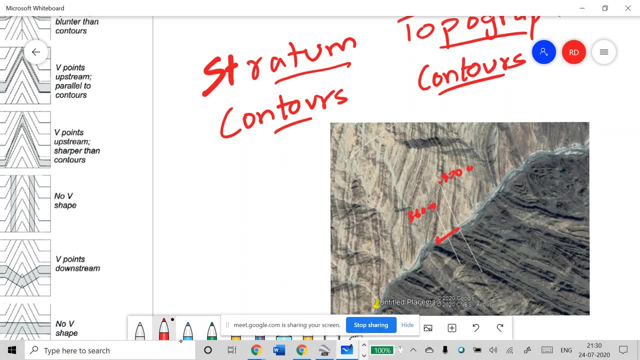 are. see, you have enough knot to trouble with the measurement. here you can see it. you are seeing the difference between these two targets. so this is, this is no 100. so dip has to be in this direction and that visually also, you saw it. so if you have to solve, 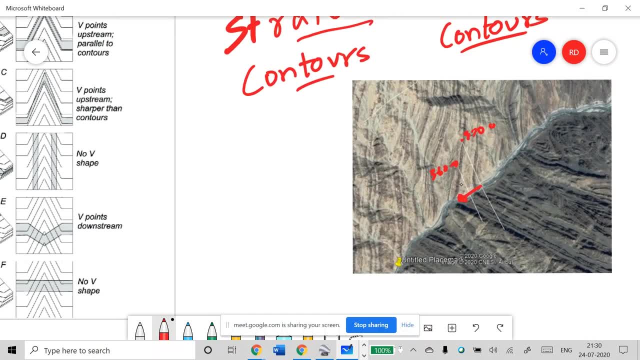 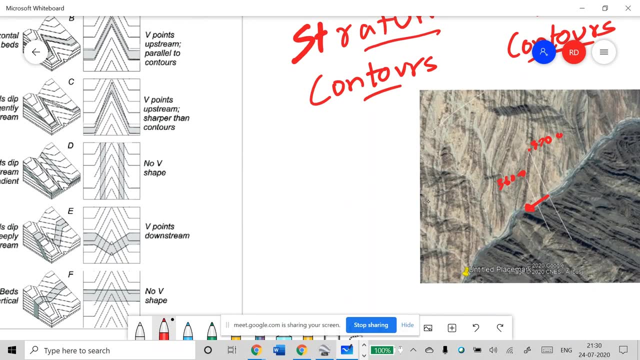 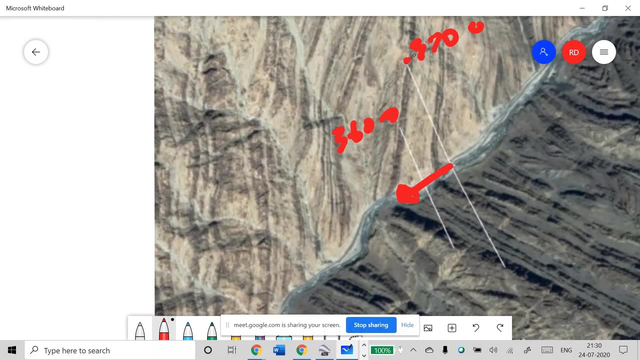 any questions of this type. all you need to do is just draw. try to draw these stratum contours. it will be very easy then to find in which direction this bed is dipping. only thing is, how will you here? you know elevation values you could read. so your only task is to just assume. 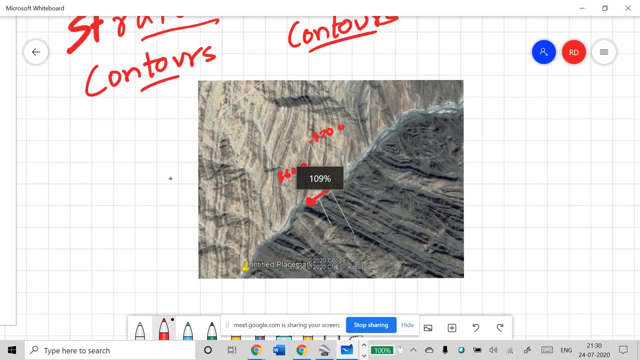 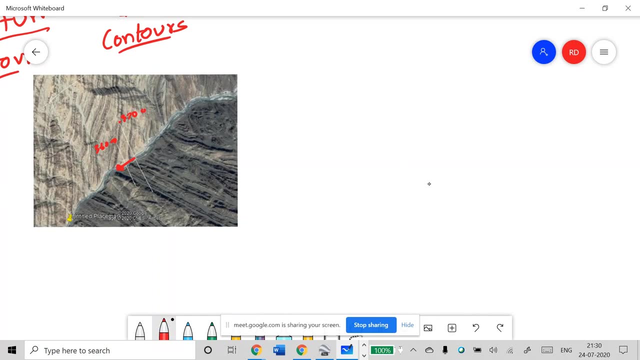 these values of contours. so usually you will be given. so just let me ask you question. then you know- because i we have not covered it, it's in the recorded lectures- what, what should be the what should be the v pattern in a valley. so let let me draw some topographic contours. so let's say 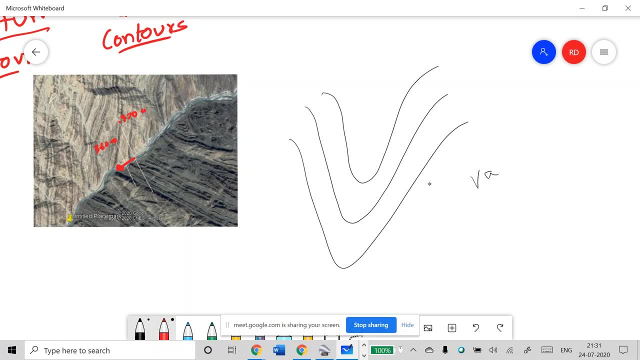 okay, so let's say: this is a valley, okay, okay, so in a valley. always remember that if stream is flowing in this direction, so the v will always point in opposite direction, so this will always have higher value and this point will always have lower value. so this is high elevation contour, for example. if you try to label these, 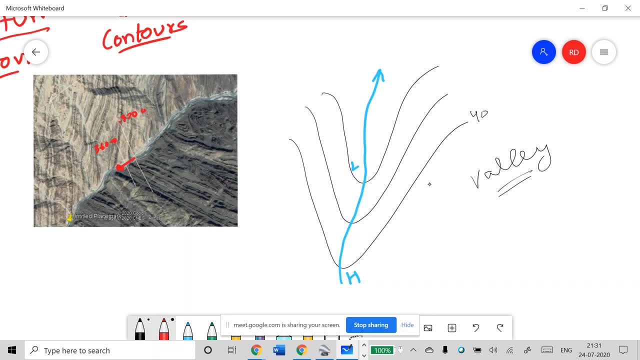 contours maybe, uh, this will be uh, four thousand three thousand nine hundred or something like three thousand eight hundred. so first thing that you should always remember. so if you have, if you go through previous recorded lectures, you will find that all this is covered. so we always points opposite to the this flow of stream. so this has 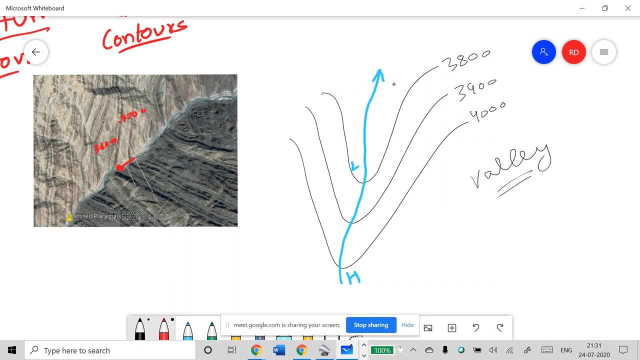 to be high area, this has to be low area. you can label them something like this: so these are your topographic contours. so what is happening? so here you remember, we drew a contour which went, which will actually go something like this: so this is three hundred six hundred thirty-six hundred. so 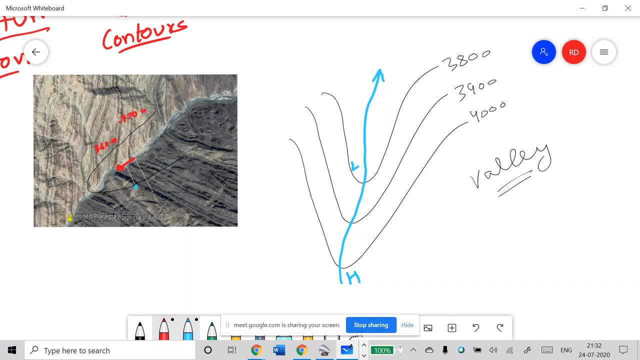 So these points it will intersect. these points, you see, will intersect and this is your stream flow direction, which is opposite of this, in direction in which V is pointing. similarly, if you draw 3700 meter contour, it will look topographic contour, it will look something like this. so, again, it will have to pass. these two points are both 3700, so it will pass something. 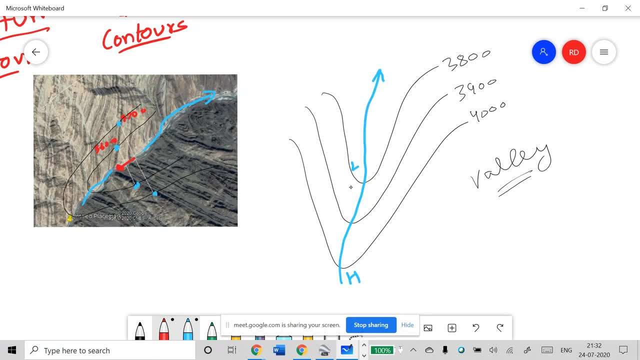 like this, so I'm drawing them roughly. so these, this is what is happening in this case and, on top of that, what you have. you have this topographic expression, so this, for example, with which we will consider one bad bed, which is the outcrop pattern. so this is the outcrop. 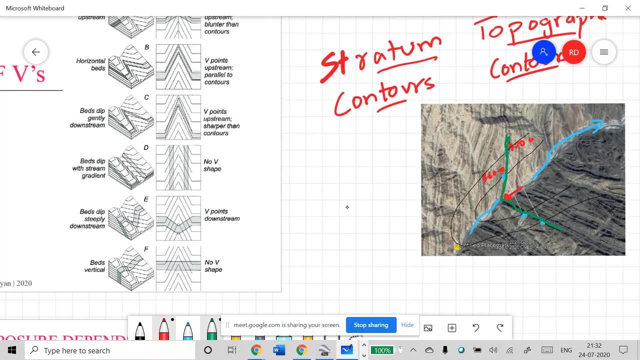 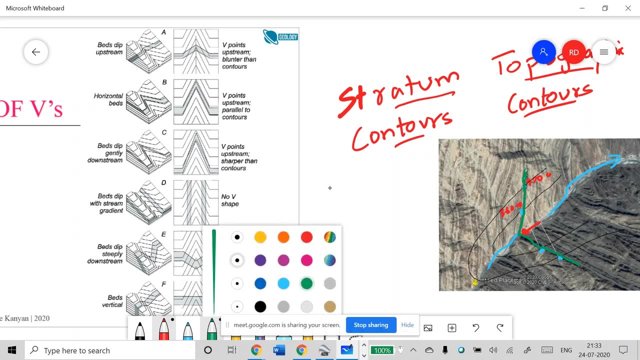 so these are the things that you will see in these kind of figures. when you see these figures, you see, so these are the V's topographic, and so these dotted lines, so these dotted lines that you see here, these, these are these contours there are. the shaded portion that you see is this: 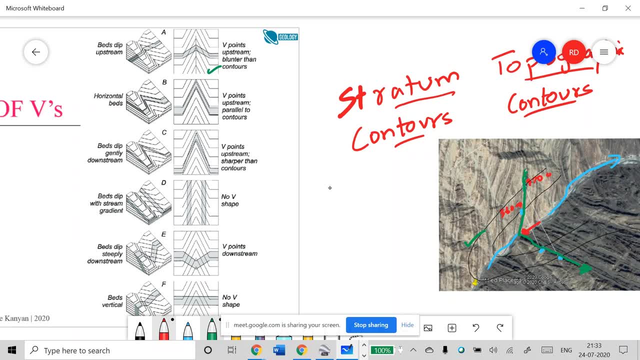 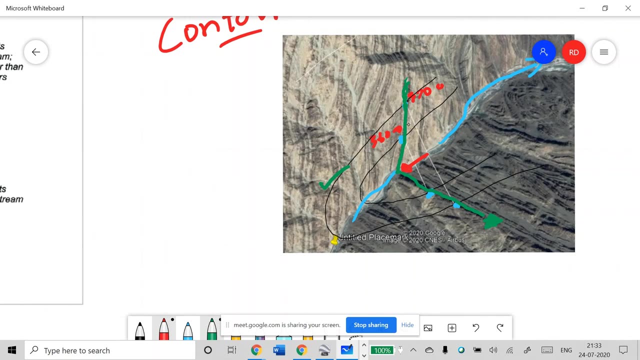 one, the shaded, so this is the outcrop pattern. so the green V that you see here, this is this one, and the dotted V's, they are topographic contours, which are these thin black lines in this case. now, you see, you need these points of intersection, so you be here, you see this. 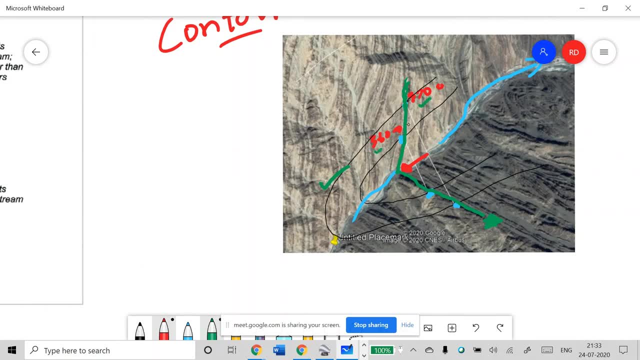 is 3700, this is 3600, so dip has to be in that direction. Okay, so this is the same principle that we will follow everywhere I will. I so this: this is one example in which beds are dipping opposite to opposite to the valley slope. so this is: 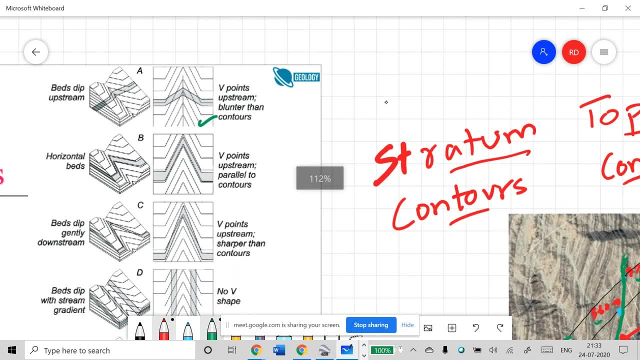 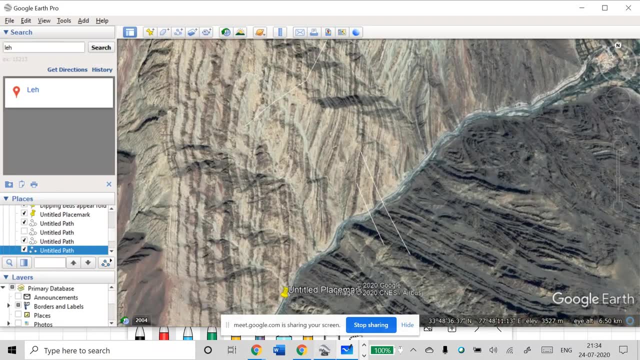 actually the first case that you'll see. I'll tell you also how you can easily solve. but before that, let's see few example in which probably opposite is happening. so if it is dipping in the same direction, do we have any examples of that? let me see. let me see. let's. 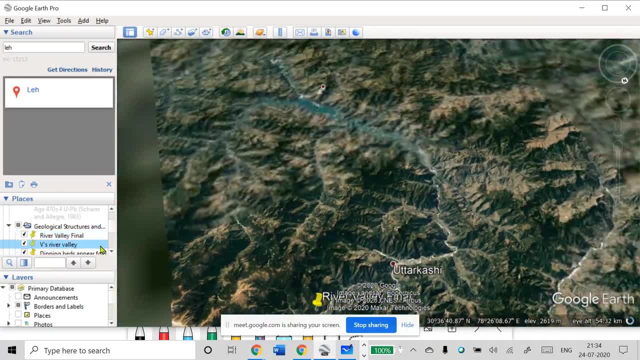 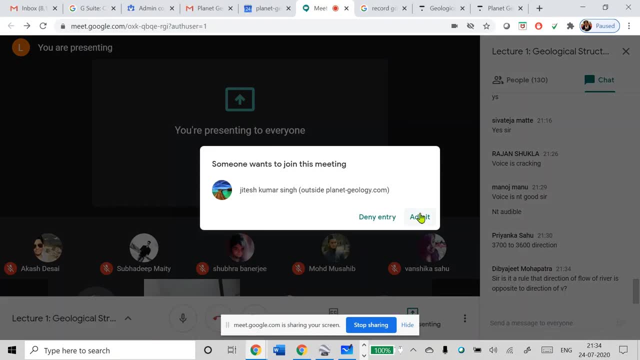 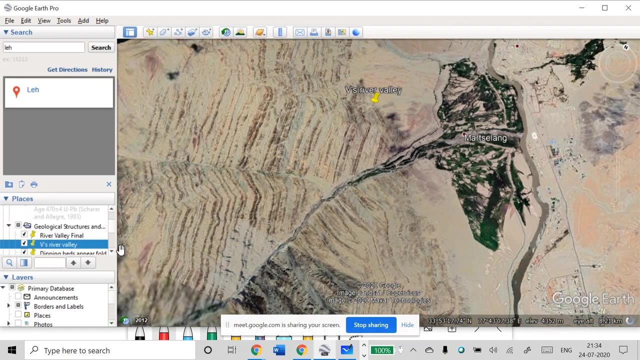 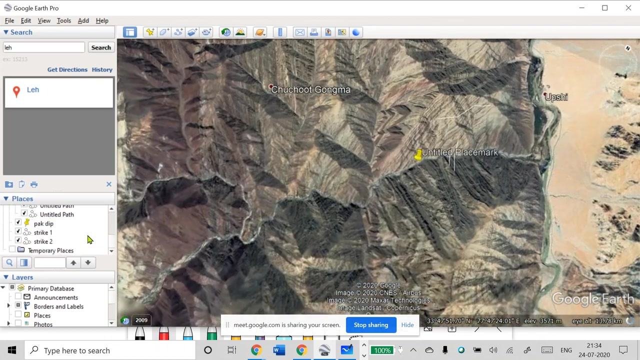 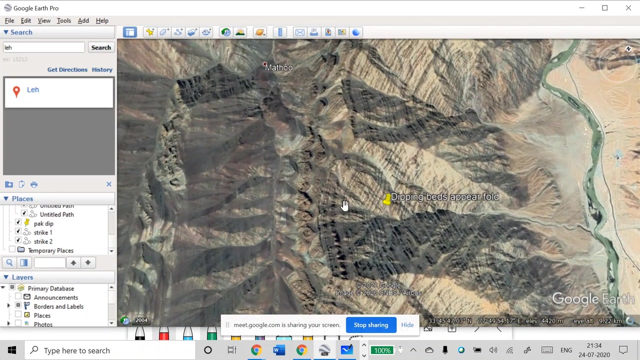 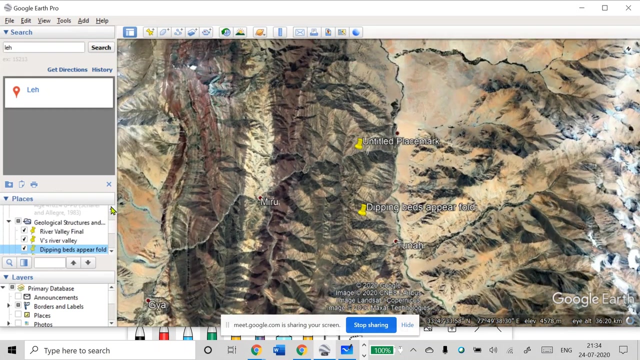 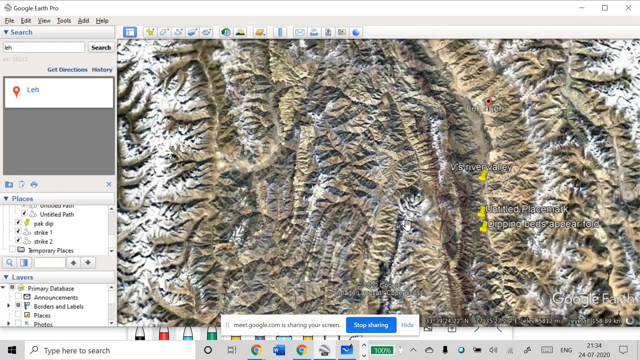 try to sort on this one other ribs. so this is also very similar, so we'll try to. the dipping beds appear like folds because of this topographic expression. so all these things that you see from top, they are so okay, what i'll do is i will share those files with. 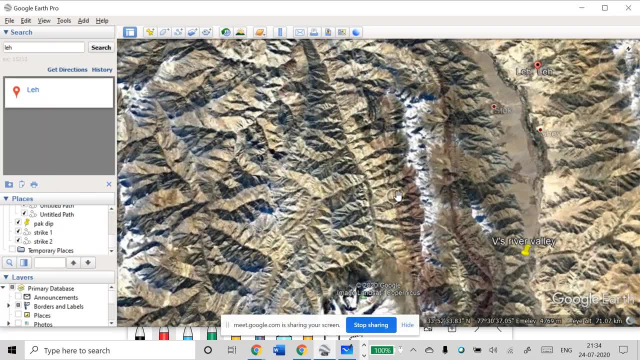 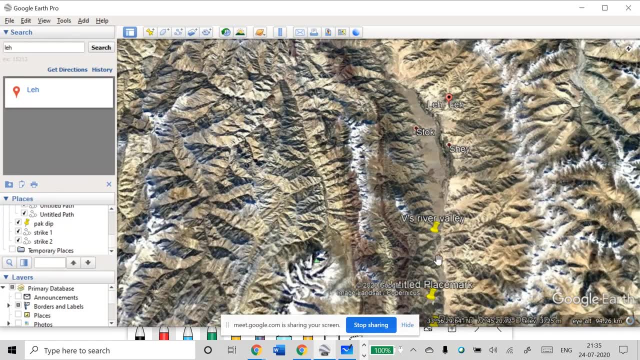 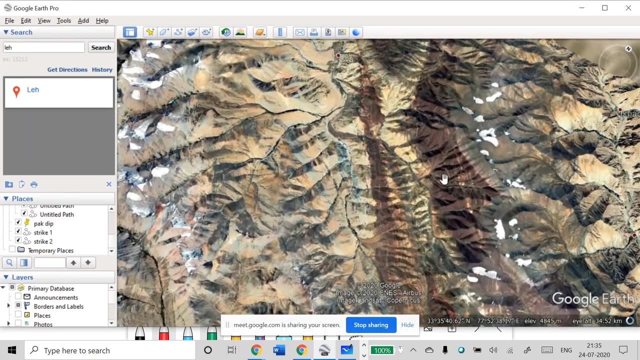 you so that you can look for them yourselves. but if you go to these areas, you will see that in some cases the pattern is slightly different from what you saw right here, in which the beds were dipping opposite to the valley floor. so what i'll do is i'll record that video. short video. 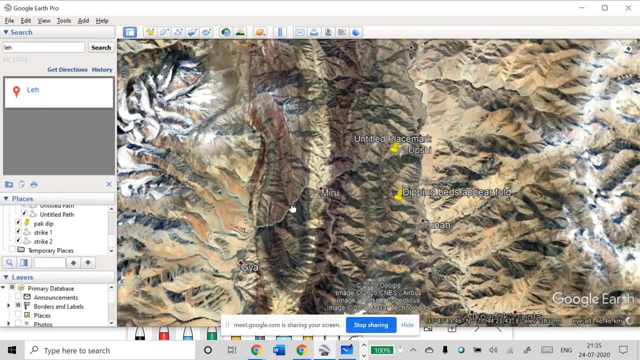 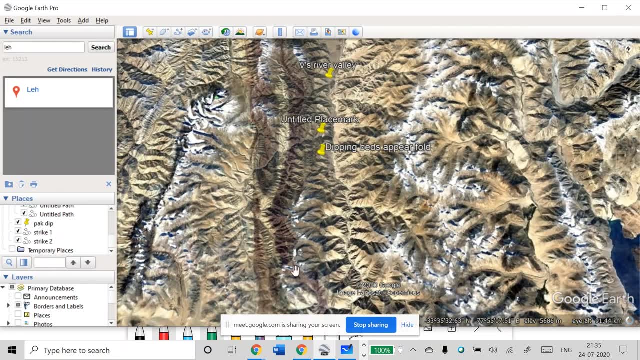 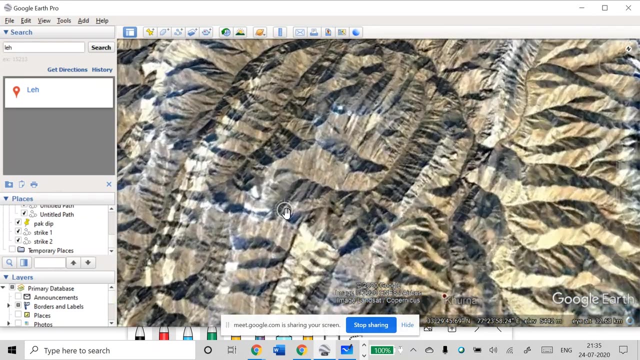 to show you the other. i'll show you other kind of patterns also, and then you could look all these and if you are curious, so what are these? does anyone know what these red, red layers that you see here, what these are, any guesses? yeah, here you are, nice, nice example. 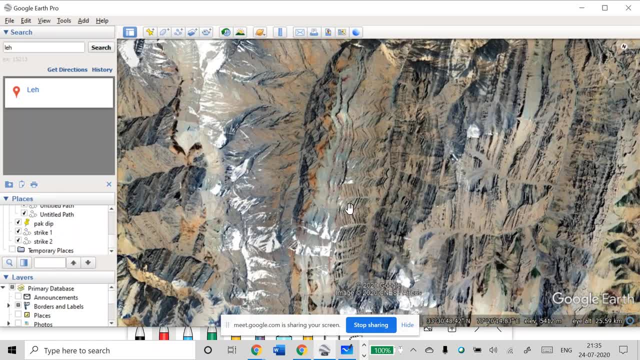 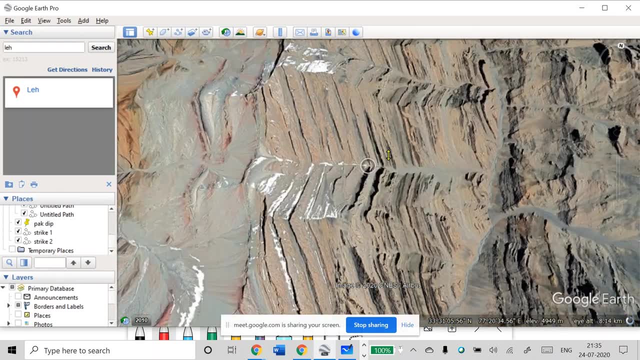 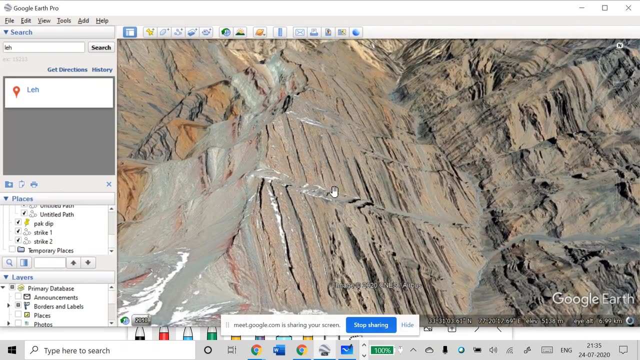 yeah, you see these v's here. look at this image. you can view from side. so what is happening in this case? so this is, we will consider this valley. so thus, if you look at the slope of the valley- so here i'm using actually these examples are good because they are vertically very steep, so you can. 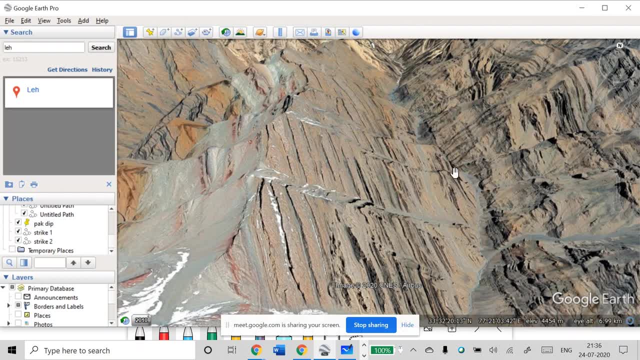 actually visualize even this stream- big stream that you see it has slope, but it will take very large area. so you can actually visualize even this stream, big stream that you see it has slope area because slope is less. so it is always better to look at these side valleys because they are 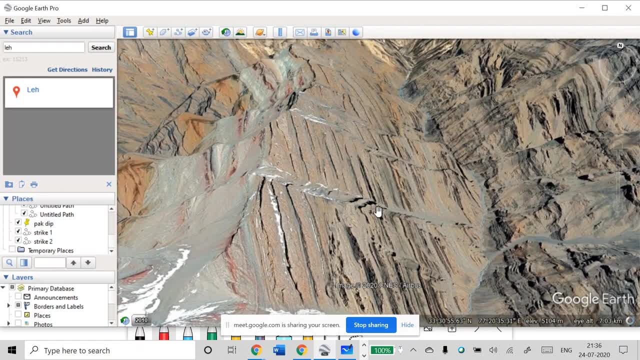 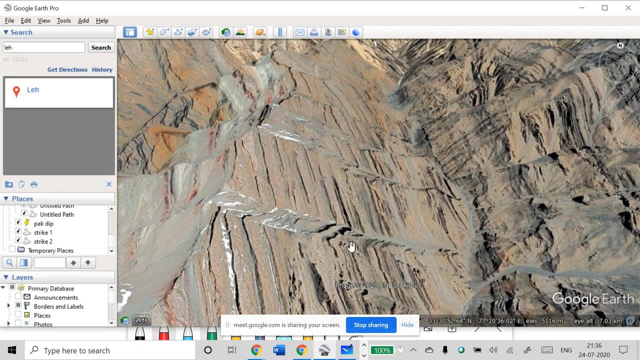 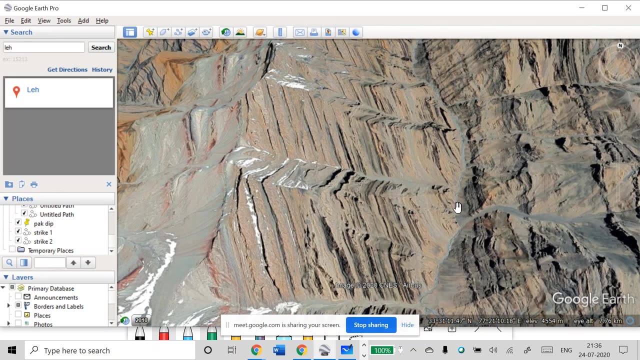 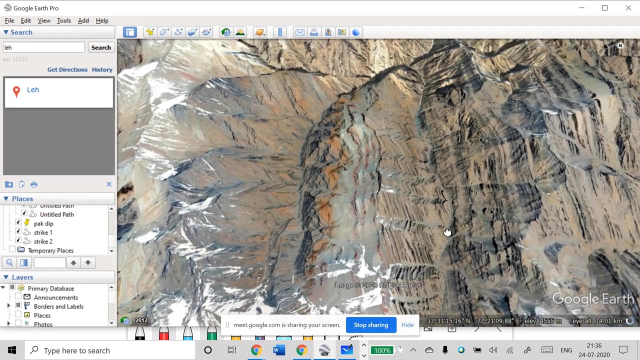 like that. so yeah, does anyone want to say anything? comment on those red red layers that you saw? no, okay, so let's see. so in this case, what you see is: so this is dipping the ancient oceanic plus exposure. okay, the ancient, so okay, yeah, so they would- which were exposed. so we are. 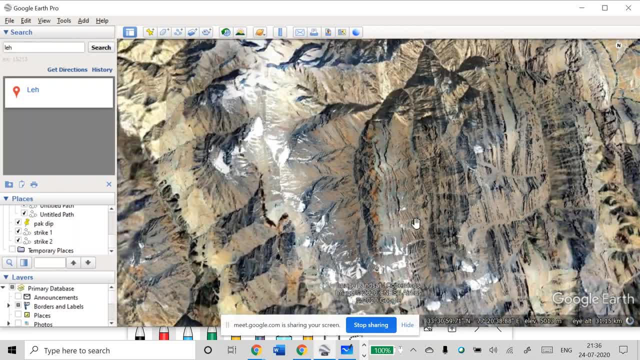 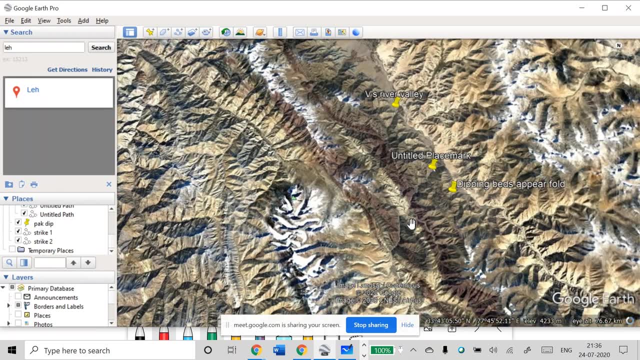 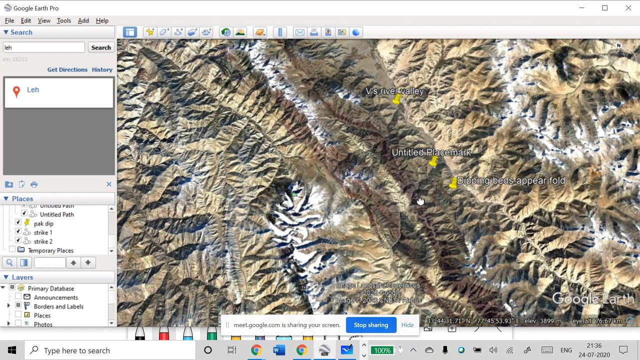 not very sure whether they are that ancient or not. seeing, these are continental. yeah, but you are correct, these are continental. uh, actually oceanic crust. if these are red, oh yeah, they could be, but at some point of time they would have been exposed for oxidation so that they could have been oxidized. so yeah, so that oxidation can happen only when. so if it was nhiều, 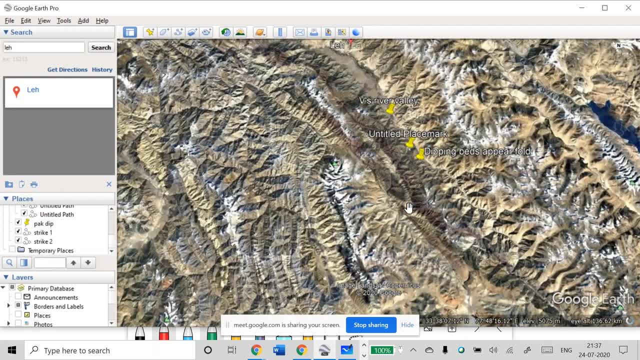 Yeah, if those there would be manyفيłagen, so yeah, so that oxidation can happen only when. so if it was baking, when? if that oxidation can happen only if it was baking, oxidation can happen only when. so if it were all oceanic. you will see, usually they are. 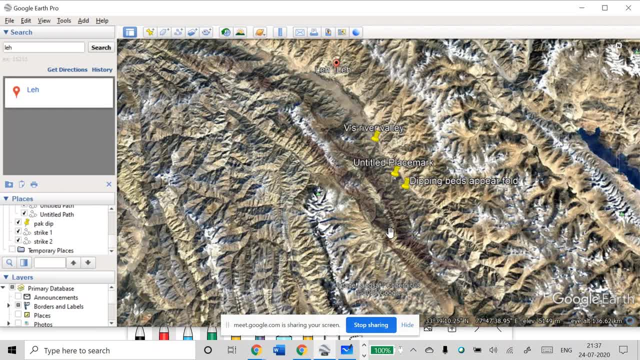 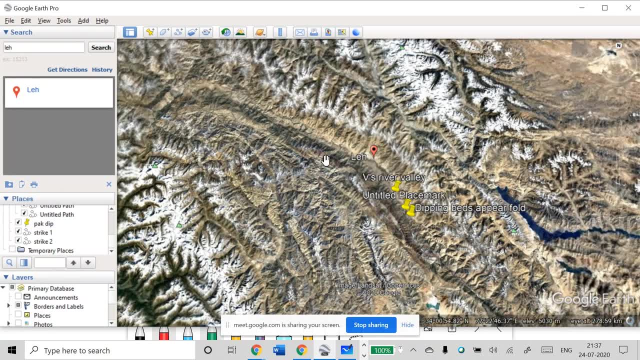 black in color, especially if you have any sedimentary layers. they will. if they will usually be black in color because of presence of organic matter, they are rarely red. so this is, I think we are very close to the Indus-Sankhya suture zone, so this is the plate boundary. 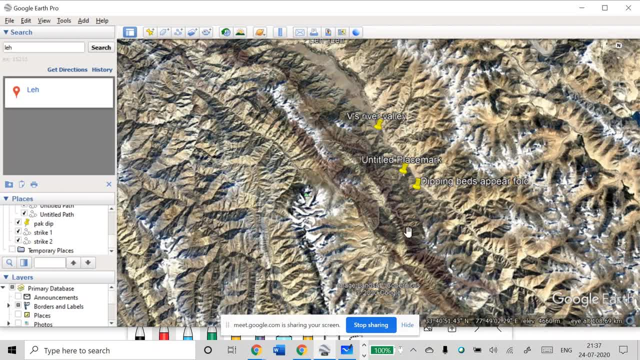 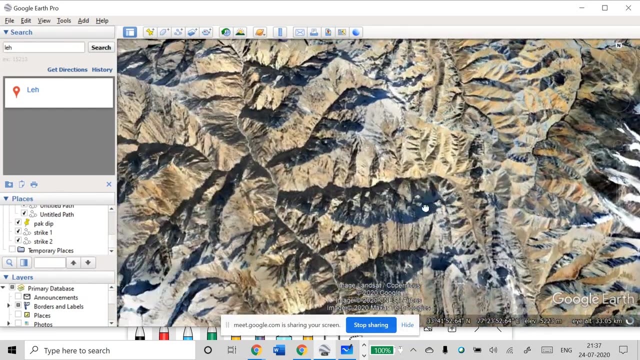 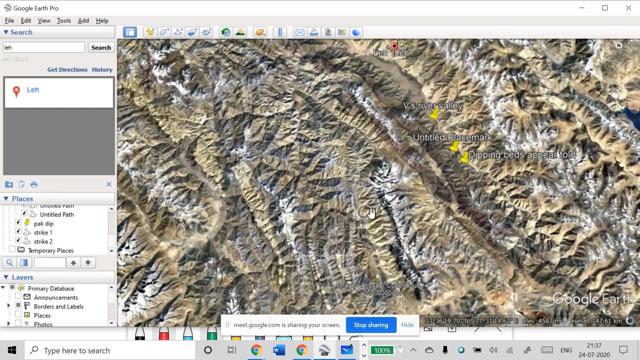 here and this is where the tethys ocean closed, and these red color is actually related to closing of tethys ocean, also because that resulted in exposure of the units that were there in this area. but, yeah, I think we again lost those. but yeah, the previous example, which 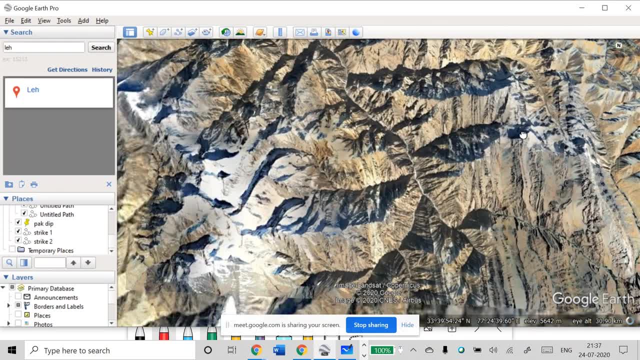 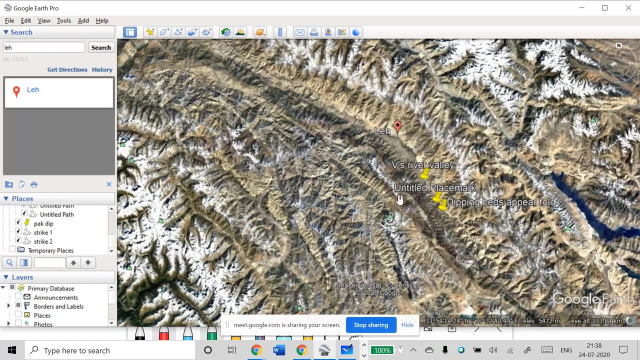 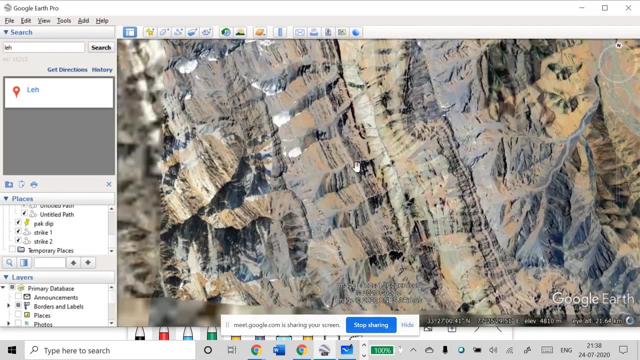 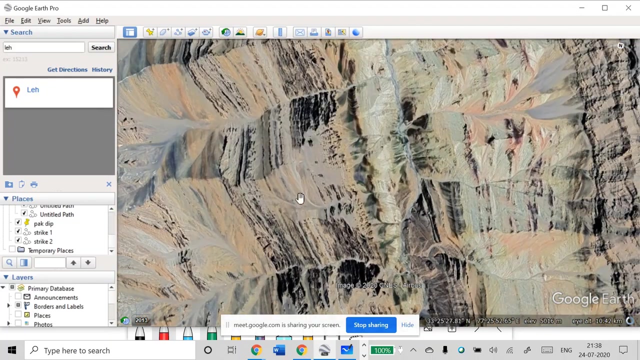 you saw. you now you can see that they were dipping in the same direction as the valley floor. This is the last example that we saw. yeah, these ones, you see, these are almost vertical. so another thing that, yeah, so, these V's if you see here, so this is a valley, this is a. 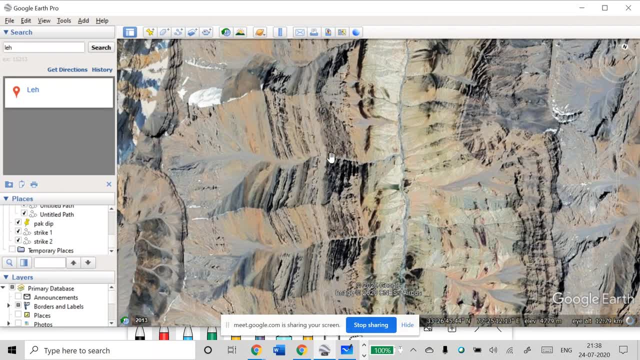 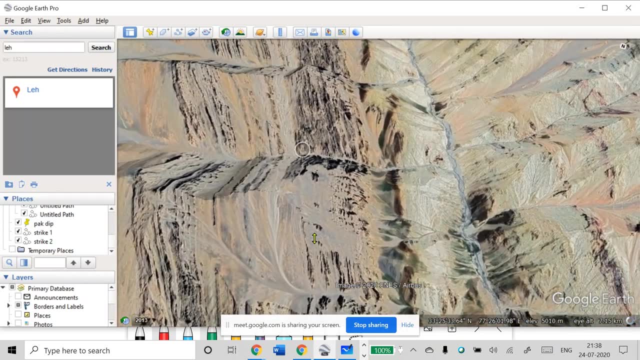 ridge. so in a valley ridge it will be opposite, but you can see they are slightly in this direction. they are pointing to direction of the tethys ocean, The slope, so you see this layer here. so if you draw a contour, how will it look? so it 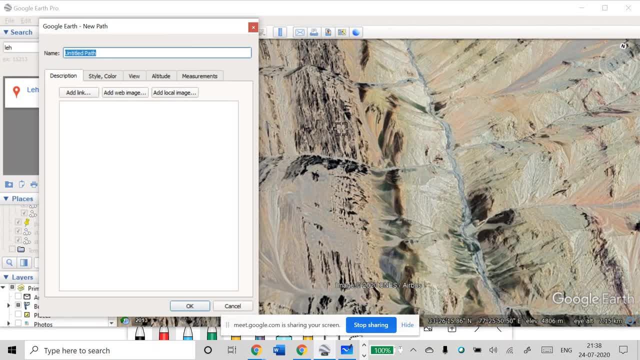 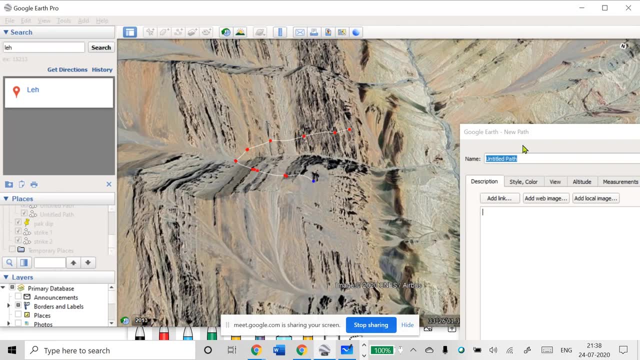 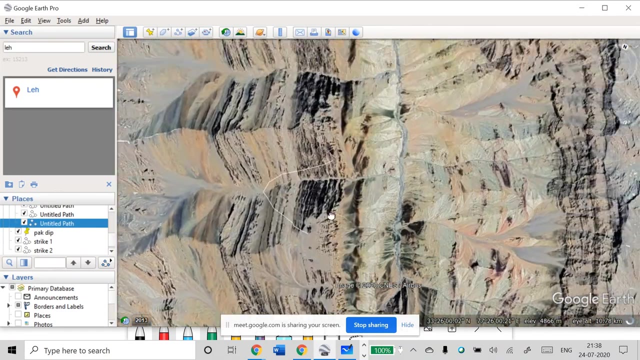 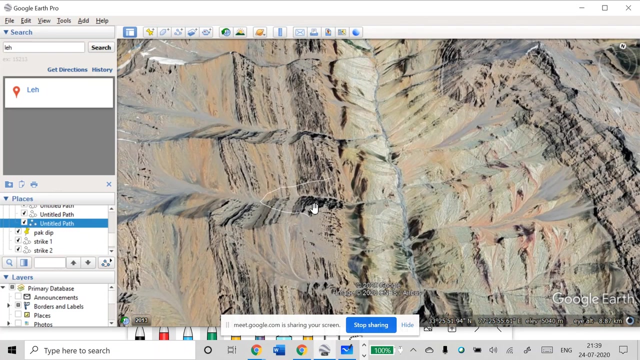 will look something like this. let me draw it. so the contour here, this valley contour, will look something like this: okay, So now, in this case, you see these V's are pointing opposite of this contour. V now, why? why is this? This is the case. in the previous case, we saw the beds were dipping opposite of valley slope. 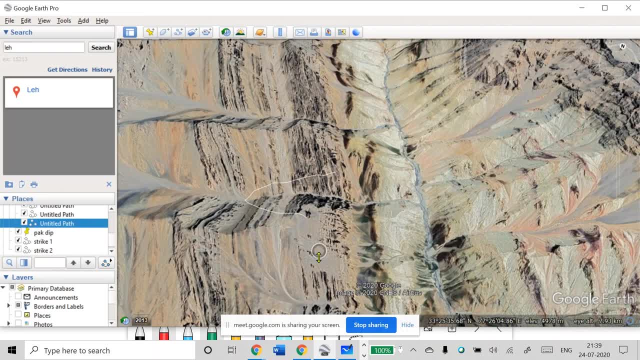 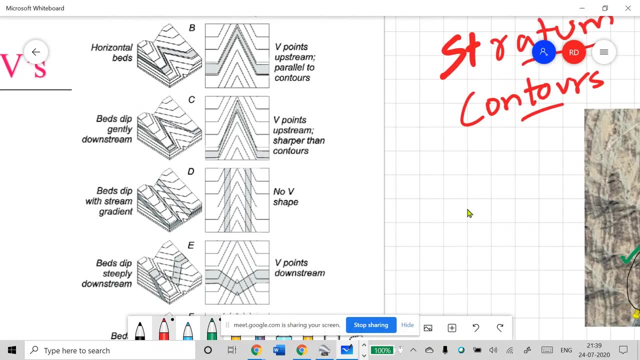 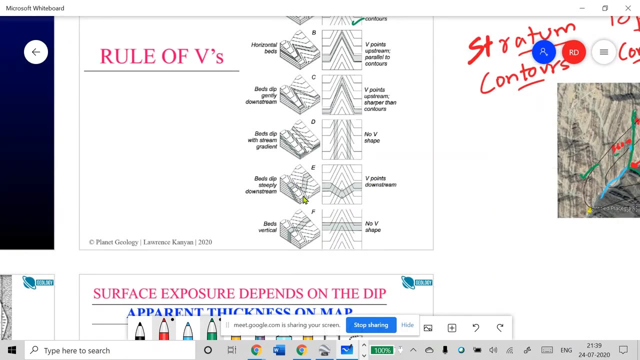 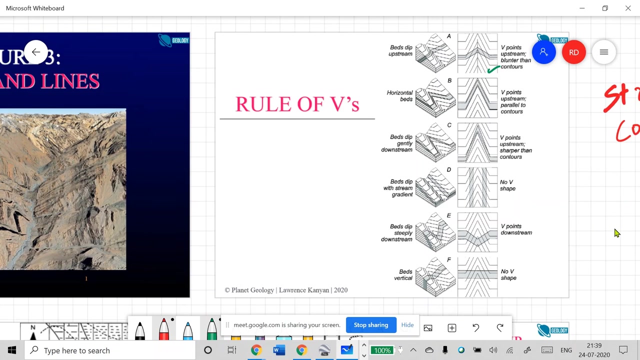 but in this case they are dipping in the same direction as valley slope. so which case is it? in this one, beds dip steeply downstream. so this is this case. so they are pointing in opposite direction and this is the image that you have here. So they will point in opposite direction of the V. so again, if you go here, so this V, this, 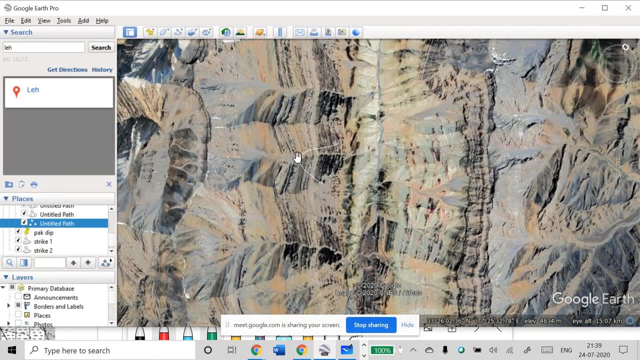 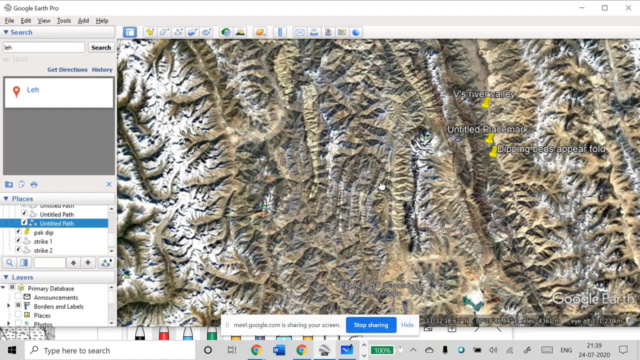 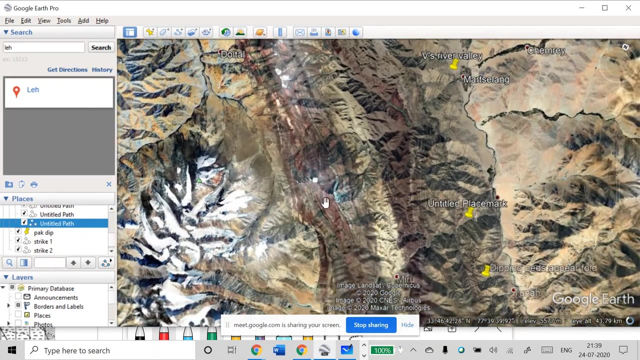 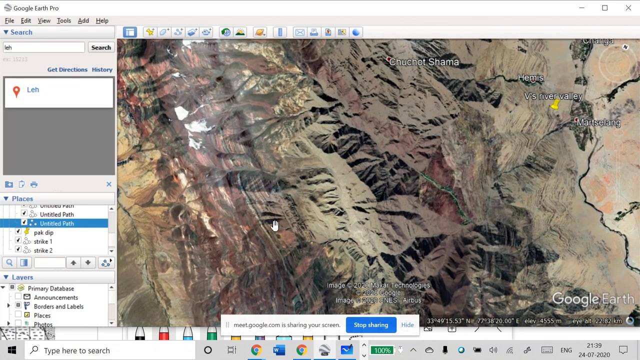 V is pointing towards east, whereas the contour V is pointing towards west, so they are in opposite direction. and there can be some examples of vertical beds also where you will not see. yeah, some examples. yeah, for example, here you see these layers. they appear almost straight, straight lines. 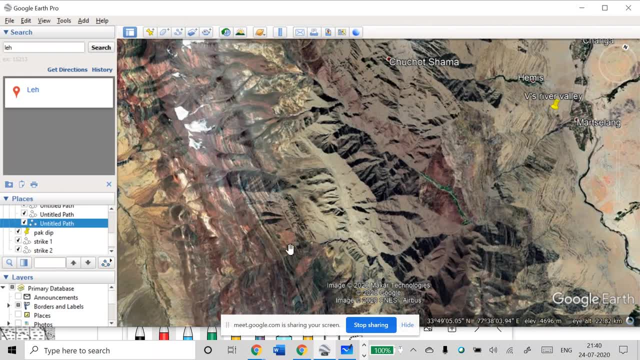 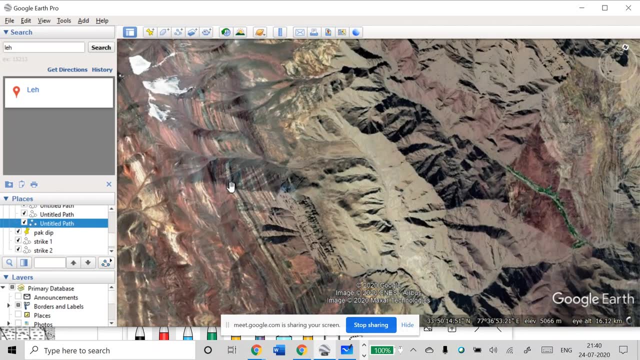 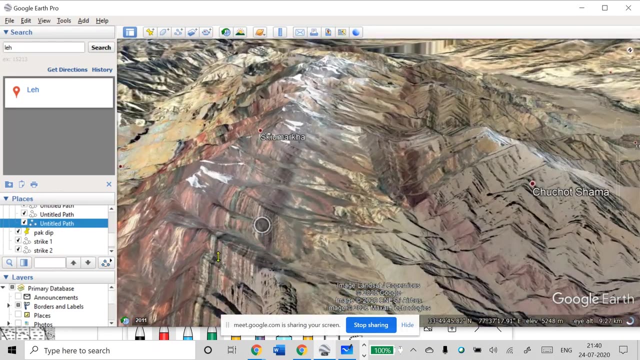 No V's. does it mean that there are no valleys in this area? you see these layers, this red layer, they are almost straight. does it mean that there are no valleys in this area? so if you don't believe me, you can see they are. actually. there is a lot of topography, even. 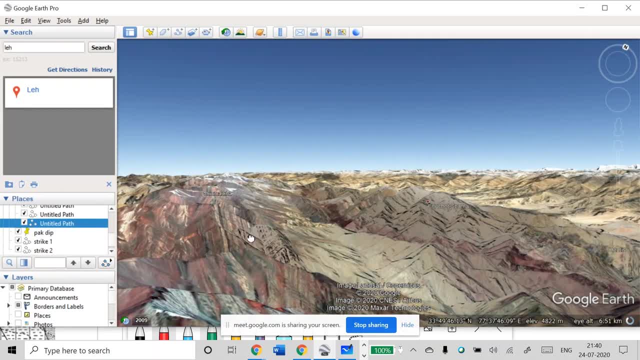 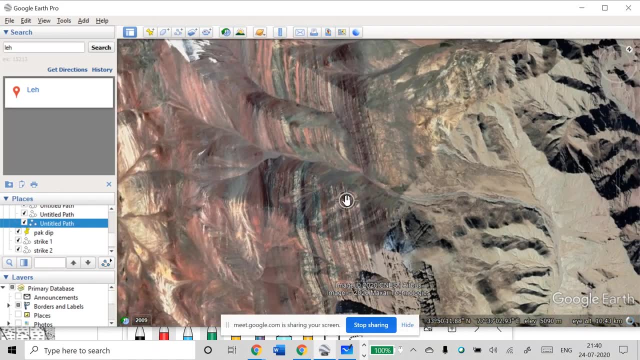 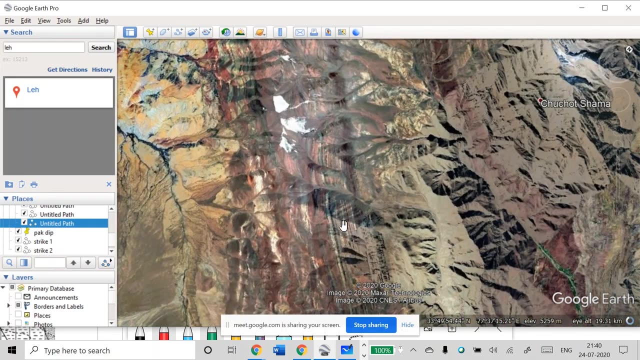 in this area. but you see the bed most vertical. so these beds are are vertical. so in case, if you have vertical beds they will not show any. So in case, if you have vertical beds they will not show any Topographic features. so I haven't said topographic features are still there, but expression will. 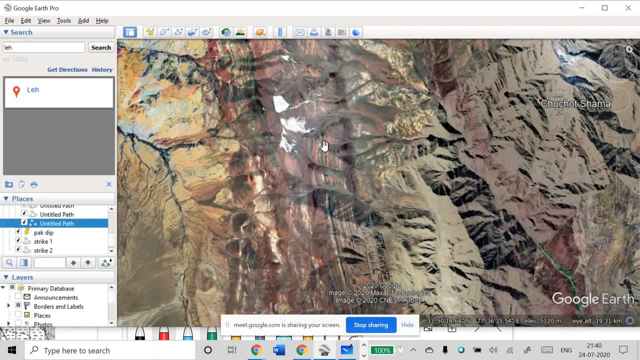 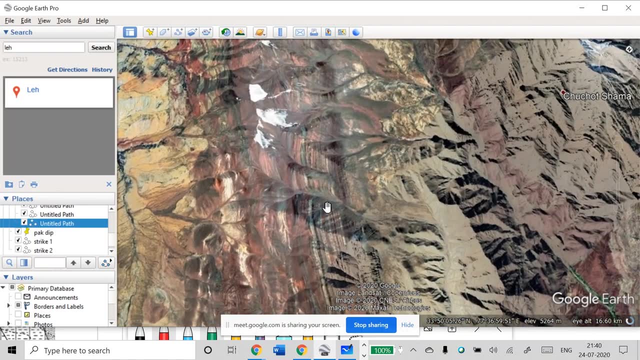 not be present in the outcrop patterns. so outcrop pattern will appear like straight lines, so there will be no V's. so you see again here. you use them from top they appear almost straight and you can confirm that there are actually valleys here and that the beds are. 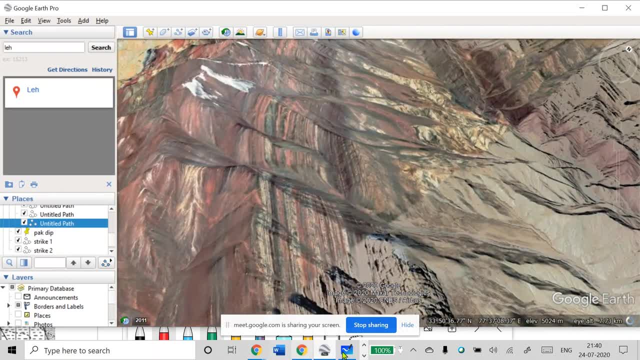 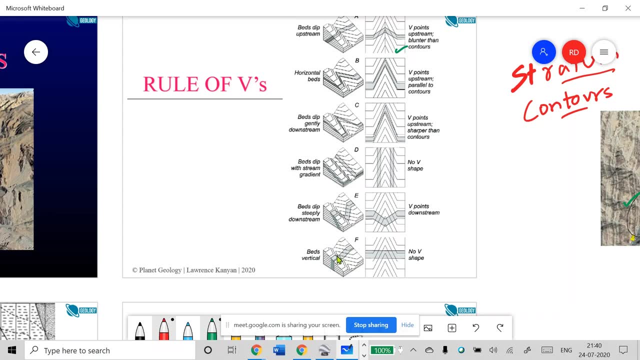 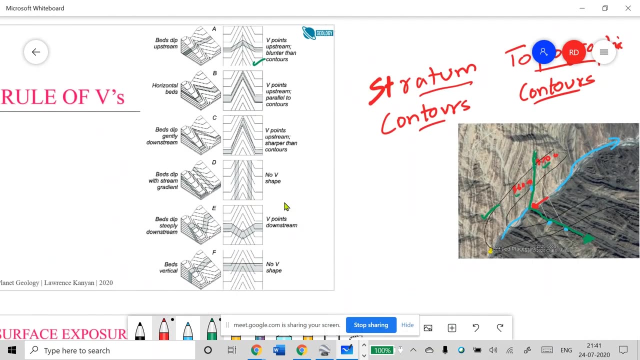 vertical, so you are not getting any V's. so this which case is this? you see this one F, So no V shape. So if the bed is vertical, so vertical beds will not show any V. So now we'll see. this is like. if you have to remember, you will forget these details. 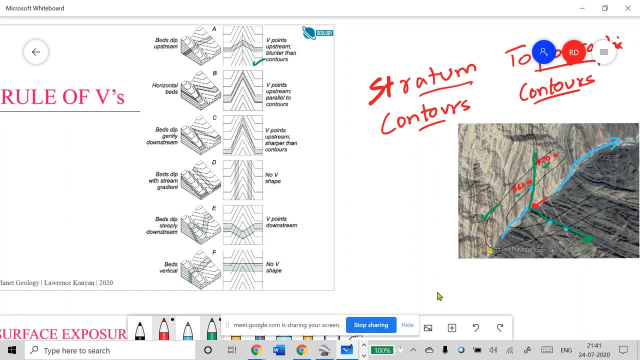 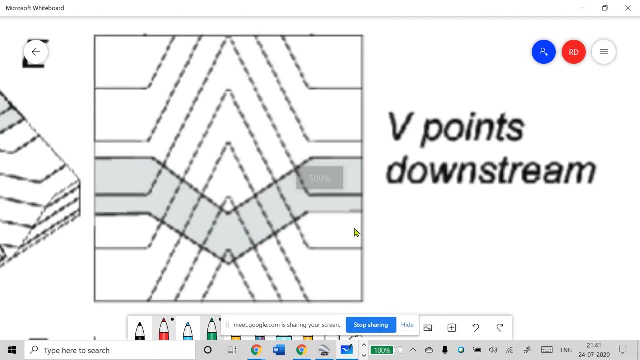 and things. but let's say now, if you have, if you are in exam and you have to solve any problem like this, let's say: consider this kind of problem. so if we zoom into it, so you know this is a valley. if someone gives you a ridge, it will be opposite. so in in a ridge. 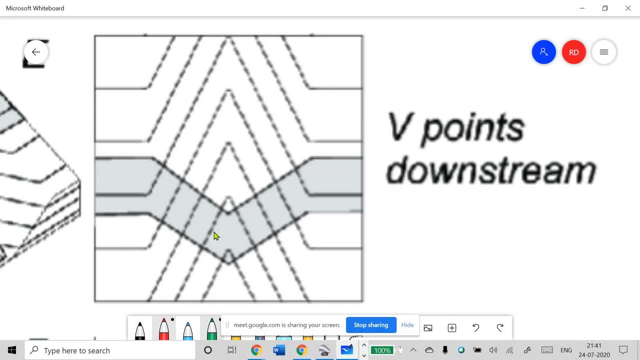 the V will point in the direction of degrees of elevation, Or downstream. V will point downstream in case of ridge, in case of valley, V will point upstream. so you know, here the upstream area the V is pointing. so these dotted contours you have already seen. so this is your up. 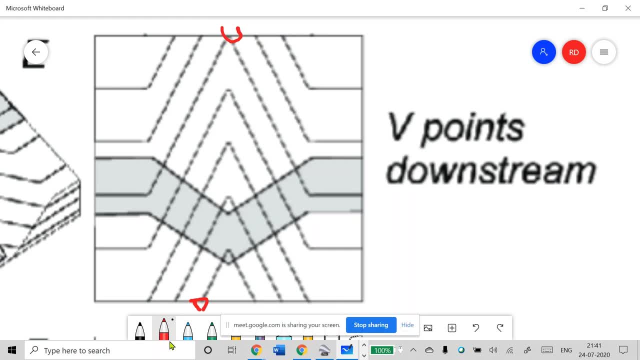 So this is upstream area, this is downstream area and yeah, so your stream is flowing in that Direction, So It is flowing in this direction and your V is pointing opposite. so you don't need to remember like where it should be pointing or it should. you know that this is higher. 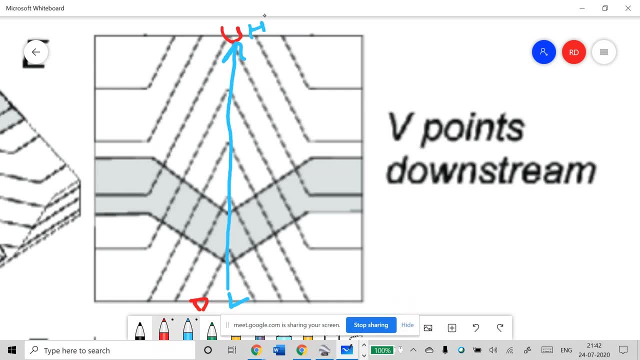 So this is. this should be lower and this should be higher. the stream should actually flow in this direction. Sorry, So it should not flow Here. So the stream is flowing in this direction, so this is lower. this is higher area. now you take any contour, let's say, let's consider this contour right here. 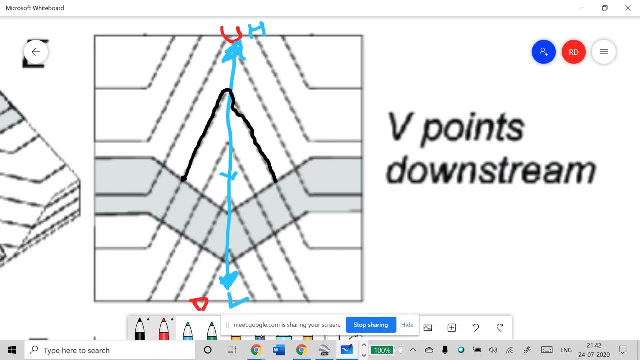 So, because it is contour, it has same elevation. so what will stratum contour look like? so, for stratum contour on this strata, so on this plane, we will consider this plane that you see here, this top surface, this contact- you need two points of equal elevation. where are 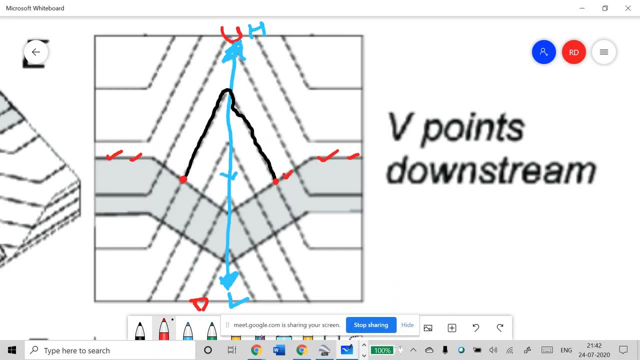 two points of equal elevation. first one is here and the second one is right here. so what you do is, if you draw this line, you will get a strike line or a stratum contour- okay, now on this same surface. so now you cannot go to this surface and draw another stratum contour. 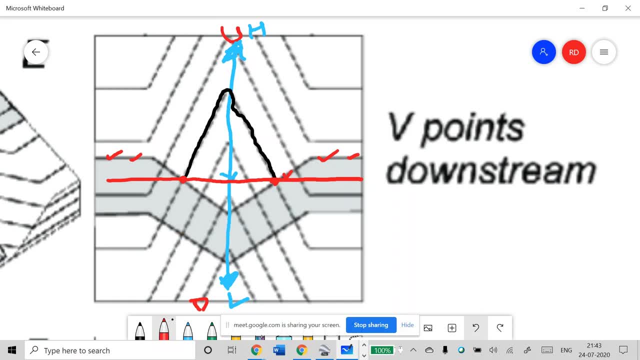 to compare. no, because you have to be on same surface. you draw anywhere. you can draw the second contour and let me draw it in different color. so here you, let's say, for example, you draw this one. Okay, now you have these contours, so you do. you saw in case of valley. so this V is pointing. 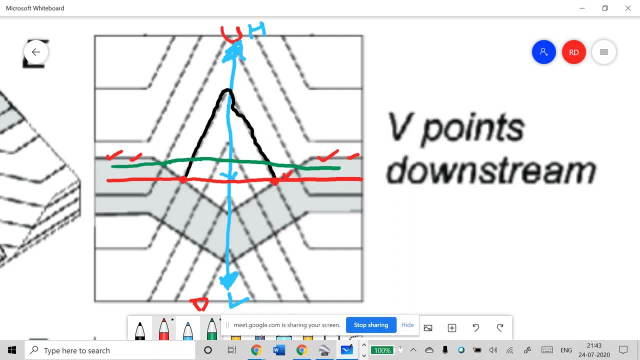 above. so this is in higher area. so the green. so which of these have will have higher elevation value? green or red green? so green will have higher elevation. so which side? with which side should the beds dip Down this side? Okay, Yeah, so they are dipping downward side, so they should be dipping. this is your dip direction. 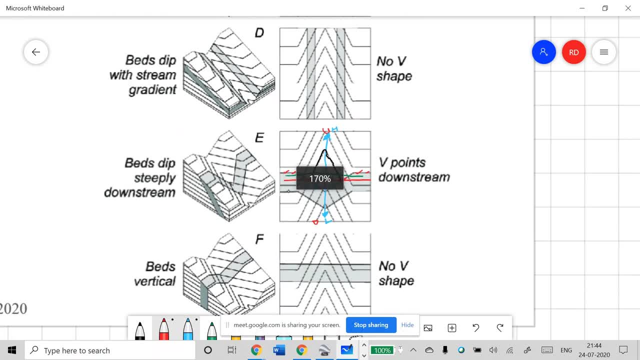 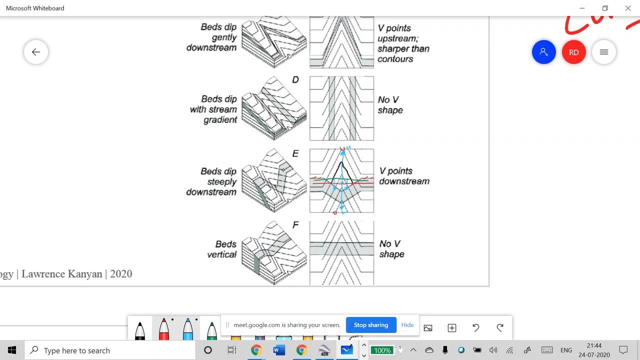 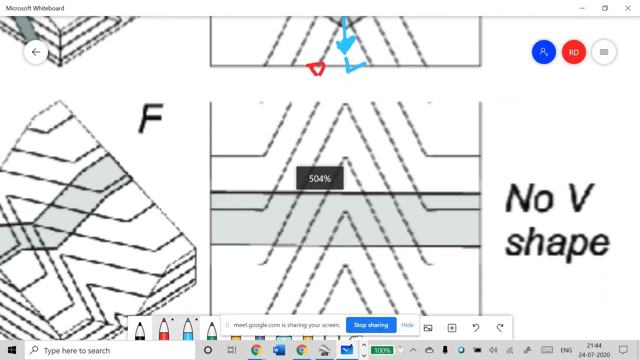 of the beds. that is in the same direction. that is downstream, so stream is flowing in the same direction, beds are dipping in the same direction. so that is why, you see, this is the case. we've already proved it. So, for any case, you can do. it will be difficult to do it for this case, but you can see how. 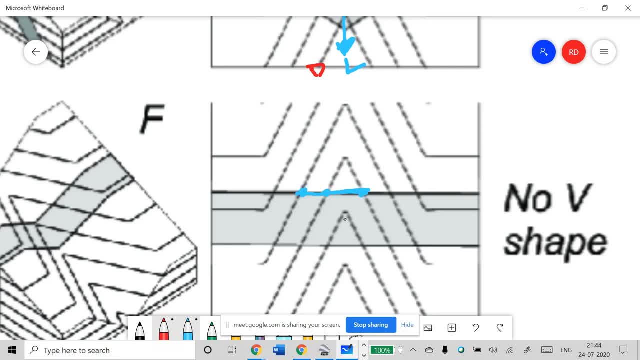 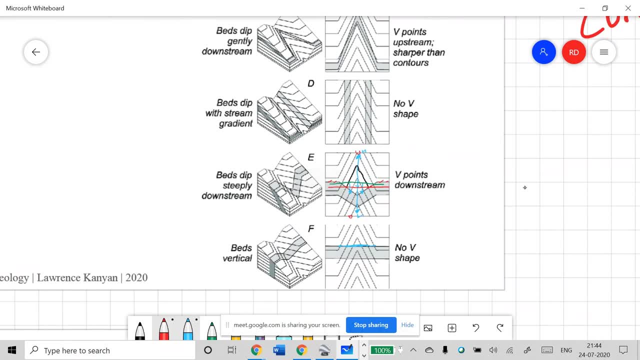 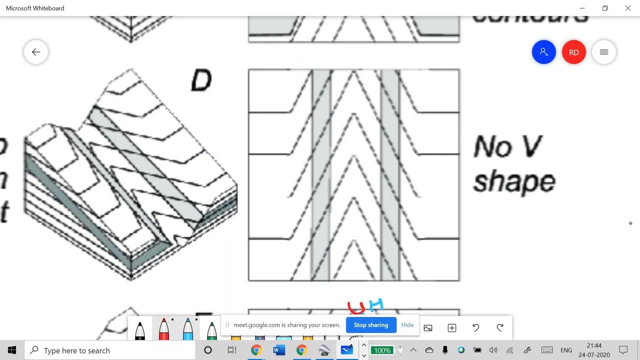 this is First contour, this is second, so all the contours are stacked at one place. it means it is vertical bed, so there is no horizontal movement, all in this case, let's say it is exactly the same, so stream. so if they are like this, so these are not forming any V pattern. the both the 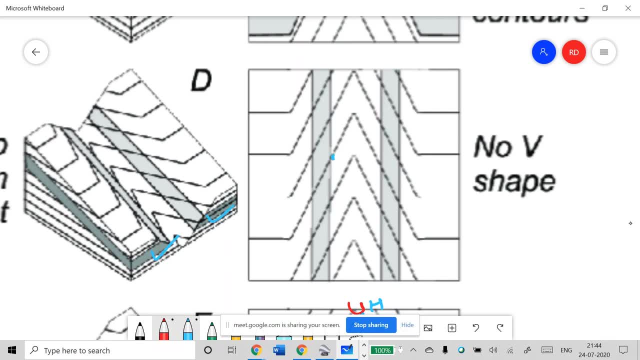 sides. it is parallel in this side and this side. so you see, this is your, this will be your one contour and this will be second contour. And what will you? how will you determine valley slope? valley slope will be? if you have seen so first, you need will later on see how you can actually determine slope also. so for 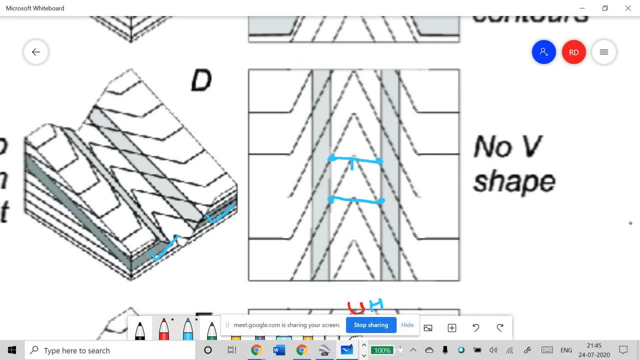 determining slope, you need horizontal distance. it is just like if you have stairs your home and these stairs go something like this: so you go vertical and you go horizontal and this is your slope. so same thing will happen here. so this is your horizontal distance and let's say this contour that you see here. this is 100 meter contour and let's say this. 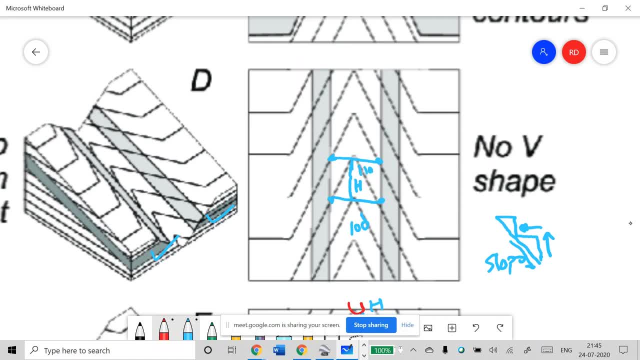 one that you see on top is 110 meter contour. so in this case, this H is the horizontal distance and your vertical distance will be the difference between these two values: 110 and 100. so this is 10 meters. so this is how you calculate slope. so if you do this for these, you see. 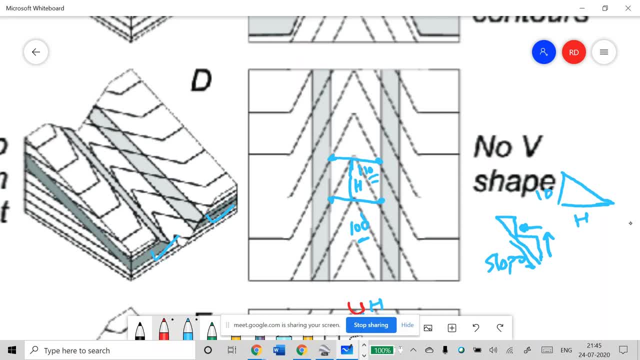 the slope for for the valley as well as for these stratum contours. if you determine slope from stratum contours it will come out to be the same. But you can remember like if they are parallel. you see this distance here, but in valley floor horizontal distance and this distance here they are both same, so it has to be same slope. 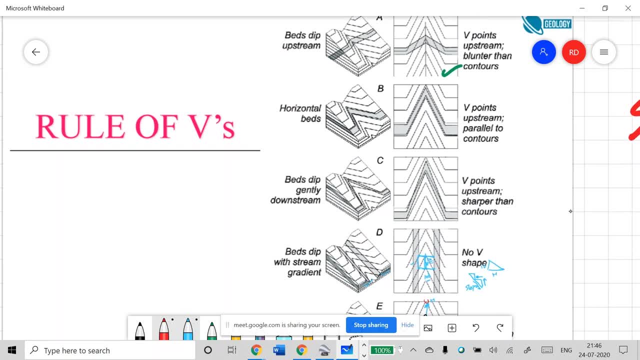 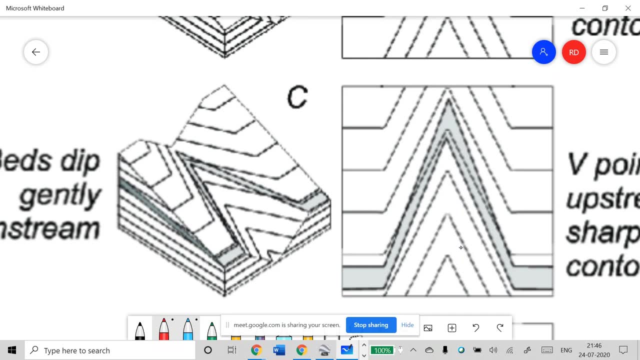 similarly you can see now in this case beds are dipping, but they are dipping gently downstream, so dip is very gentle. it means you will cover a lot of horizontal distance. so you see first stratum contour. if you look, it will. so for this pattern it will actually look somewhat. 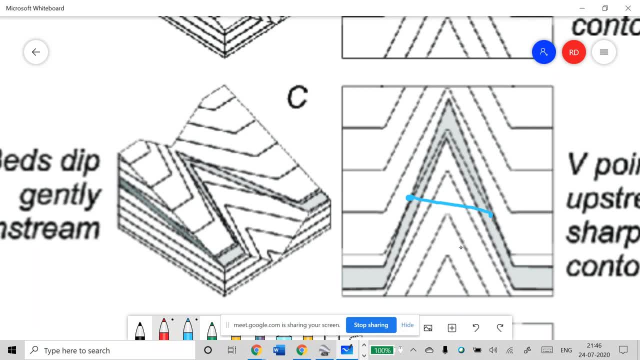 like this. For the second one, it's actually very difficult to determine because it is not actually this, this surface that we are using. so we are somewhere here. so let me draw this first, because it is very confusing. so your outcrop is something like this: so actually we are not even intersecting. 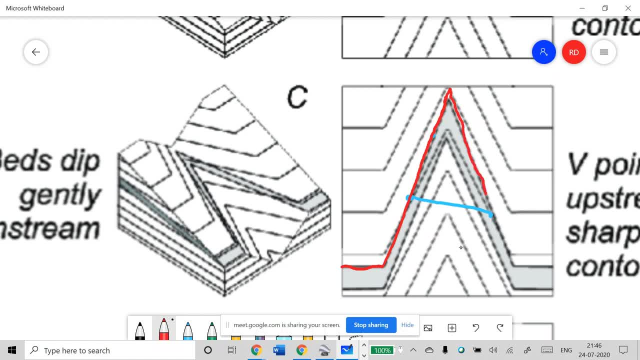 another. but let me extend it a little so that you can see. So it is not even Even intersecting another contour. but let's say: first consider this contour. so let's just assume that this contour is 100 meter. okay now, in a valley we always points upstream. 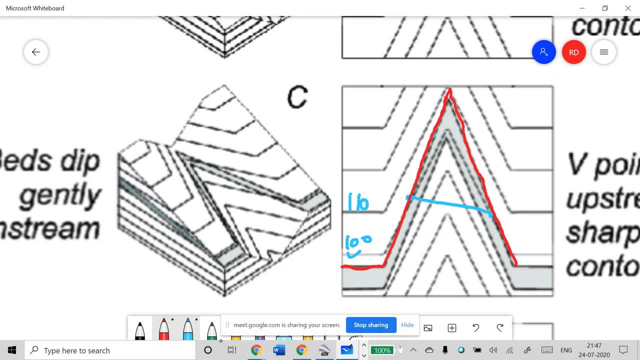 okay, so this has to be, let's say, just for example, 110. you can take it 200, whatever you want. so the second is: so where will you see? so 100? so now let's say it intersects. so here it is not intersecting, but let's say it intersects here. so this 110, so this will be 110, this is. 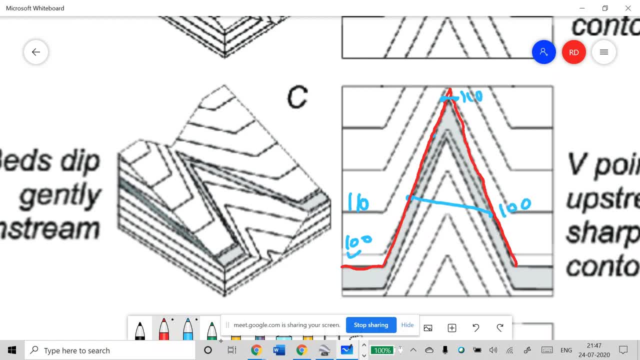 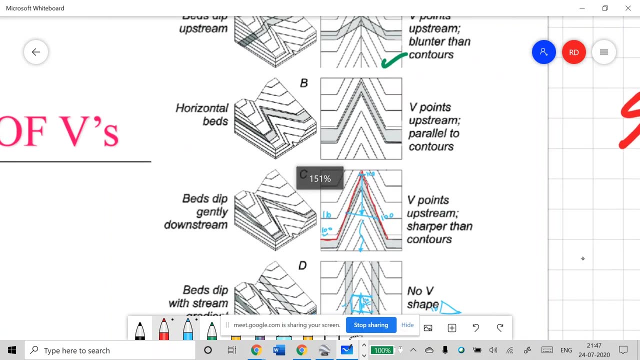 100.. All right, so where should be? where should this be? dipping beds should be dipping in this direction, so these are also dipping downstream, because stream will flow opposite to the direction in which you have these these are pointing. now, how do you know? these are gently dipping. 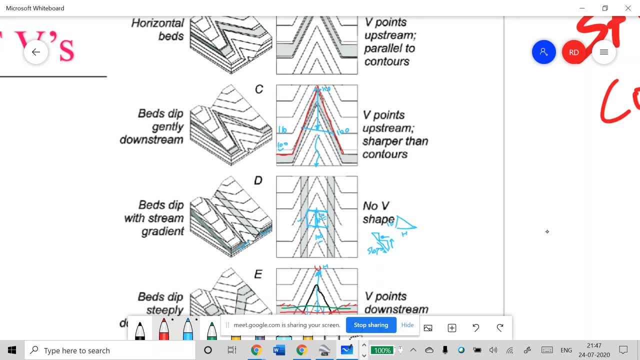 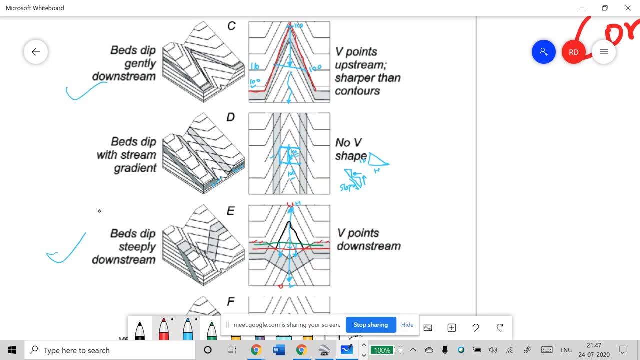 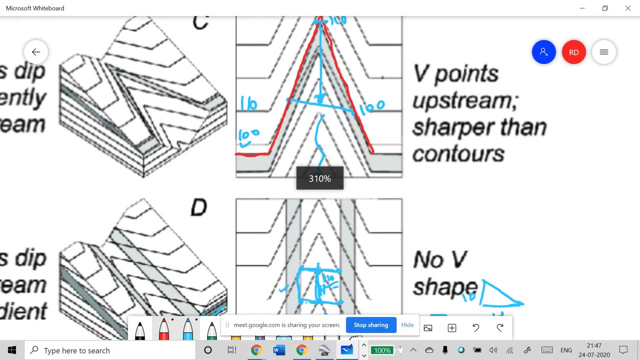 so you see these beds dip with stream gradient. they are parallel. so you see all these are dipping downstream, especially these two cases. but difference is these are here. the slope is less than the valley slope. Okay, How will you know that it is less than the valley slope? because you see horizontal, vertical. 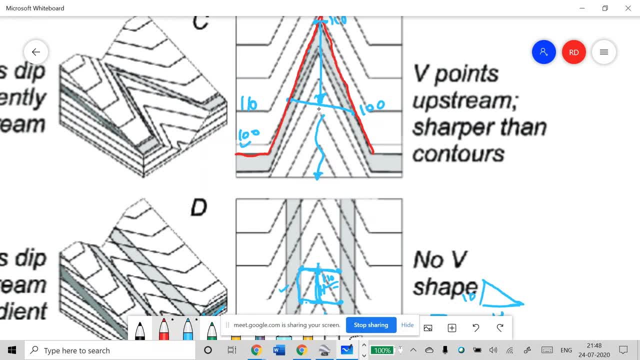 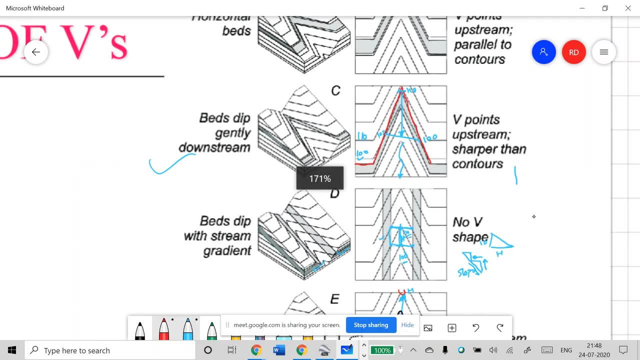 distance is 10 meters. between this contour you see 100 meter, and so this is 100 and this is 110. so vertical distance is 10 kilometer or, sorry, 10 meters, and slope will depend on horizontal distance, so if horizontal distance is more or horizontal distance is less so. 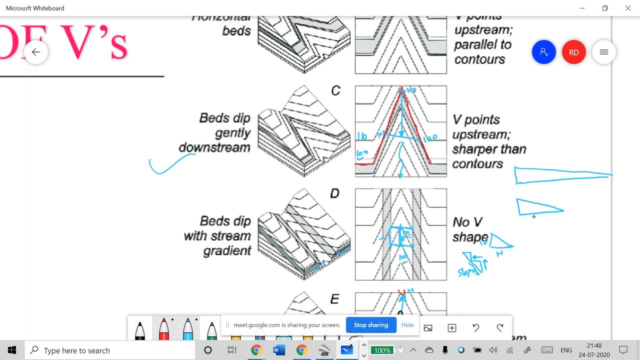 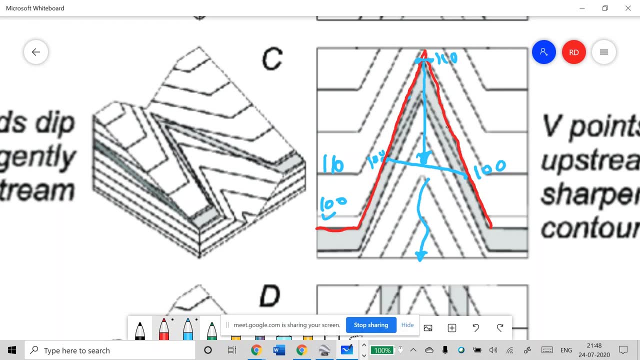 if horizontal distance is more, you have gentle, and if it is otherwise, you will have steep. so in this case, you see, horizontal distance is large And that is why Your dip is less, and horizontal distance if you calculate between these two beds. so for stream it is less. see for stream, horizontal distance. let me call h stream and let me call 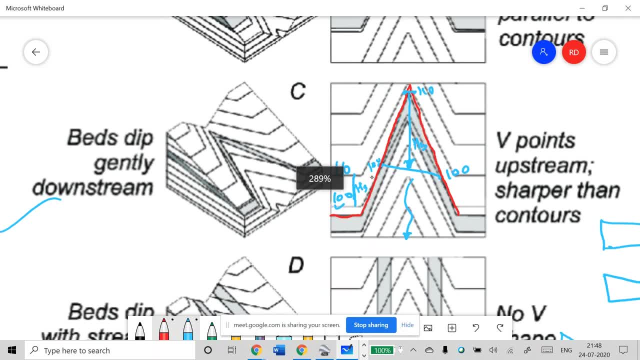 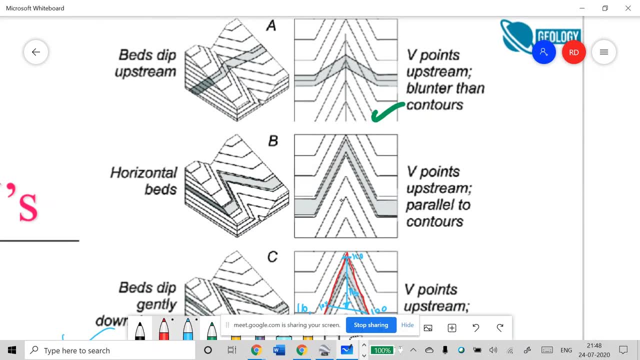 this h bed. so beds, it is more. so beds have to be more gently dipping. Now for horizontal beds. it is very easy to remember. I don't think you need, because if beds are horizontal, that is the definition of when you define contour, itself so topographic. 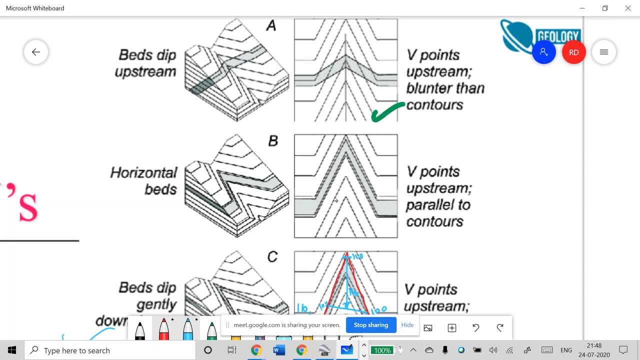 contour Is when you cut topography with a horizontal plane, you will get a topographic contour. they have equal elevation everywhere. so if you, if your bed itself is horizontal, it should be parallel to a topographic contour. so in case of horizontal beds, these will be parallel. 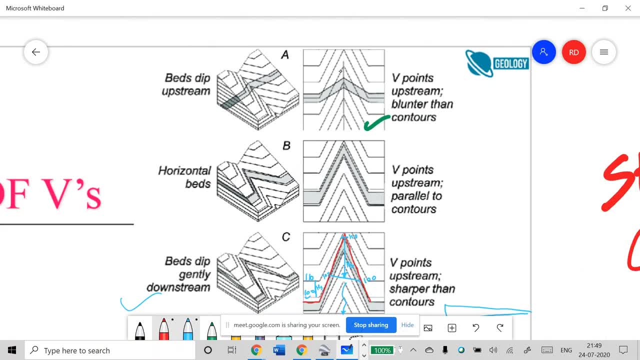 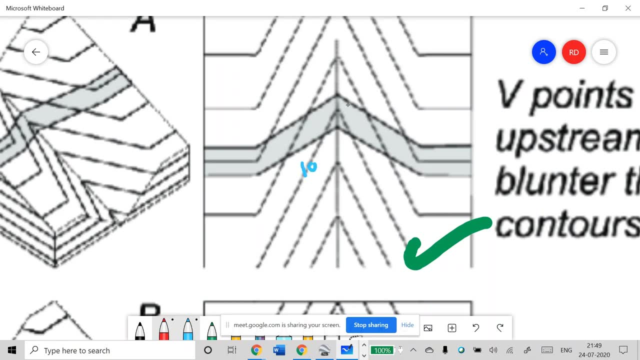 safe. these will have same thing. And finally, this: we had already seen previously how you can actually determine it. so what you see here. so again, v is pointing upstream, so this has to be 100, this has to be 110. stream is flowing in this direction. 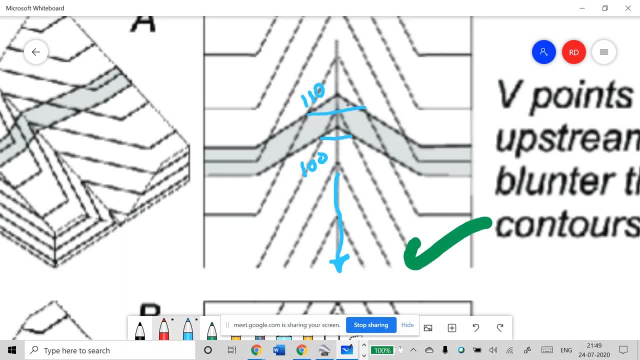 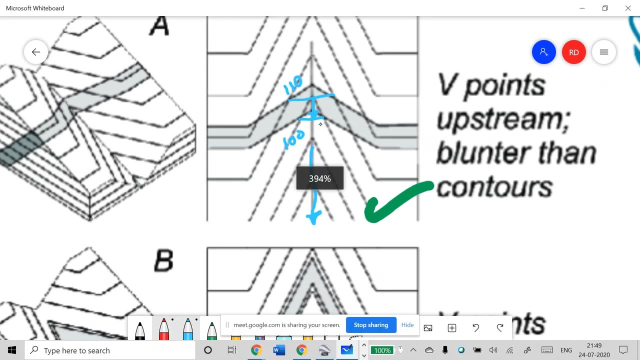 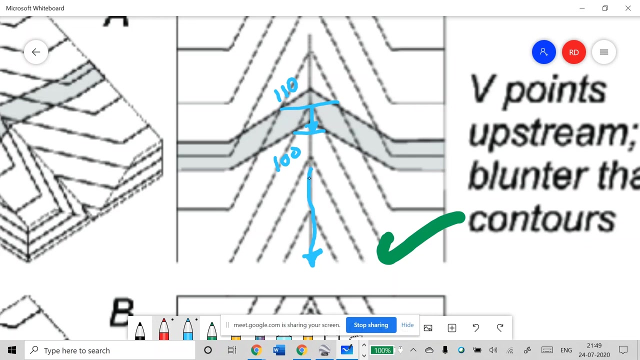 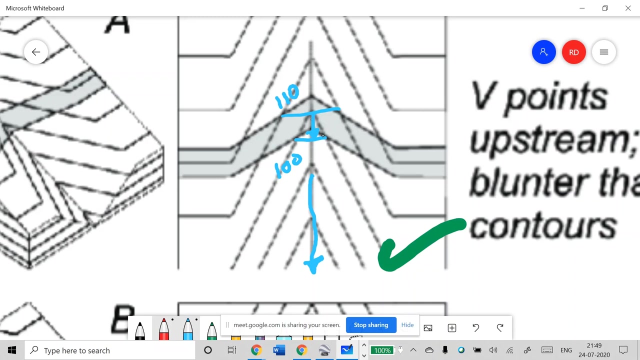 And so this again is 100, 110, so so the dip should be: oh sorry, I think I did something wrong. We will point upstream: the stream is flowing in this direction, Oh okay. so yeah, I was telling you guys not to make that mistake and I myself made that. 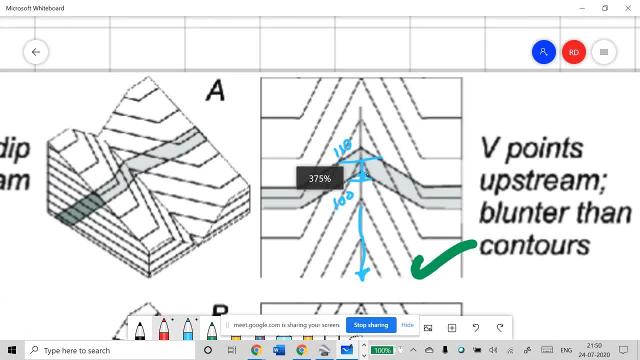 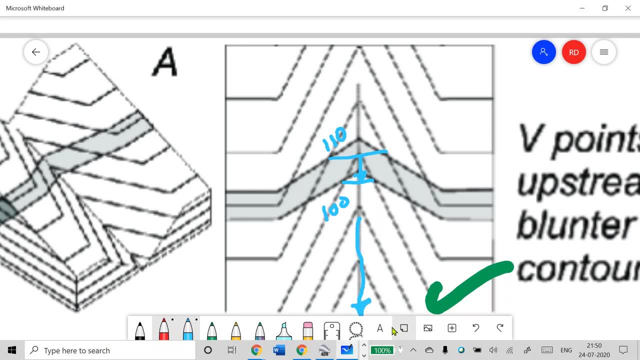 mistake. can you, can anyone tell me what we have to use? yeah, so we have to use same contact. okay, so the one that I drew here. this is incorrect. I was telling you guys not to make this mistake and I myself making this mistake, so you have to use the same element right in different. 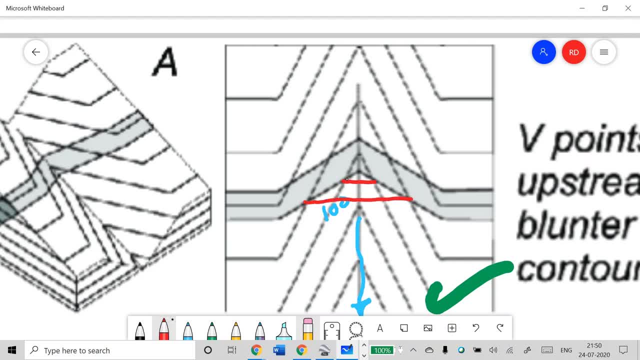 color. So you use this one here and then you use this one right here. now you will see that this we saw was 100 and if this is 100, then this should be the second one. if you are assuming this to be 100, then this should be 90, because upstream, when you are going, your these v's. 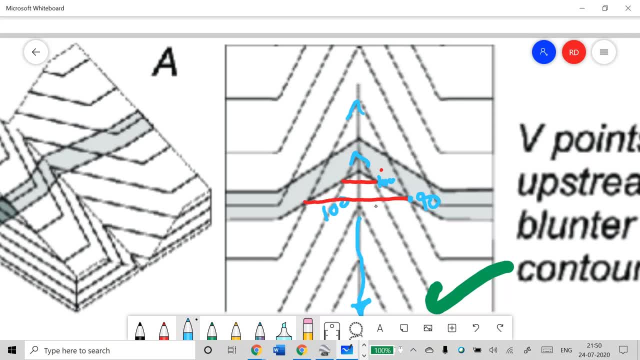 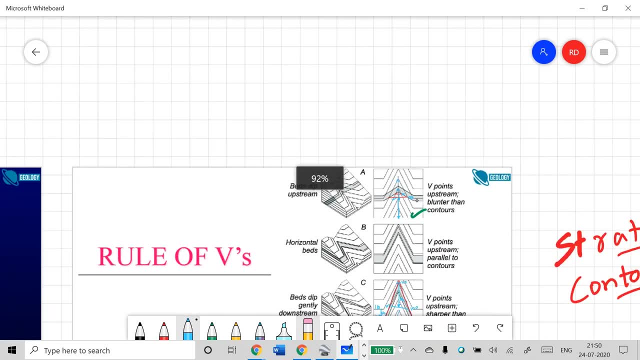 are always pointing towards areas of higher elevation. so you are coming opposite of v. so you are going from 100 to 90, so your dip has to be in this direction. so now, anytime you get this question, Even if you don't remember, Remember these things: what is happening, in what case. so what you do is you draw any contours. 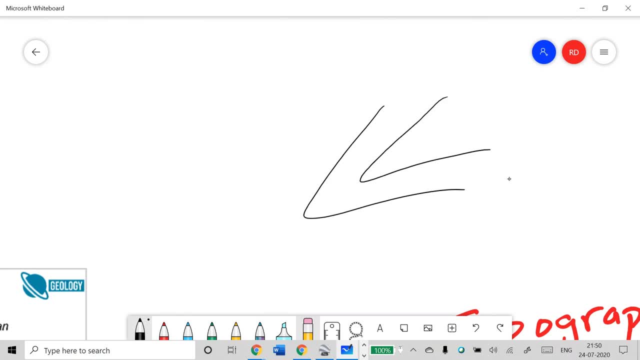 let's say this contour v has to point in opposite direction. just label one of them as 100 and another one as 90, and then you draw any bed like this. so whatever pattern is in the examination is given to you, maybe something like this, or you get something which is in the same. 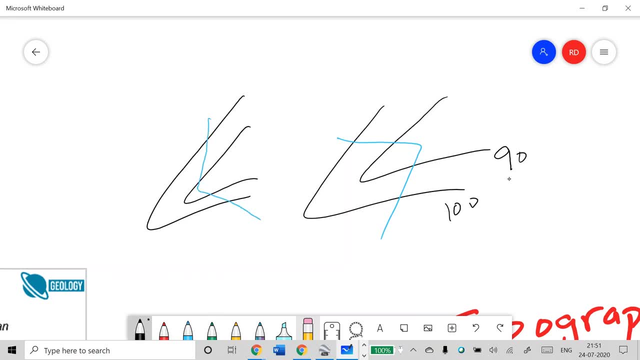 direction like this. So what you can do is very easily, very quickly, you can just draw these two figures to remember and then you can again label them 190, just like here, and then you draw these contours, for example: here you are going. So this, this is now same bed like this, so this is. these are actually very rough there. 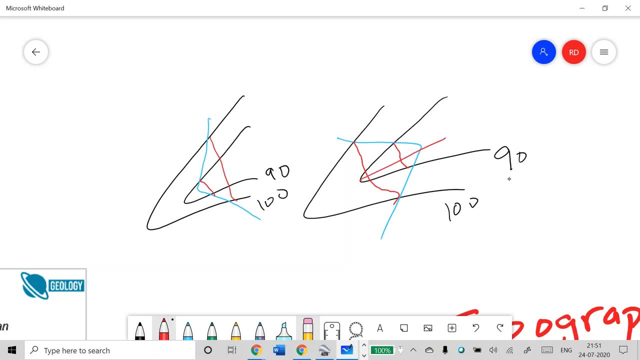 these strike lines should be parallel. now this is dipping from 100 in this direction and this is dipping from again. so this is 100 and this is 90 and this should be dipping these beds. So this bed should be dipping in this direction. Okay, 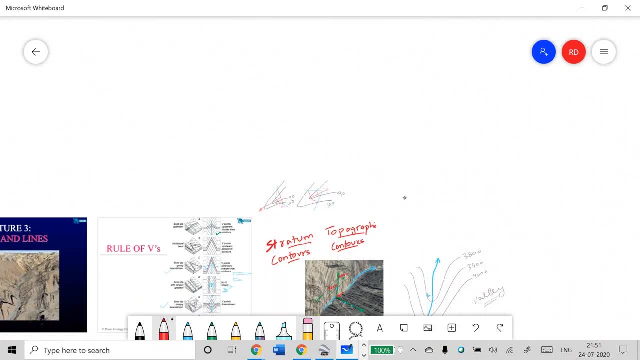 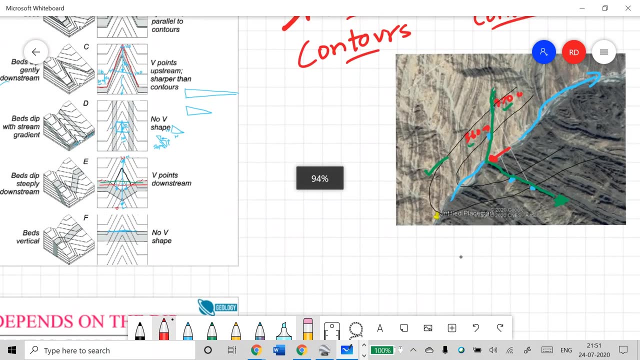 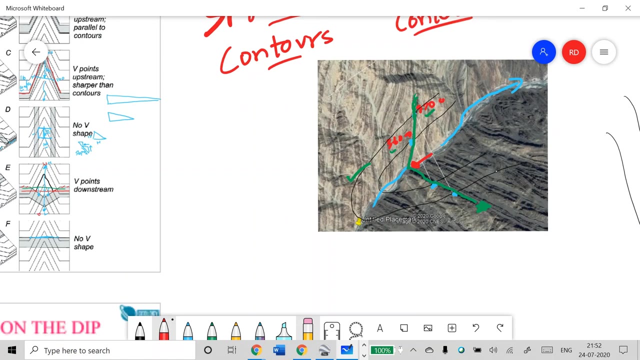 so this is how very easily you can solve these type of questions and now you understand. you also understand how you can actually, and you how you can. what is the difference between this strata and topographic contours? so topographic contours, these are actually values of equal elevation. and then, if you want, if, 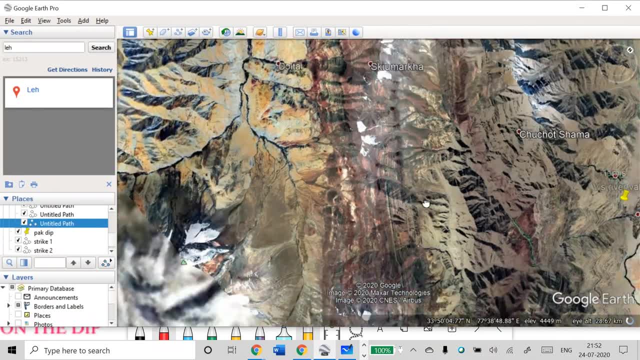 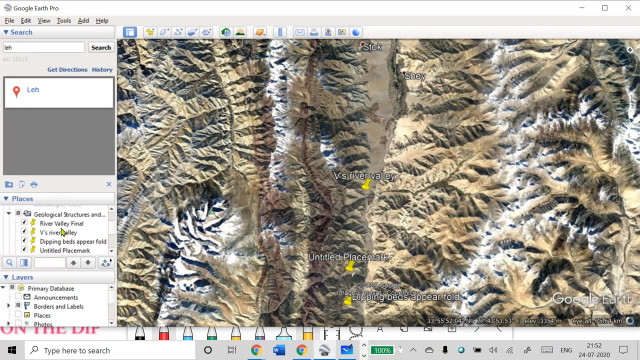 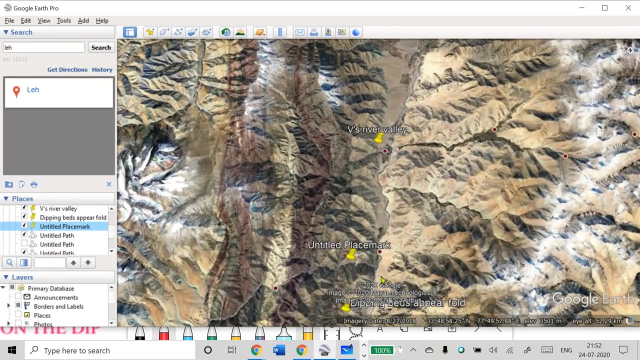 you have, especially if you are not preparing, you're still in undergrad graduation and you just want to learn more things, then you can actually go here and see- there are a lot of examples in this area which you will find- and you can go here and you can actually draw that plane also. you see what you can do. 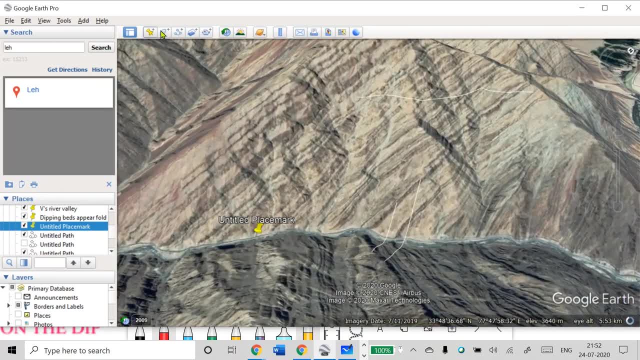 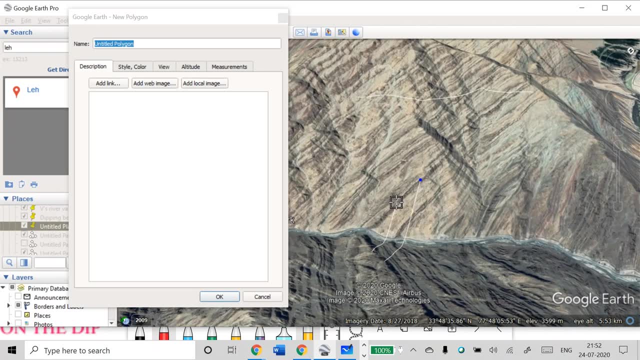 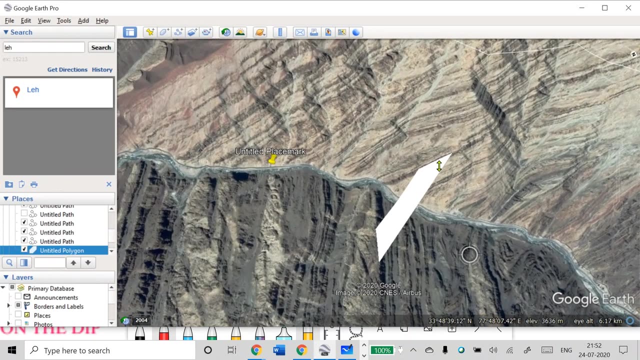 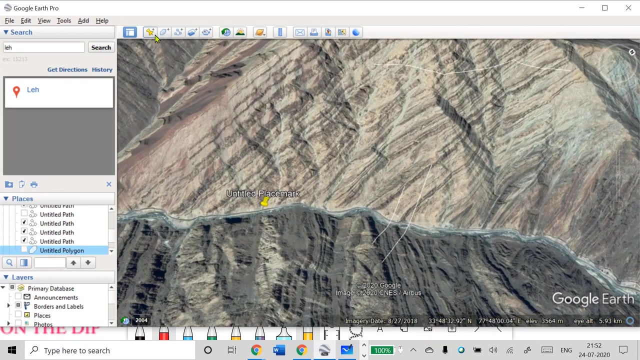 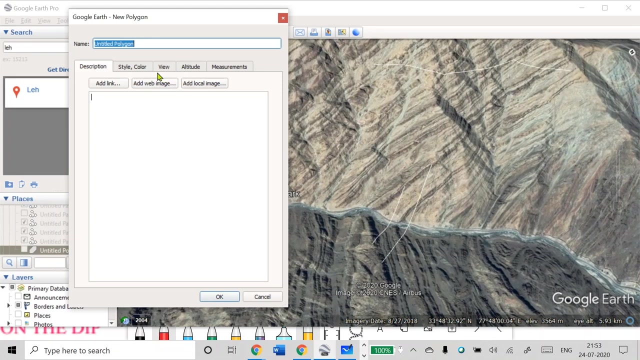 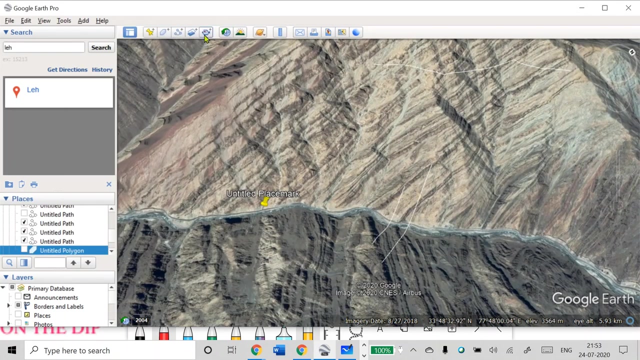 here is that you can add a polygon also and it will give you a plane, for example. you just join these points. so now it has not shown in 3d, but not this one. actually not polygon, let's. i think it has to be done with measurements. 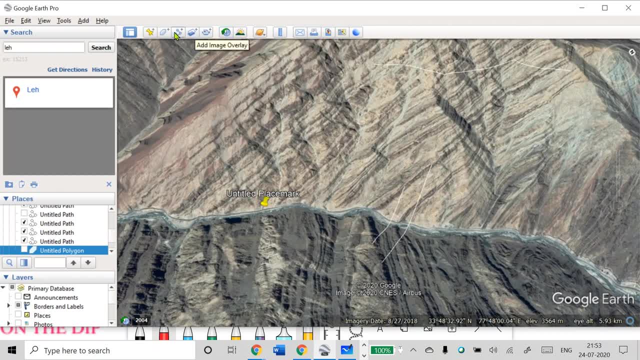 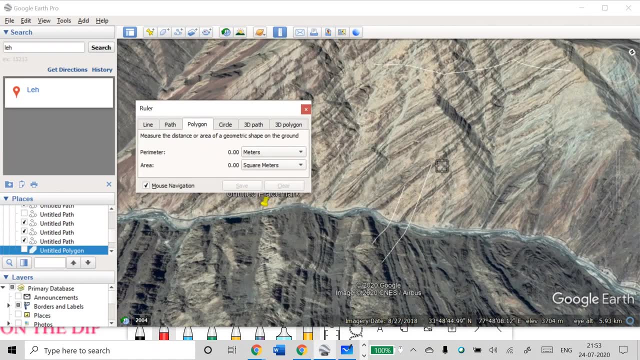 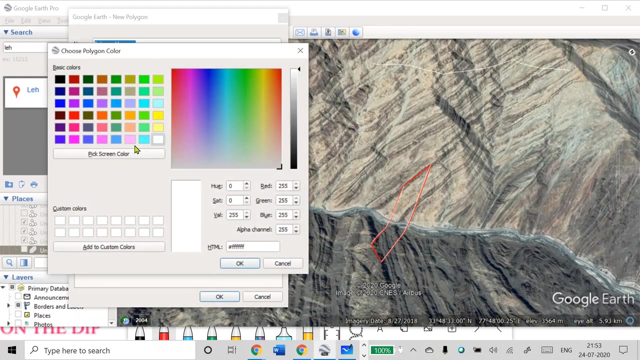 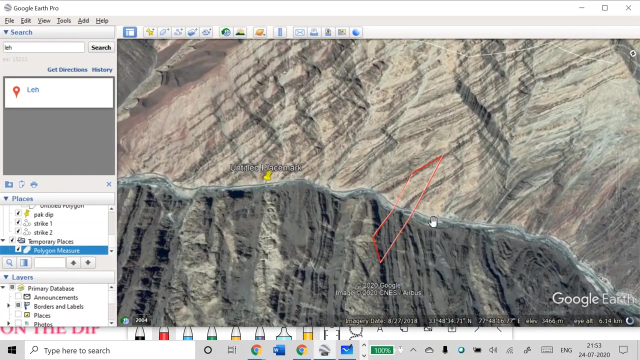 so you can actually uh, put, you can actually put a polygon here, show ruler. okay, yeah, polygon, and this one, you go, let's. no, it is also so. okay, i'll maybe later on share something with you guys, which will be better, but you see this, a plane will a. 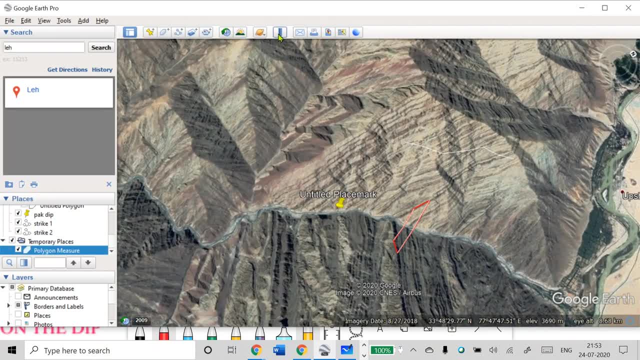 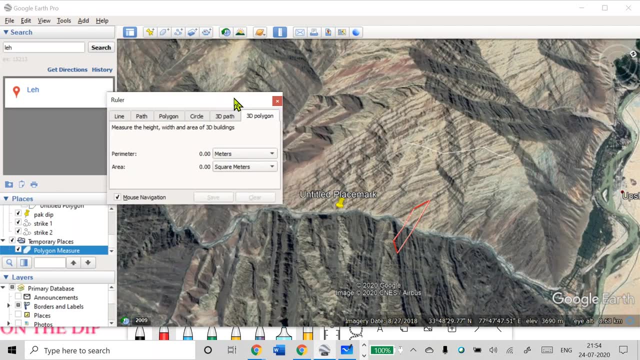 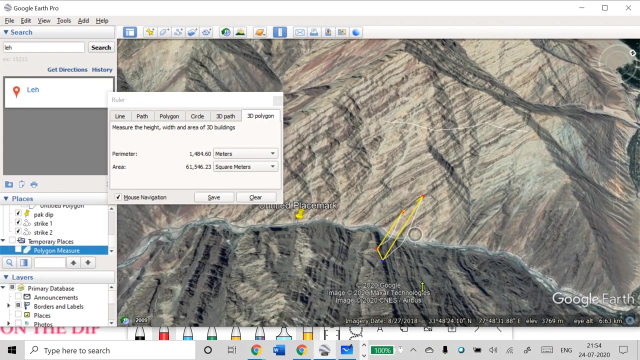 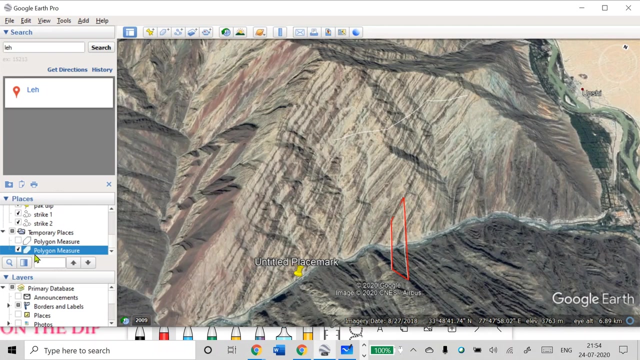 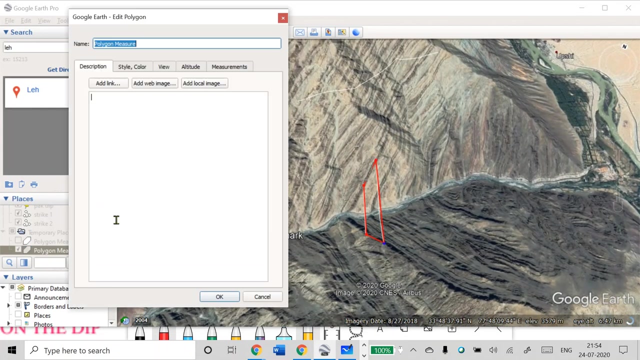 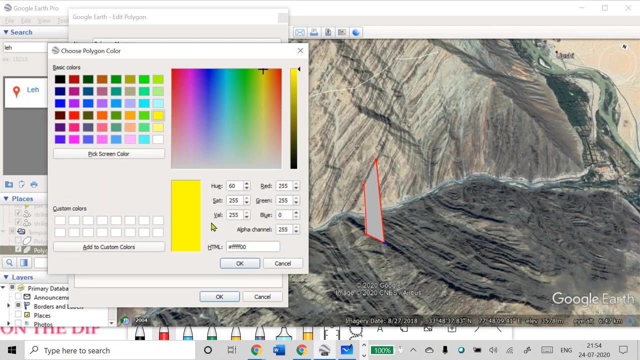 plane should form here like this: okay, 3d, path, 3d- sorry, 3d- polygon, let's try this. yeah, this, this is now. this will give you the plane. yeah, so very easily, you can see that this is how the beds would have come out of the plane. 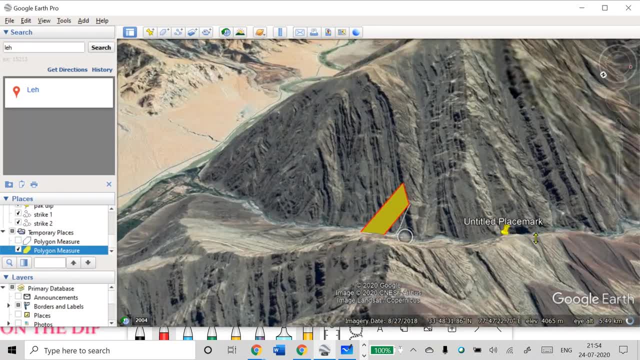 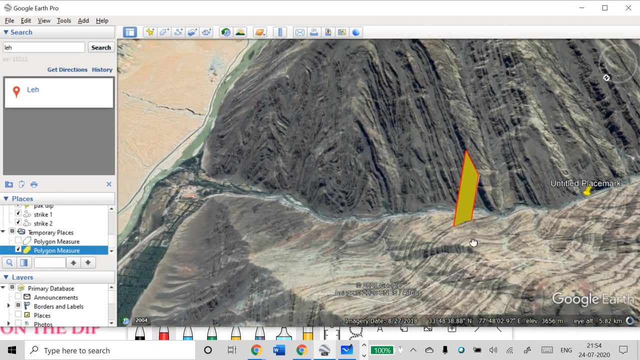 yeah, this is how the beds would have come out of the plane continued. now, this is how you visualize it, what you have given. so those strike lines, so these red lines that you will see from top, these are the two strike lines, and in 3d this plane looks something like this: it. 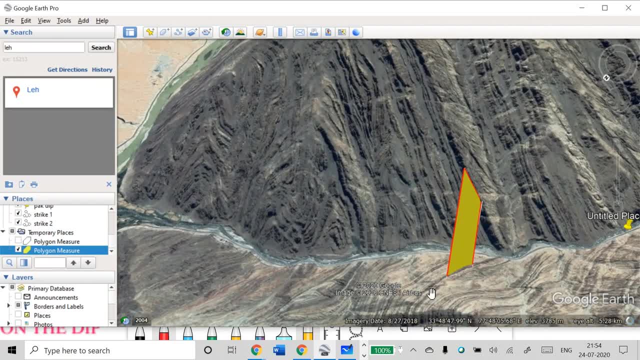 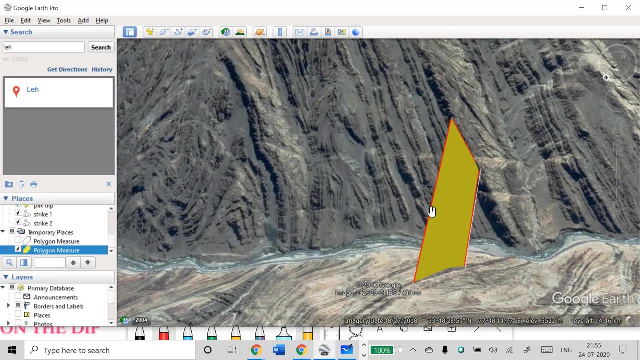 is dipping in that direction and you can actually continue it whole thing away. so, and on this one line, so this is a stratum contour. now you see this red line that you see on top. this is a stratum contour, or a strike line in this case, so they're both the same. and now you see 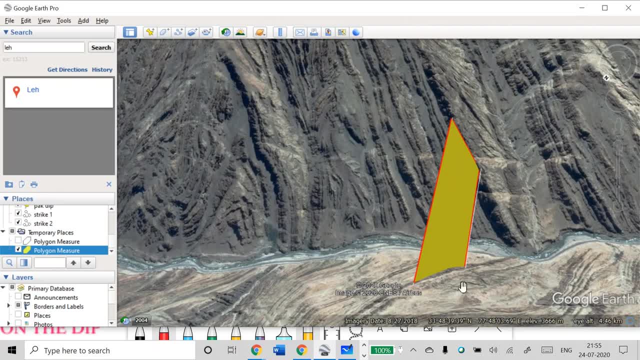 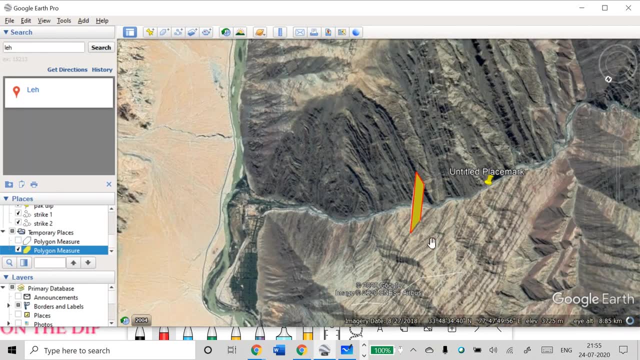 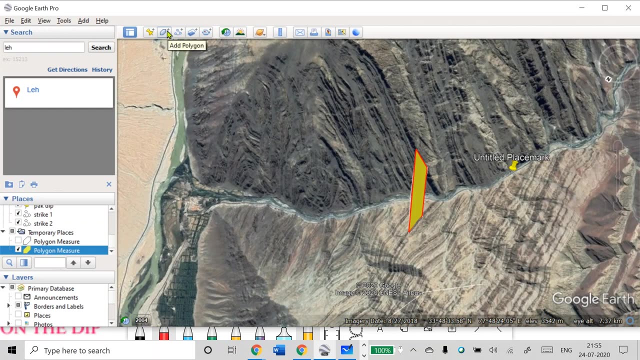 you're dipping, so you're going from one to another and if you draw these, uh, elevation contours, as we have already seen, so elevation contours will come, something like this, so you can actually practice it yourself also if you share these, so if you start drawing elevation contour from here, so it will go. 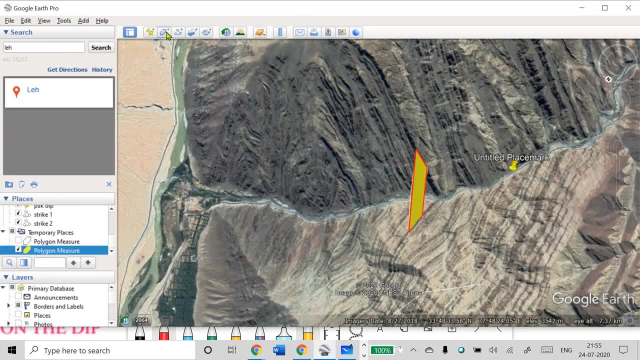 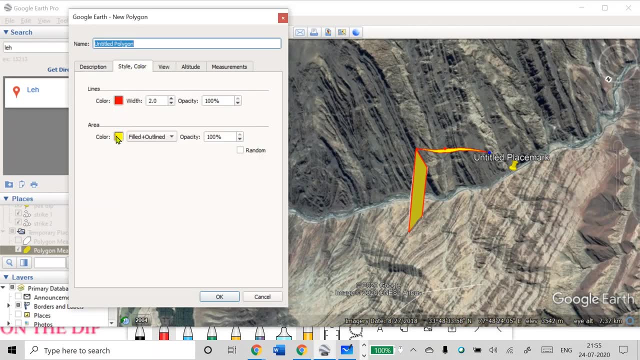 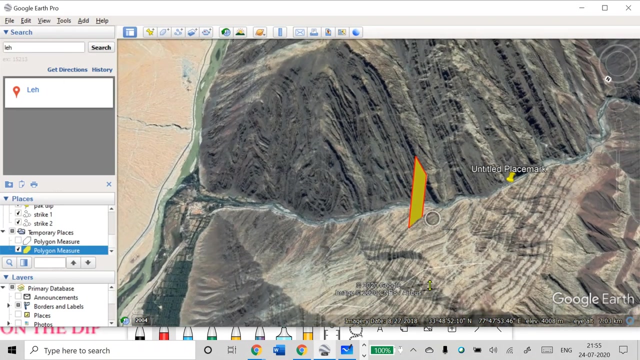 this is actually. this has added a path. cancel, yeah, and now it's just filling it up, so it will appear. these contours will appear, something like this: this is a contour, so it will. so now you get an overall idea, but just remember what is happening. so this plane. 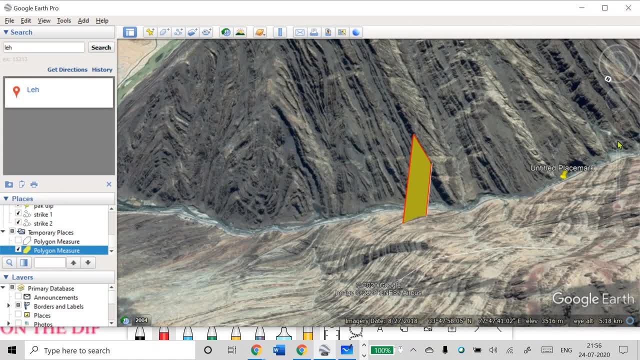 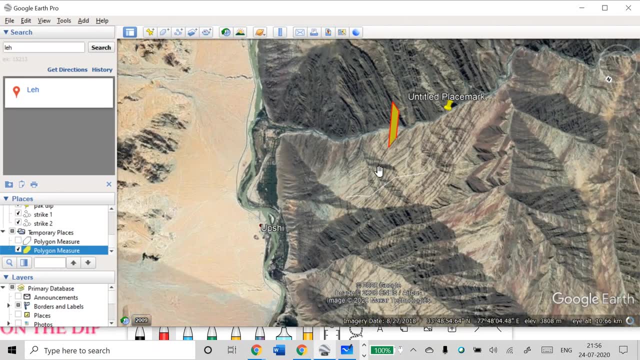 so this bed was continuous at one point of time. it's only. the only thing that has happened is a stream has come which has eroded these beds here and that is why you are getting this outcrop pattern. so it is very many times students find it very difficult or they find it very confusing when they see these different 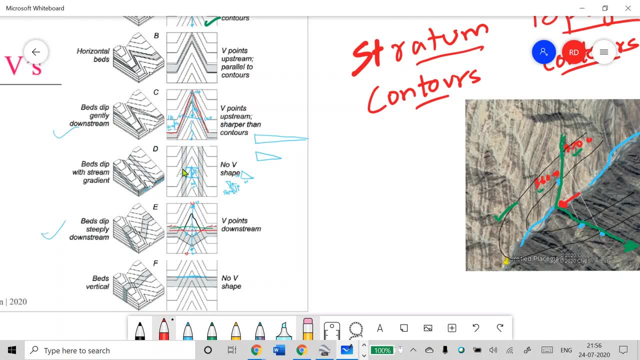 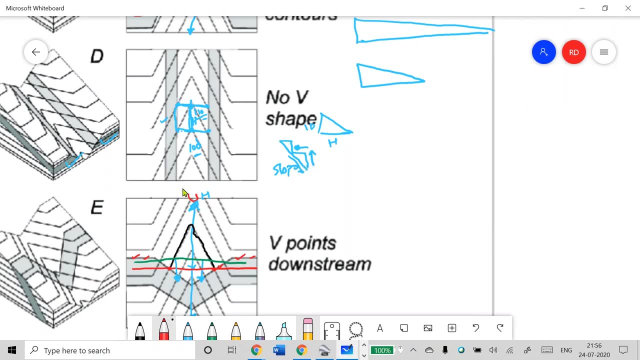 kinds of uh lines. what do they actually mean? for example, this, you have to remember, is outcrop pattern, these shaded areas. they are themselves not contours, stratum contours. so this line that you see here, this line for this one, uh for this bed, for example, this line that you see here, this. 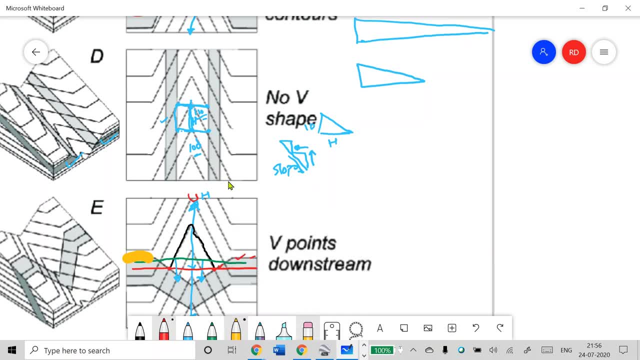 is not a contour. sometimes students get confused in this part also, so they will think: let me raise. they will think that this line is a contour, but contour, this is not a contour, this is just so. you'll call this as let's just call bedding trace. okay, so this is just the surface expression of that thing. 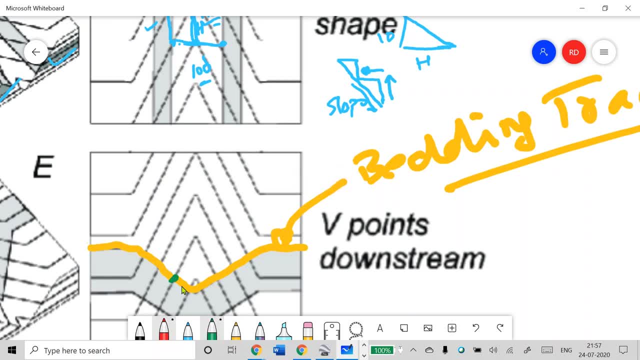 if you join points of equal elevation along this trace, and you can do this for fault also. for example, if you have a fault plane, you want to calculate dip of a fault so you can draw the contours for a fault plane also. the same thing because of principles are the same. so here: 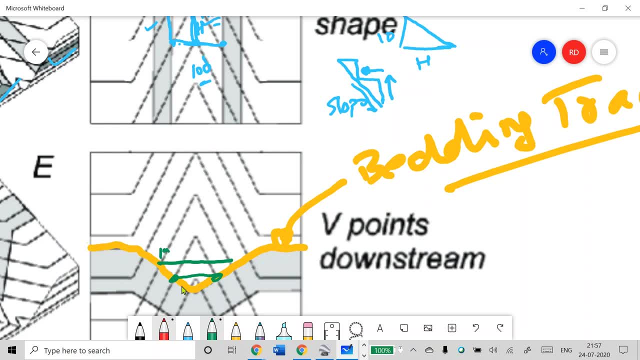 this is how you draw it. so this we has to be high, low and then here dipping. so these green lines are stratum contours, or bedding contours, anything you can call them, and these dotted lines are topographic contours. so these three things you have to remember. what are topographic contours? what are 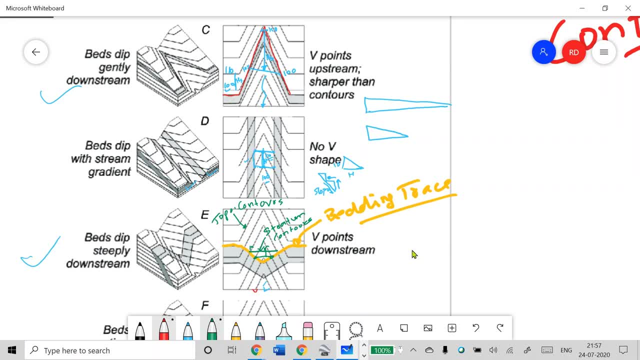 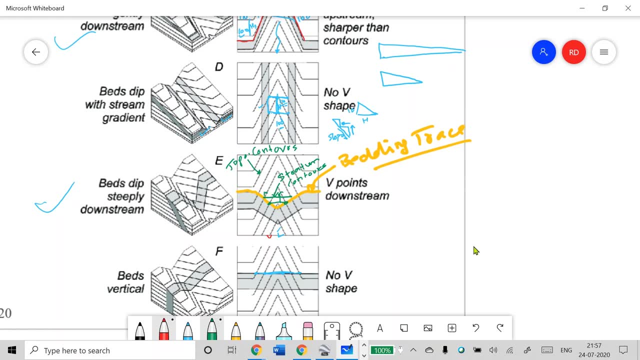 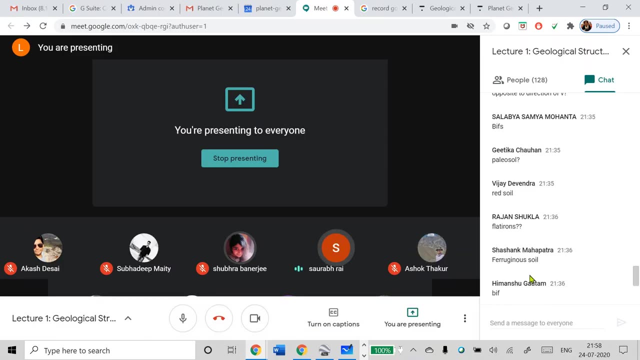 bedding contours and what? or stratum contours and what is bedding trace? so if beds are planar, your uh strike line will be the same as uh will be the same as stratum contours. now, once any, do you have any questions in this part? okay, someone was saying these were banded iron for others. 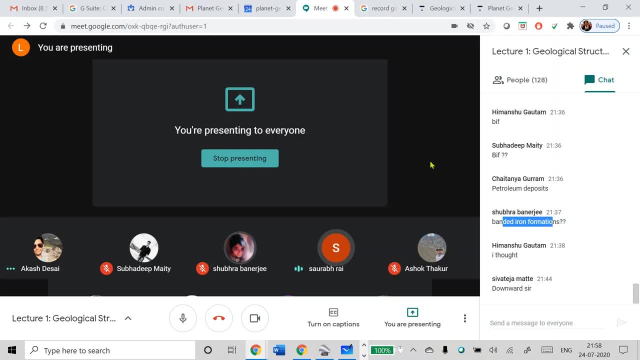 that the red beds that you are seeing. they are not actually banded ion formations. they are younger than banded ion formations. they are continental red beds, that usually called, and they are present within that close to that suture zone that you see there and many of them they have. they have. 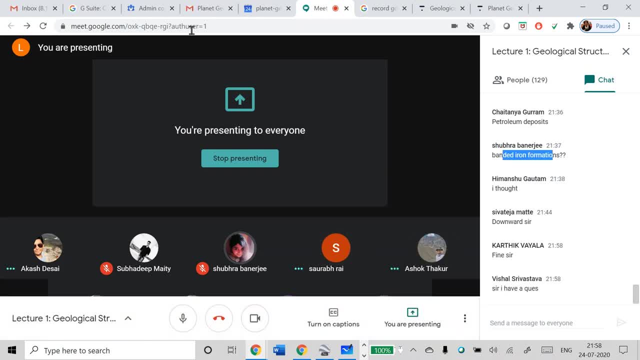 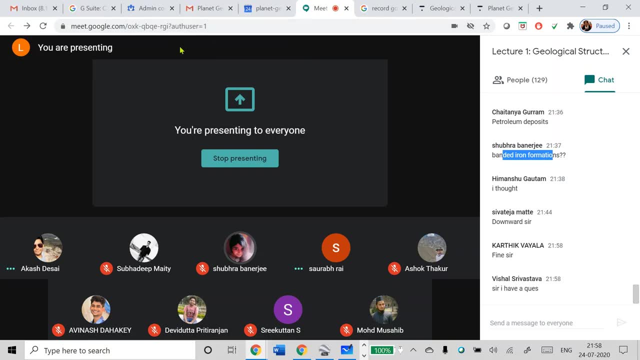 this red color because, yeah, ITCZ. so they, they are along this ITCZ where the closing of tethys C has happened. so actually, many of these beds, if you date them, you can also find out, if you know the age that, at what time this collision happened and when. when did this ocean closed? that is ocean. so 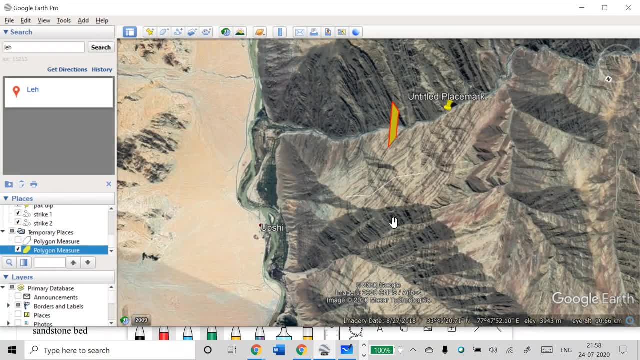 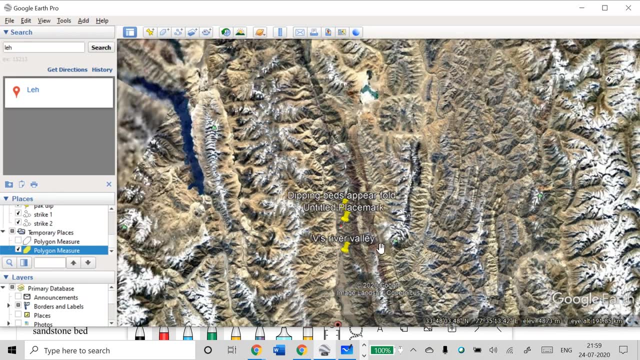 these, these are related to that. so here, if you go northward, so you've seen in different types. so we have seen the beds which were dipping in same direction as Valley. we were, we were, say, we have seen beds which were dipping in opposite direction as Valley and we have also seen examples of 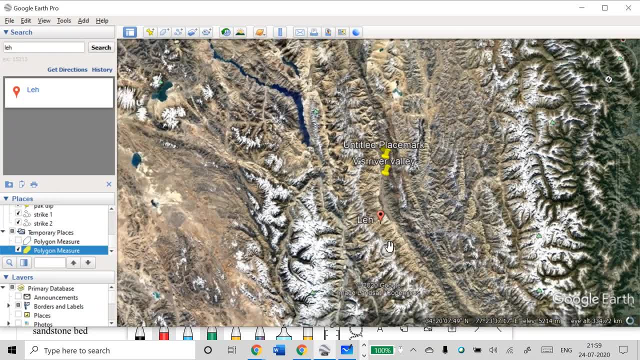 different types of tethys C. so we have seen the beds which were dipping in same direction as Valley vertical beds here. if you want to see examples of horizontal beds, if you have already seen recorded lectures then you will know. but okay, let me ask this: where, where do you think in? 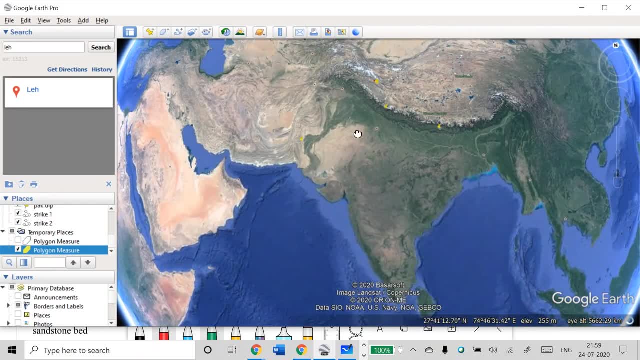 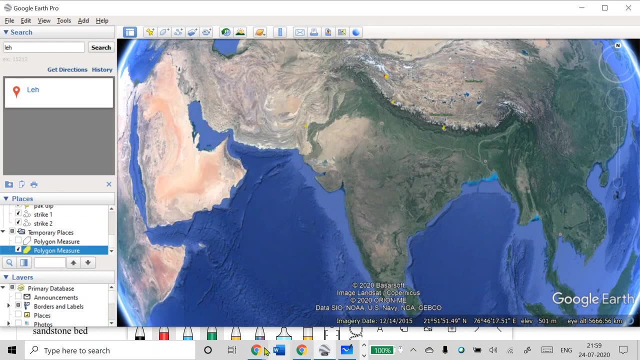 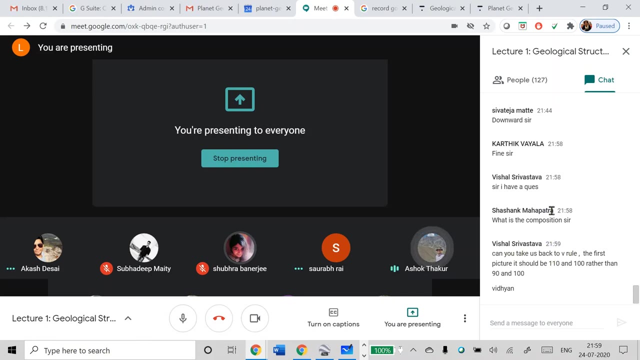 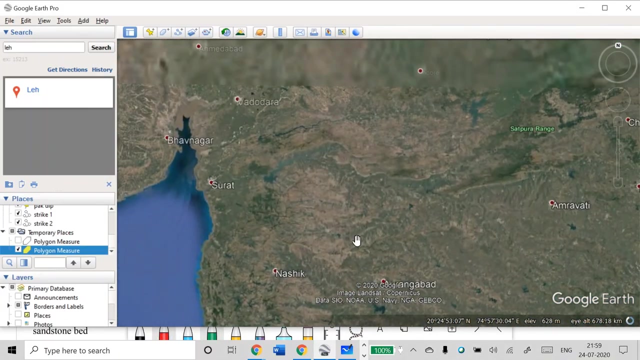 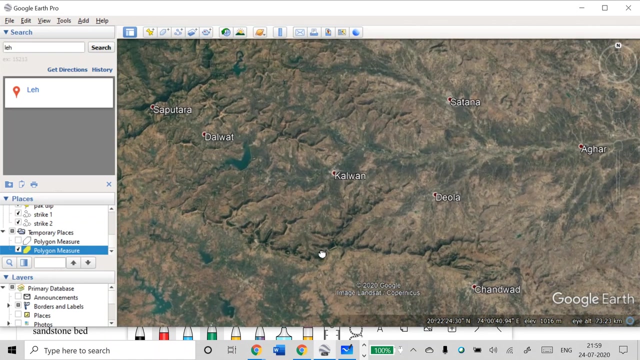 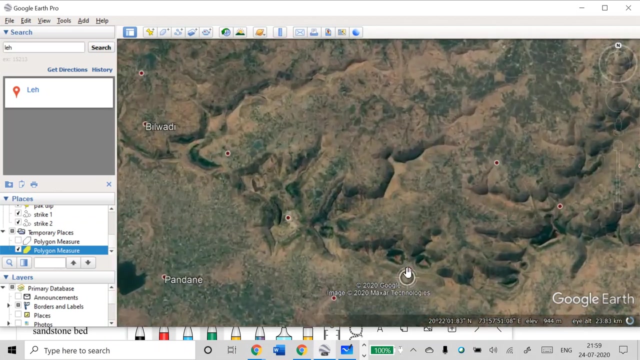 India, it will be easiest to see horizontal beds. any guesses? Deccan traps correct? so in Deccan traps? because these were low viscosity flood basalts, so they did not. they were flowing. so due to gravity they form horizontal layers and if you want to study any topographic expressions, you see here these examples. 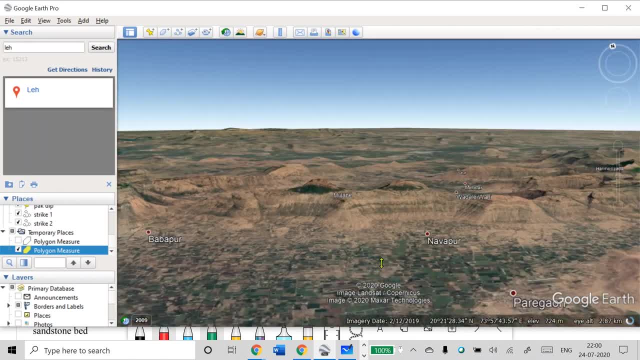 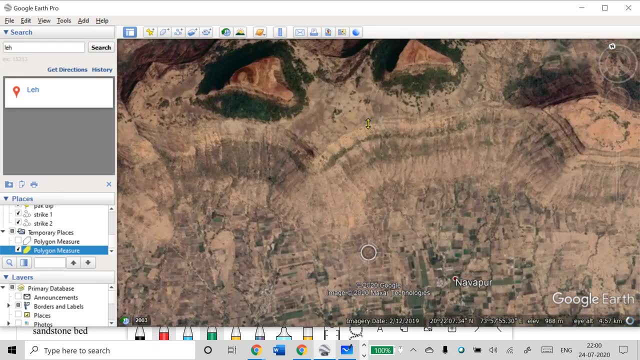 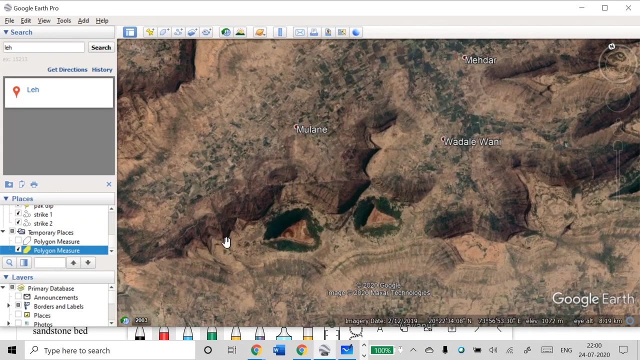 if you want to draw contour now, these are Deccan traps. and you see these layers. they are almost horizontal in this case, so they are not dipping in any direction. and if you want to draw, so now these, these will be parallel to topographic contours. so these should be parallel to. 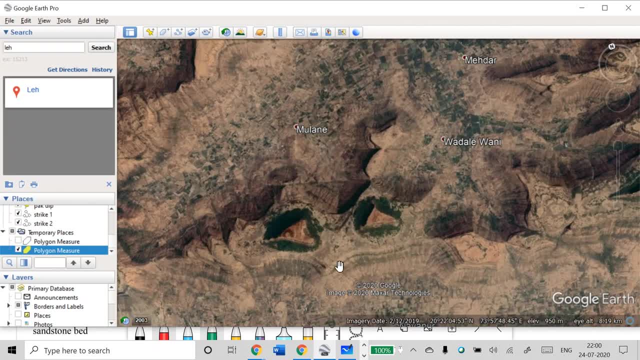 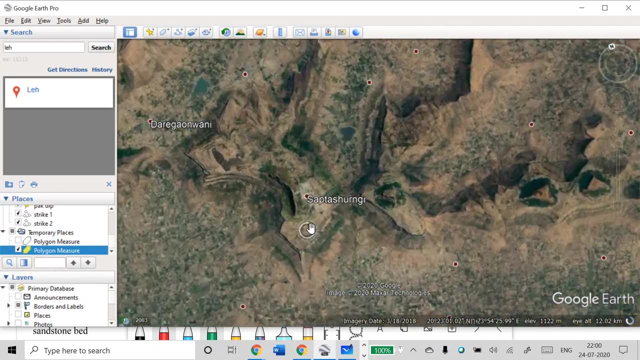 topographic contours, so these layers that you see, this layer. so this is the example in which you had those parallel. so if you take any valley close to this area, we will, let's say, if this is the valley, so you are here. if you have to draw topographicAntoode. 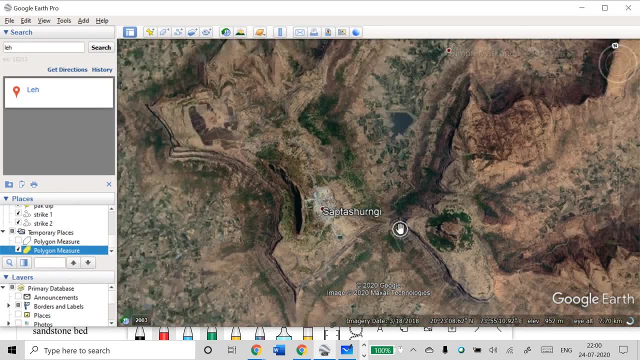 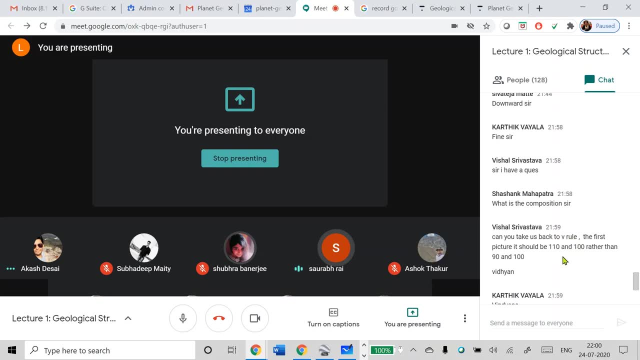 these will exactly follow these layers which you are seeing here. okay, so someone was commenting on first picture should be 110 hundred, rather 90 hundred. it doesn't matter see 110 hundred, ninety hundred you take these are. you are just assuming. no one has given you exact values. 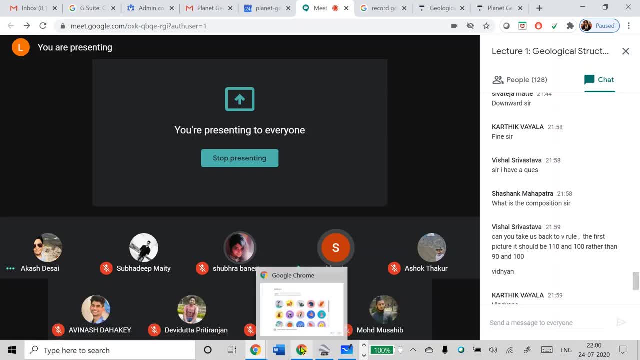 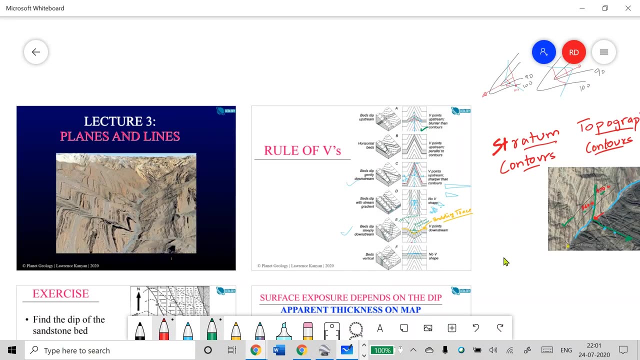 they are just for remembering. so you can take thousands of pictures and you can get to the thousand, fifty, ten lakh, whatever you want. only thing you need is which one is higher, which one is lower. you can also use just H and L. so for rule of these, you're asking: okay, so this, this picture, you are asking, yeah, so. 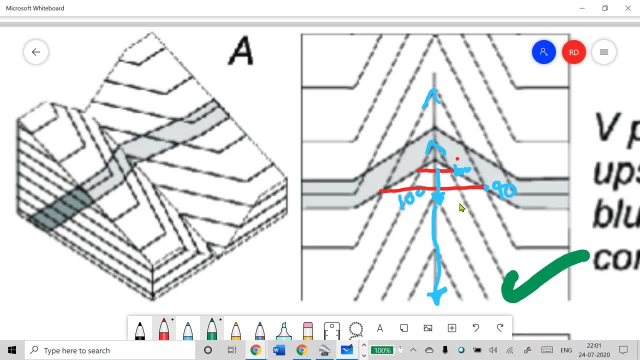 you're saying: so this has to be hundred and ninety, only because you see this one here that you see hundred. so this is this for the same one. yeah, so just a second, let me do it again. so let's say which were considering this, this part, and let's consider this part. 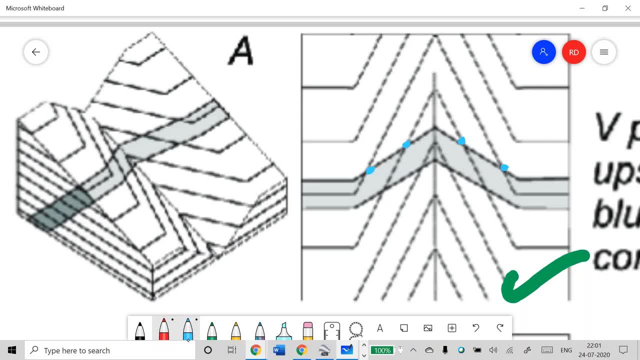 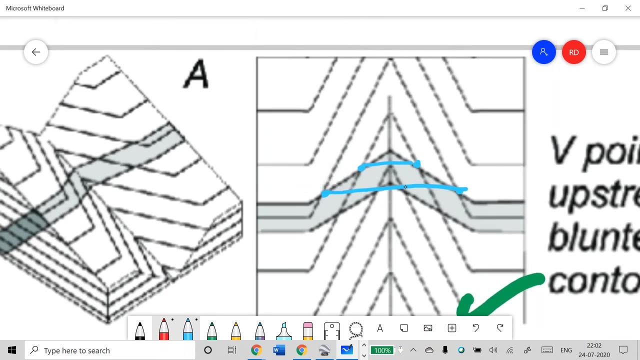 right here. okay, these two lines we draw. so these point upstream. okay, yeah, I think you're correct. and this is how will these are dipping upstream, correct? yeah, my bad, so this has to be so. this has to be lower, this has to be higher. so these are the two ones which we're. 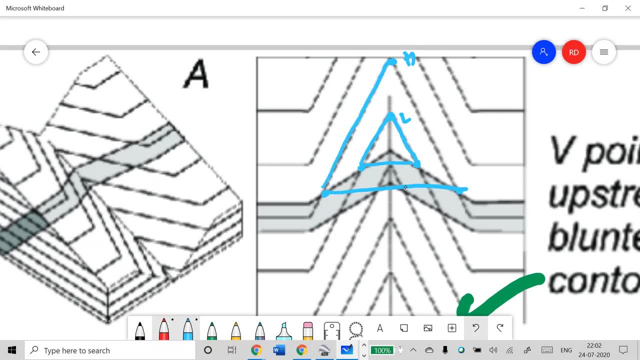 considering. so we points in high direction. ok, so you're correct. so this is higher, this is lower. so again, this is lower because you see this is continuing here. so well spotted. so this has to be higher and it has to dip, sorry, so now. yes, now you get the correct thing, so your stream. 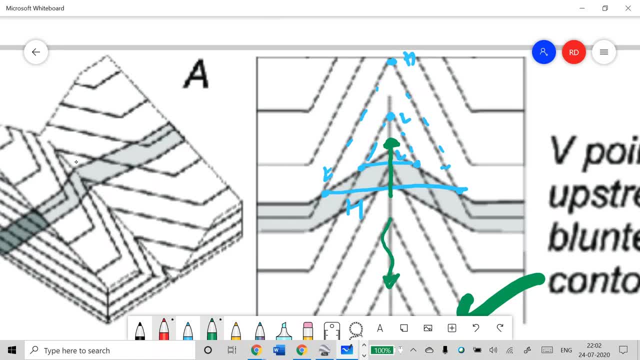 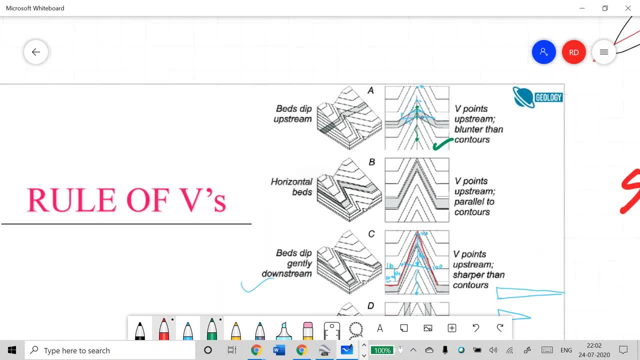 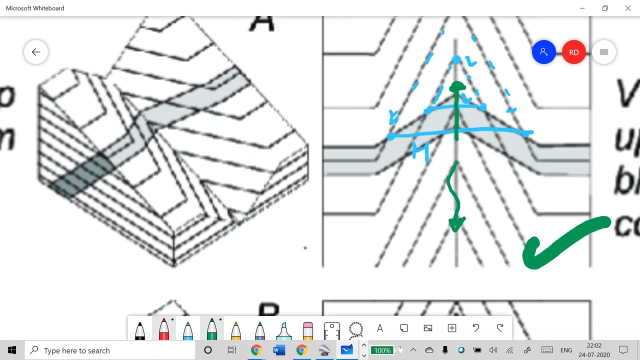 is flowing in this direction and beds are dipping upstream. so these beds are dipping upstream, like that. so thank you very much for pointing it out. so I had made a mistake. I drawn it like: so these beds, you know, you see they are dipping, stream is flowing in this direction and the birds are dipping upstream. 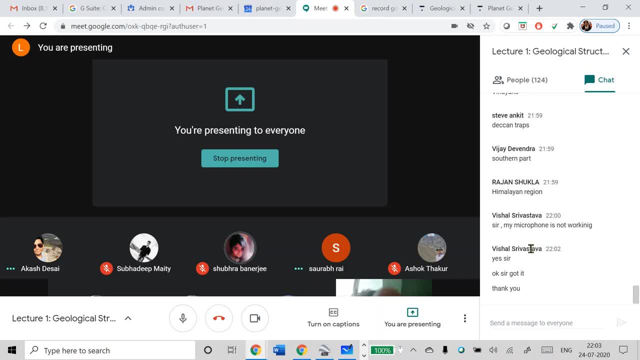 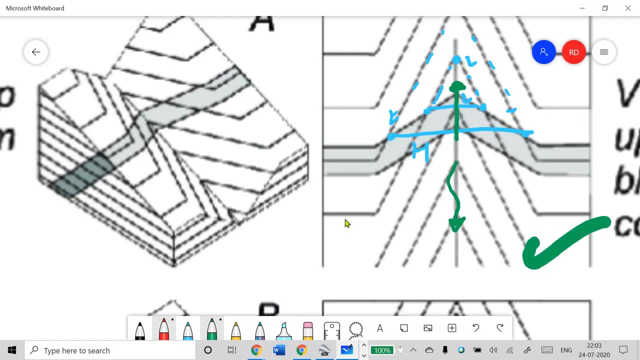 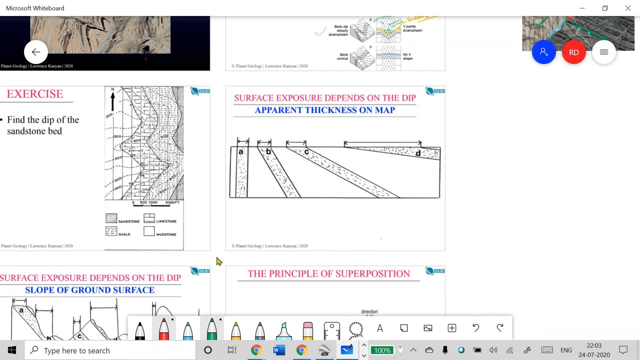 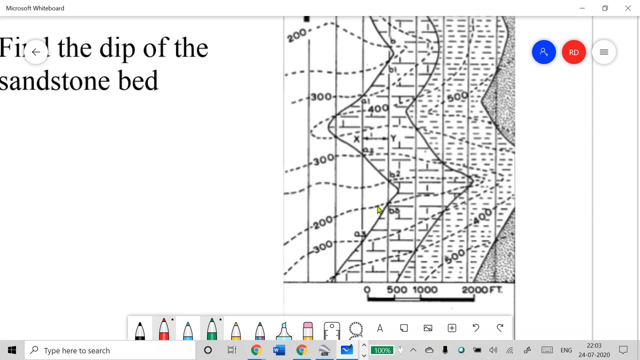 and okay. okay, thank you, Vishal, for pointing it out. now there are some more slides if you have to cover. so this, this thing, you should never forget, this is very important. so, similarly, there is a problem here. now, another thing is: after you can find stratum contours, you can be asked to find the dip of a given bed. so 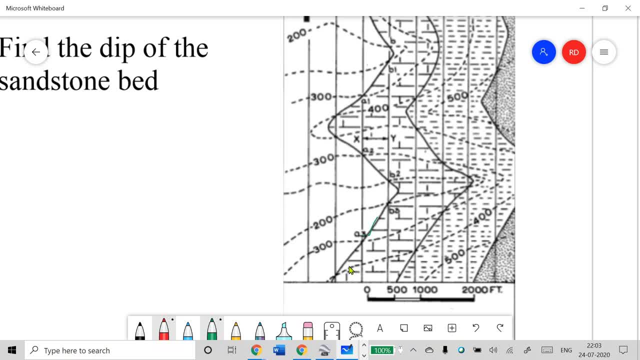 how will you find the dip of a given bed? let's say, for example, you can say, yes, you should consider this contact. so this contact you are considering. so for dip you always need two stratum contours, so the value difference between them will give you height, so each stratum contour will have its own. 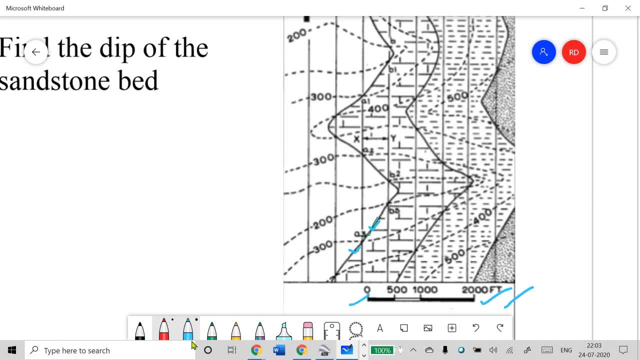 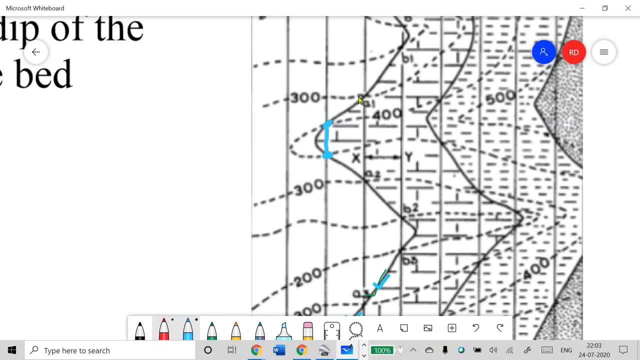 value and horizontal distance. you can measure from horizontal distance. you can measure from the scale which is given in a map. for example, let's consider this bed we were considering so this is of 400 meters stratum contour. they have give meters and this is for you see this. 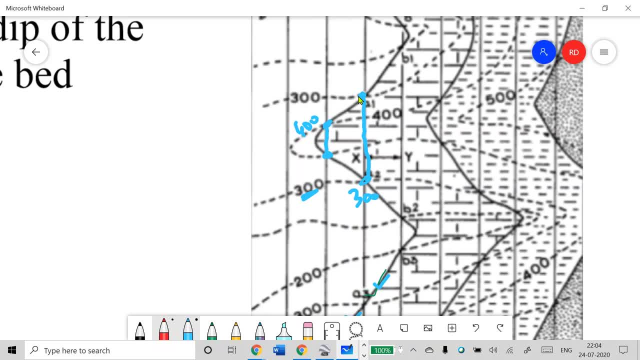 300, correct? so how will you calculate? so dip should be in this direction first of all. okay, so V is pointing this direction, so these are dipping in the same direction as stream is flowing, assuming this is a valley first. is this a valley? first of all, let me 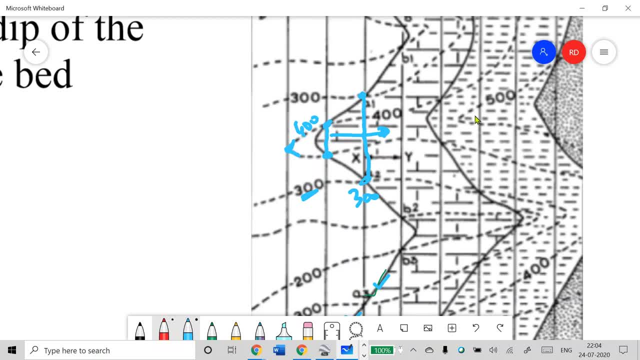 ask this should: is this a valley where I have drawn these lines? why do you say that this is a valley? let me erase everything and then try to answer again. is this a valley? so this? so again, let me tell you. so, first of all, these are topo contours. 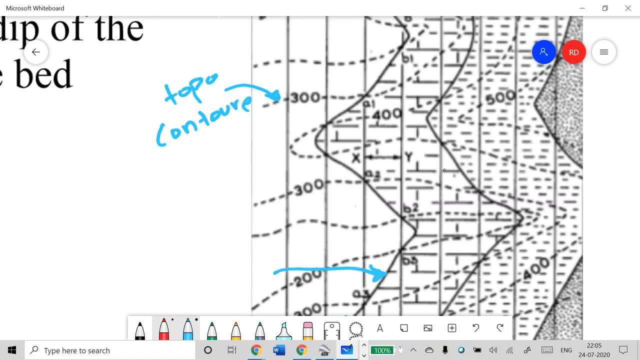 this right here is trace of bedding, okay, and these actually the ones that you see here, these ones, these are the dotted lines, so these are already drawn. these are stratum contours and you see, they are straight lines here, not like topographic contours because beds are all. 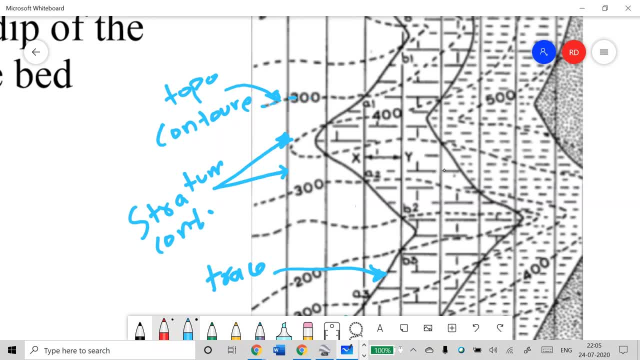 planar. if your stratum contour are not straight lines, then that means this area is folded. if your stratum contours appear something like this, it means folding has happened. so for planar beds, these stratum contours, they always have to be straight line. you see, these are all. 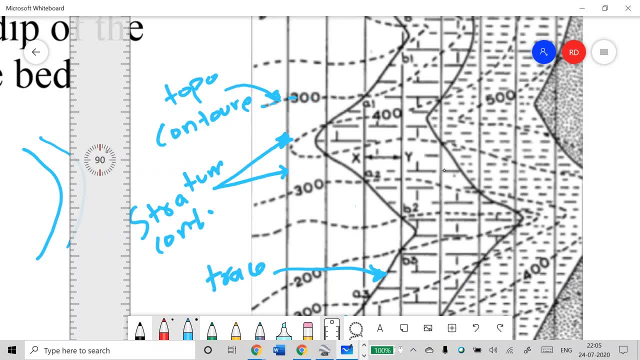 these are your stratum contours. so I was asking whether this is a, this is a valley or not. here is it a valley? so answer is no, it is not a valley because you see, this is 500 and this is 400, so V is pointing in downstream direction. so 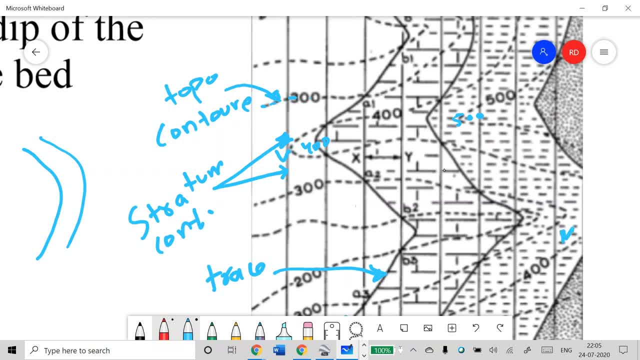 for valleys it has to be opposite. so valley is right here. so it is. this is a ridge. and again, this is a ridge, this is a valley. and then you will see another ridge down here. so this is a valley. here you see, the V is pointing upstream. 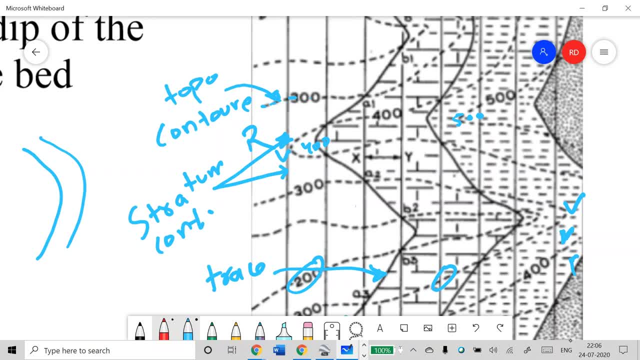 so, for example, this is 200, this is 300 and this is 400, so up V should always point upstream in case of a valley, but you can always tell where whether it is dipping in same direction. so the same rule of V that you saw. if someone wants to, 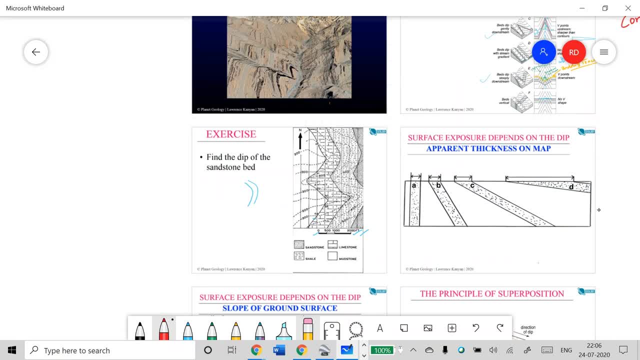 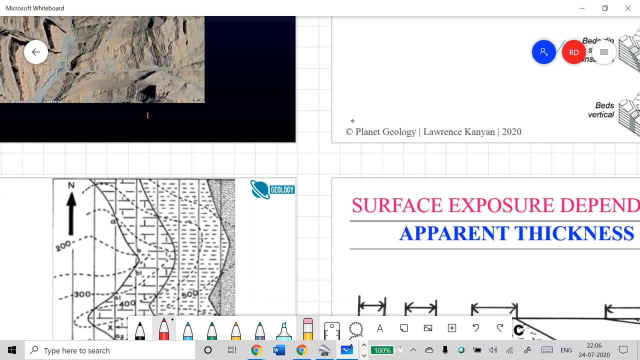 complicate this question what they will do. instead of V, they can give you just stratum contours. they can give you topographic contours and ask what is happening. so if you can read these values, you don't actually need to figure out whether it is a valley or a ridge. 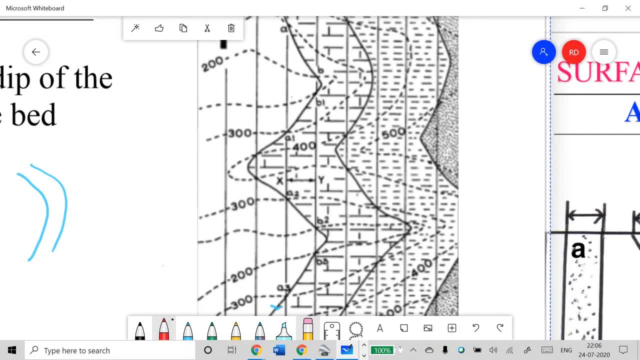 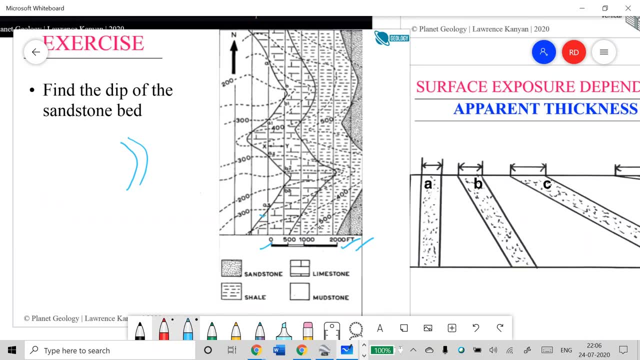 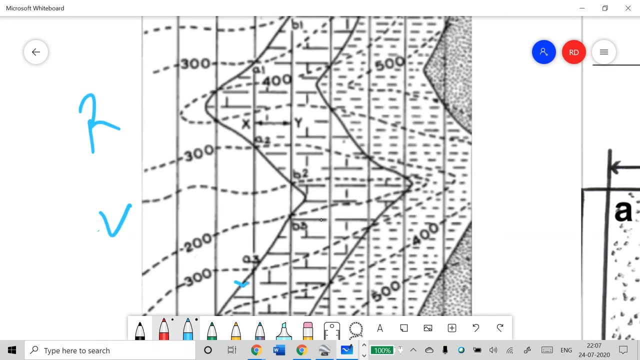 but just for your information, this is actually a ridge and this is a valley, right here, valley and ridge, let's do it for a valley only first, so because you are already familiar with that, or here let's do for ridge, so that that will give you more practice. so for 400 meter, you see. 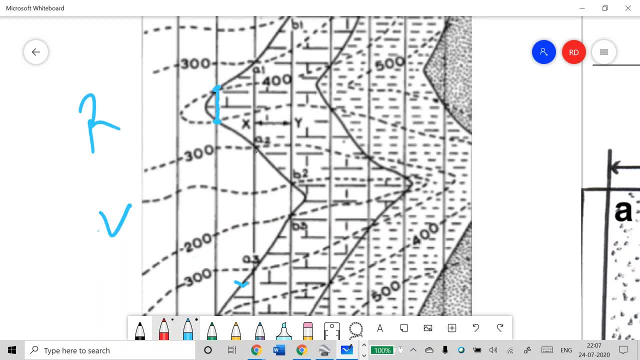 this is 400 meter, okay, and then you need to draw. for any other contour you can draw, it can be 300, 200, 500, whichever you can find this one. so this is 400, this is 300. so what is the dip? what is the dip? 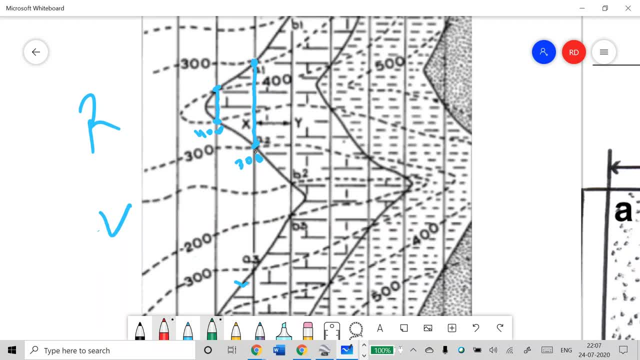 what is the dip direction in this case? east-west, north-south. what is the dip direction? yeah, so it is dipping eastwards. you see, now you don't need to remember rule of these, you can just directly use this or we use this method and you see the. if you 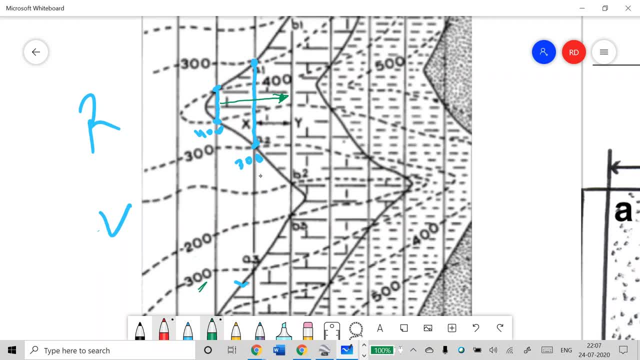 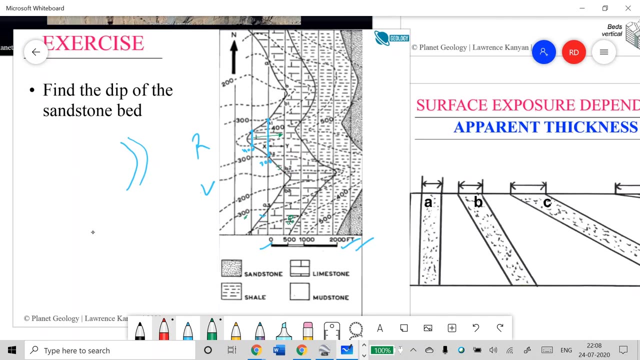 find another point. for example, this is 300 and this is 400 right here. so this contour, and you see, here it is again intersecting the same trace over here. so you, in this case, you actually get three points. so this proves that it is not folded. so this is not folded in this. 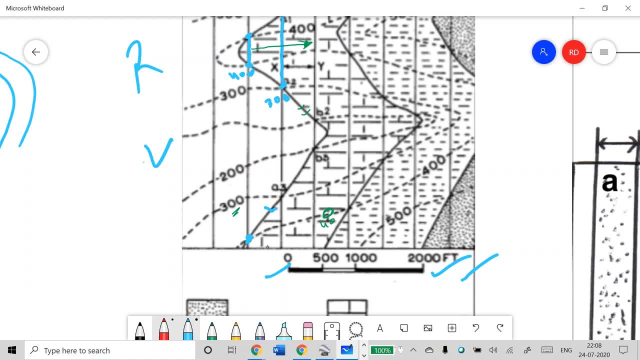 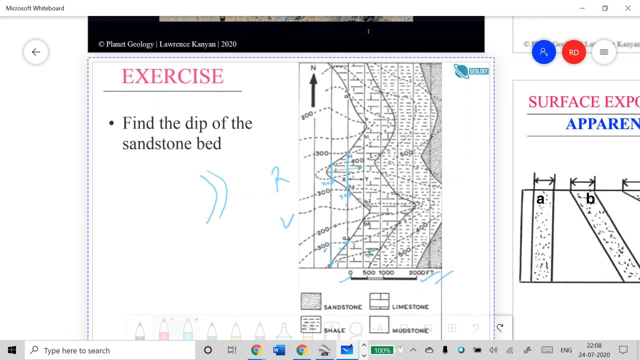 case. you see this blue line. you can continue it up to here. similarly, this for 300. it is intersecting again here, so you can continue. so you get the whole stratum contour. now the question is: how can you calculate the dip amount? so how will you calculate the dip amount? so for 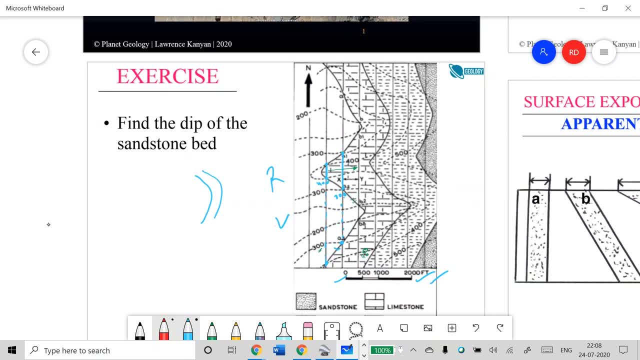 that you need. you need to know the vertical distance and then then you can apply simple trigonometry: you need to know the vertical distance and you need to know the horizontal distance. so what is the vertical, what is the vertical distance? in this case, hundred meter, because you have two. 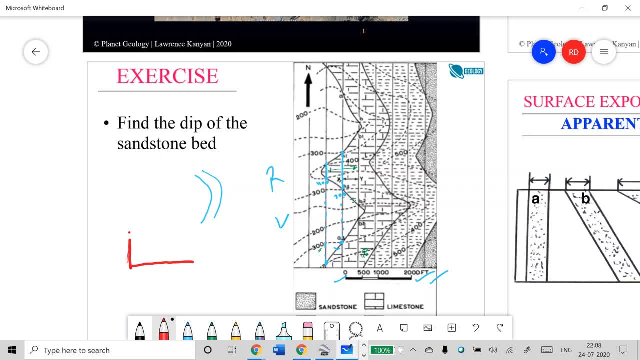 contours: 400 and 300 meters. two contours you have already got. so this is the hundred meters, because this was 300 meter contour and on top you have 400 meter contours, so difference between we should be hundred. what is the horizontal distance? how will you find horizontal? 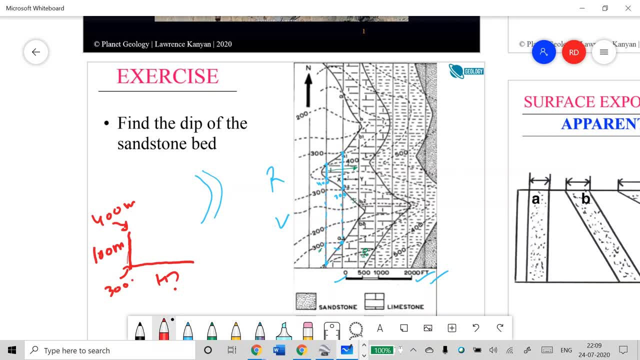 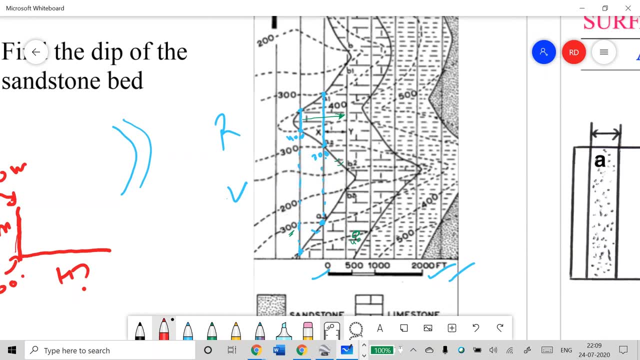 distance. yes, correct, so with the given scale. yes, so yeah, here you see, approximately will be 500. so normally what you will do is you will put your scale here and see what is the distance and then you use the scale for the that. that distance, let's say this is approximately in this: 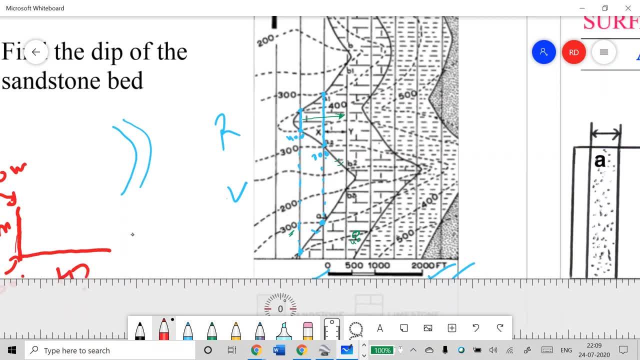 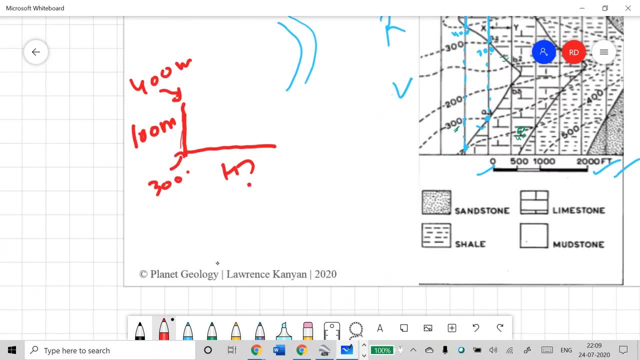 case. you see, these are two units and 500 meters is all to unit, so actually it is given in feet. in this case, these are all values and feet. so let's so, if you go back here, so this should actually be all these value should be feet. and you saw, 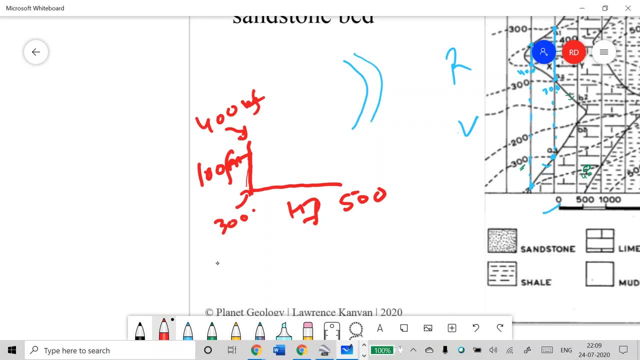 this is 500 feet. okay, so we make it more clear. everything is in feet. so what should be the slope? this was 100 meter and if you assume this as a not hundred meter, feet in this case, so if you assume this is theta, how will you calculate slope? so slope, if you. 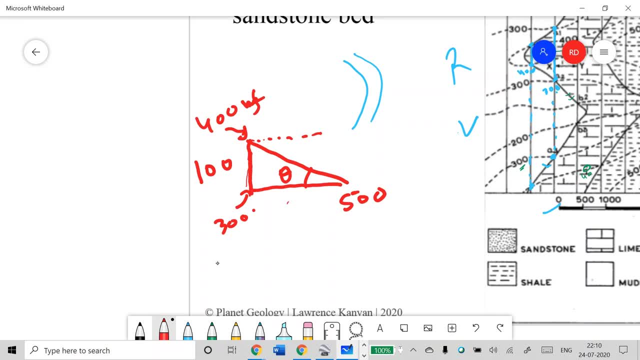 know, or the dip, dip of a bed. you measure it with respect to horizontal, so this is your dip. so alternate angles, parallel lines, so this is also. theta is also dip in this case. so you use the formula tan. theta equals 100 over 500, so theta will be. 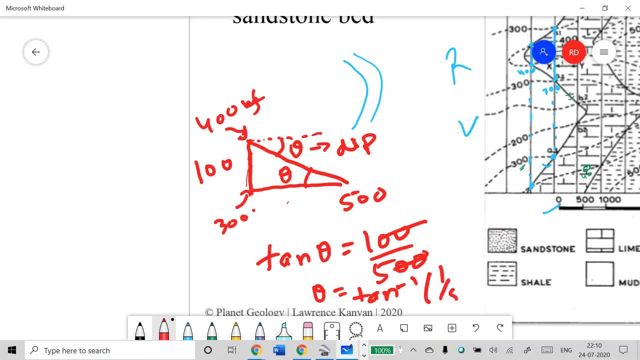 equal to tan inverse 1 over 5, so someone can ask you question. in this case they can ask you what is the value of theta, or you can, you can be given a simpler question, for example, if this is also 100 meters, then you will not even use a. 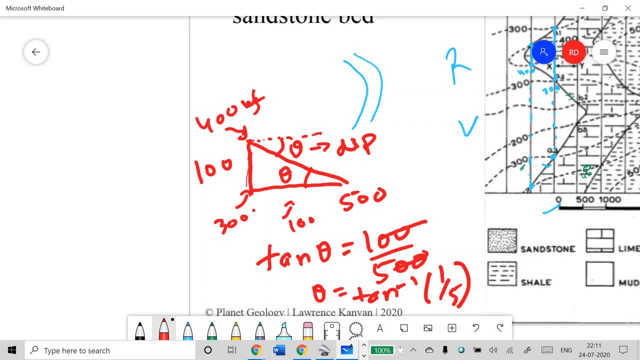 calculator. you will not need to use a calculator. in that case, it will come out to be 45 degrees, so, and you can apply this principle to determine dip of anything. you can determine dip of fault. you can also determine dip of Valley floor. so if you want to determine what, 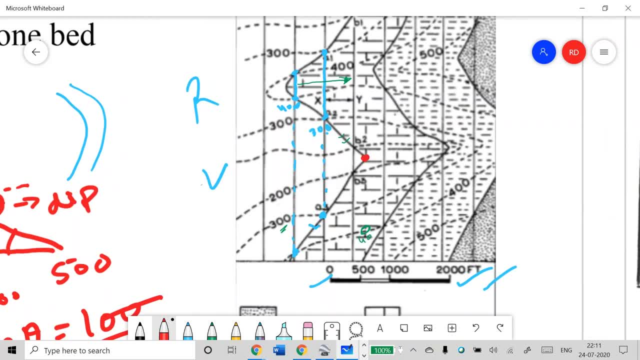 is the Valley slope. so you, what you need is, you need to know, for example, what is the elevation value here. so it will be around 150. you see it is less than 200. so you don't know exact value here and you need value here. so it will be closer to 200. so this, for example, will come out. 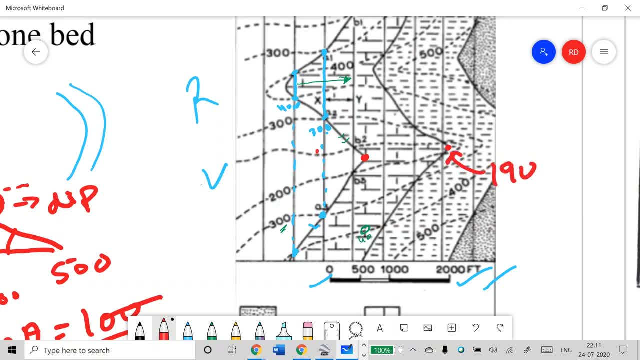 to be somewhere. let's say 190 is 200 meter. contour is very close by and the red one here it will come out to be how much so it will be around. let's say 150. so you know, vertical distance is 40 meters, horizontal distance again you get. 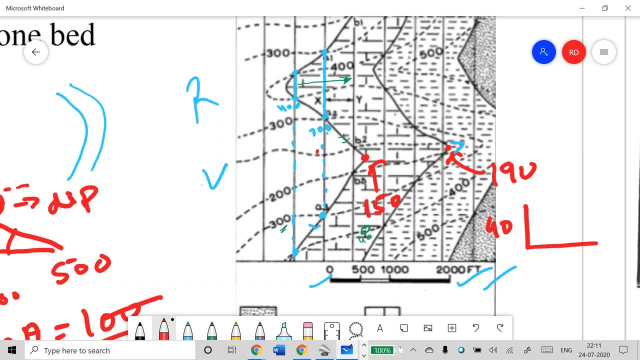 from scale, not meters, feet. so in this case let's say it's 2000. so for now, in this case will be tan inverse 4 by 200. okay, so this is how you will calculate. so you see, this will be much less compared to the slope that we found out. 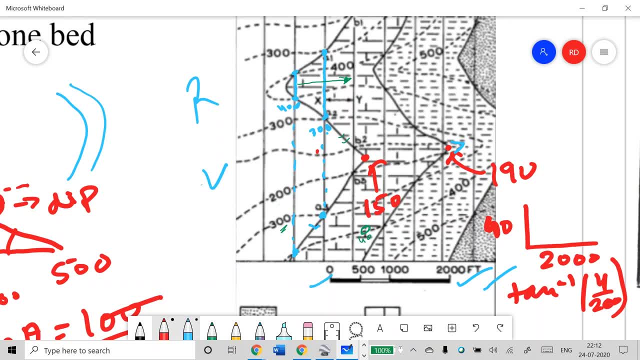 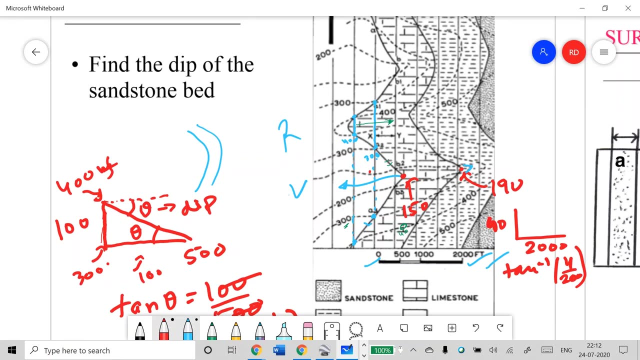 so in which direction the slope slope is? in this direction, opposite of V is pointing, and it is much less compared to the slope or dip of the beds, because horizontal distance is much larger for same, but actually your vertical is even shorter, but if you increase it this will also increase. 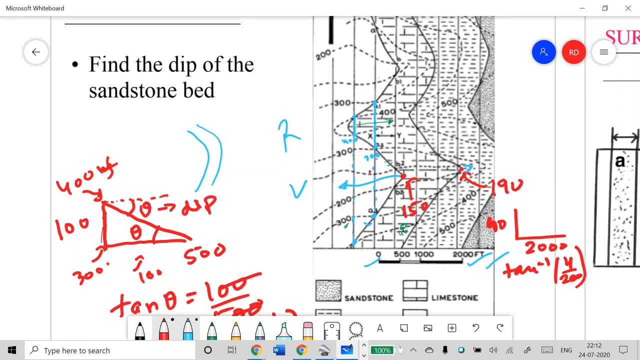 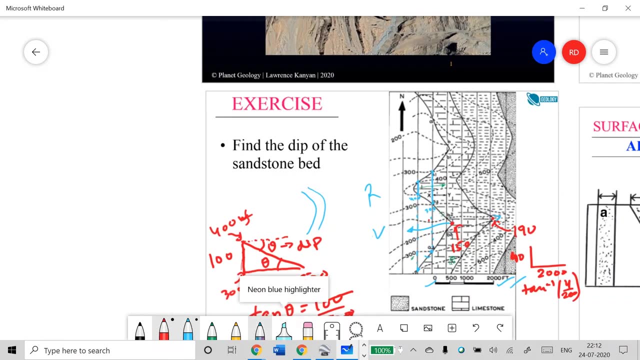 so it has less slope. so whenever you see more horizontal distance for same vertical distance always means that the dip in the bed is less. everyone understands up to this point. so all these are stratum contours and you can use those stratum contours to determine the dip. 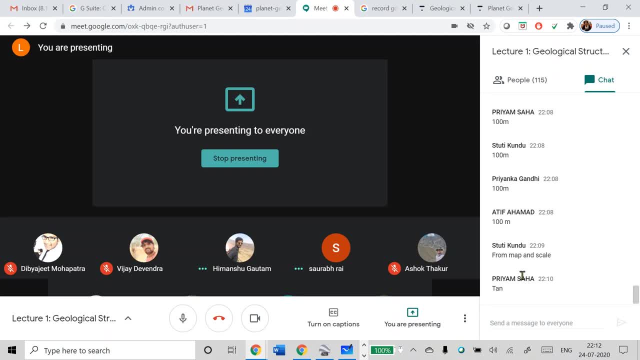 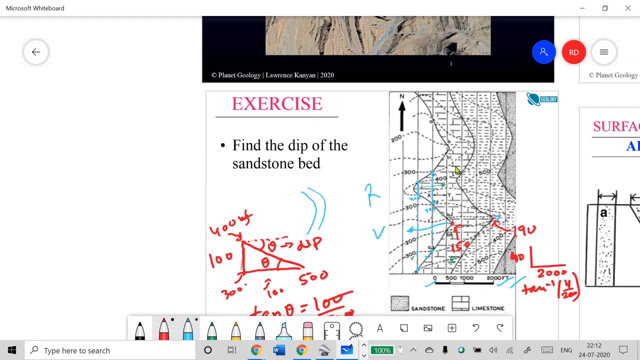 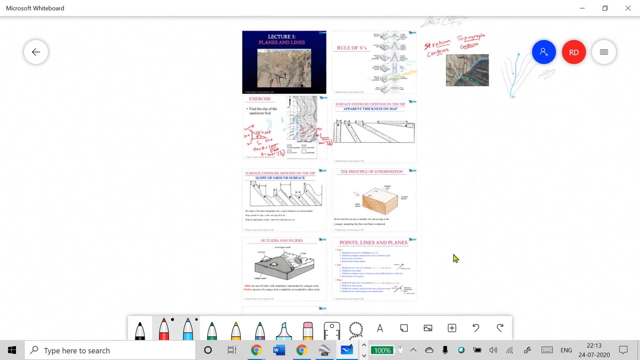 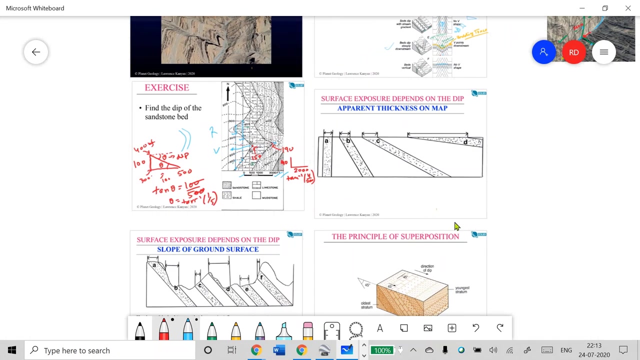 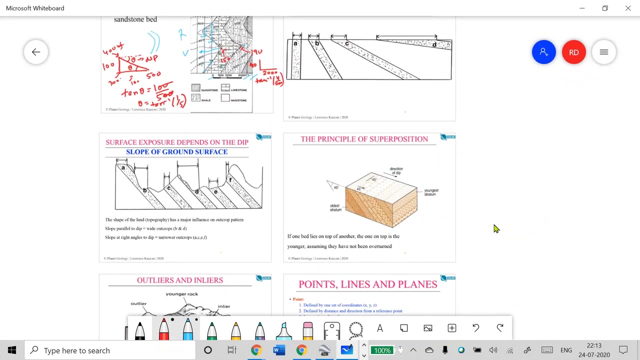 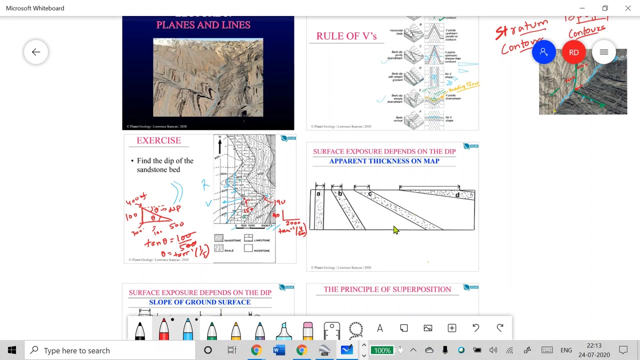 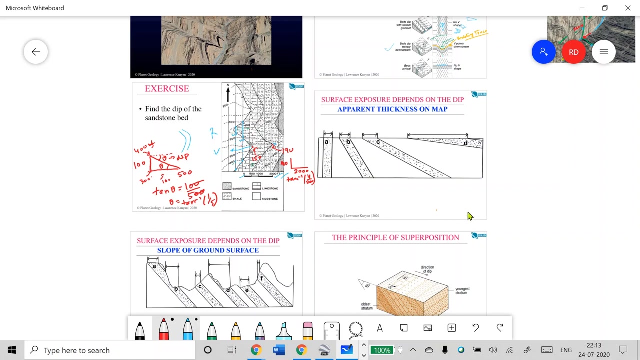 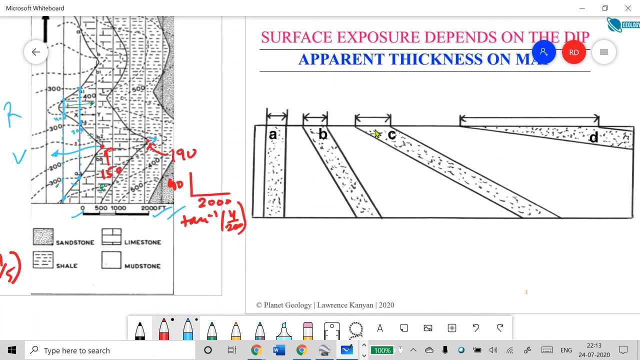 so glad that many of you actually give correct answers of the. I will also upload this recorded lecture so that you can view it. you And so, and, or I will upload recorded lectures for these so that you can view in your own time. But main thing that I wanted to discuss I have already discussed: In these cases also, you just have to apply trigonometric principles, For example, this is the apparent thickness of the bed Here. you see, This is the apparent thickness. 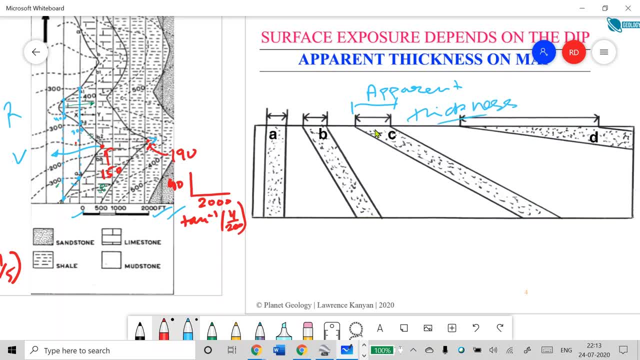 This is the apparent thickness of the bed that you see in outcrop. So for vertical beds, apparent thickness is same as stratigraphic or true thickness. This is the stratigraphic thickness or true thickness. As your beds keep getting gentler and gentler, your apparent thickness keeps on increasing, and for horizontal beds it will be almost infinite. 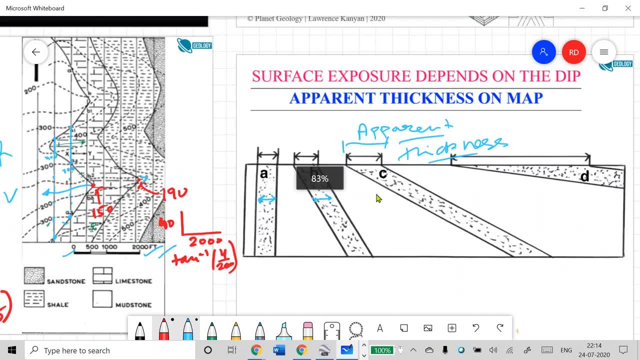 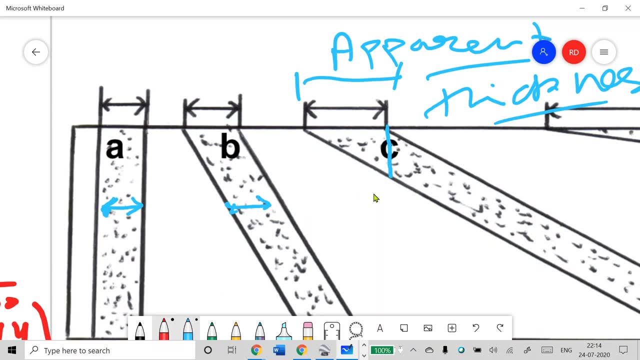 You see it is increasing as they are getting gentler. So what you can get is- you can actually get a question based on this- That what should be a bed is dipping like this. It has thickness of this, So you need to calculate what is its true thickness. So this I will leave as a homework exercise for you guys. You try to solve it yourself and then tomorrow, tomorrow- I will upload a recorded lecture for this part also. 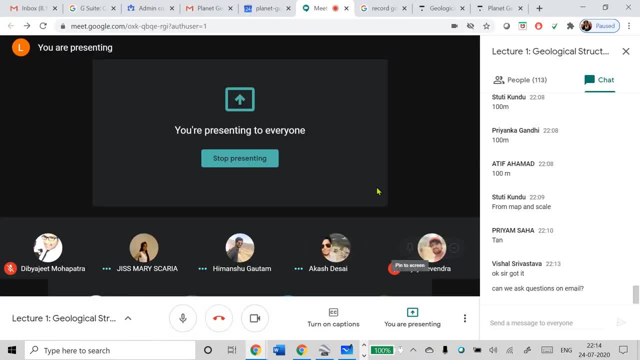 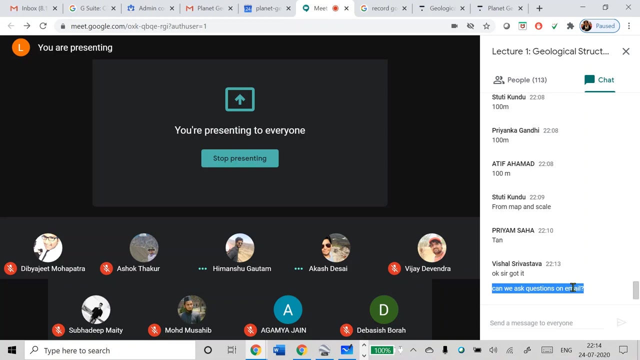 So after taking if you have any questions, after taking those questions we will stop. and can we ask questions on email? No, I will say instead of email: You ask if you go to course website, there you have discussion forum So you can put a discussion out there so that everyone, so it will, it will benefit everyone if you are asking a question and then then I can also respond, or if someone else responds, then I might not even have to respond. So if you are, if you have to ask any questions, just put them on the discussion forum on the course website. Do not email me. 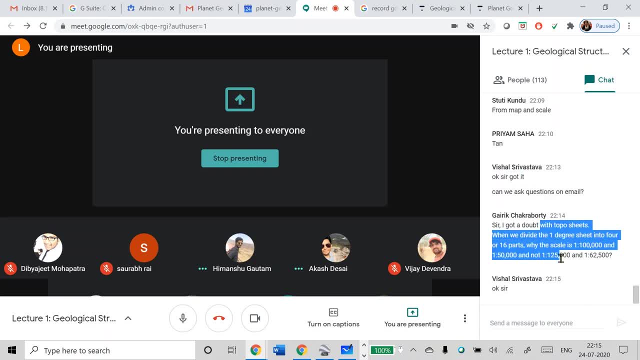 Okay, So for toposheets greek, I would first say: you, I have already covered this, I've already covered this in the recorded lecture, So once you see those, you will all, you will automatically understand this part. Okay, Okay, Okay. 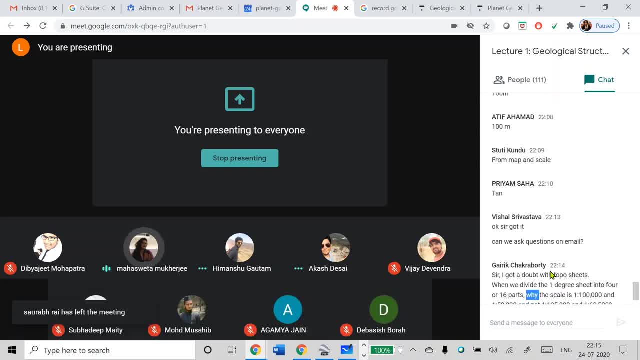